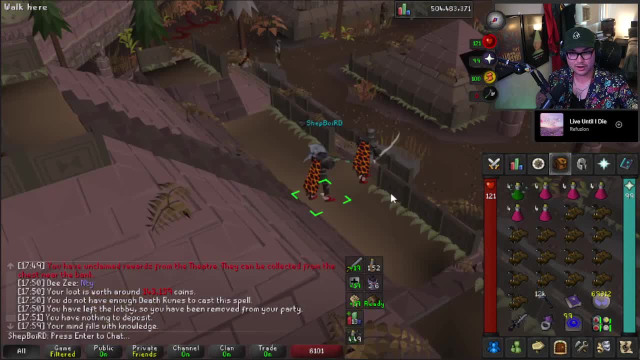 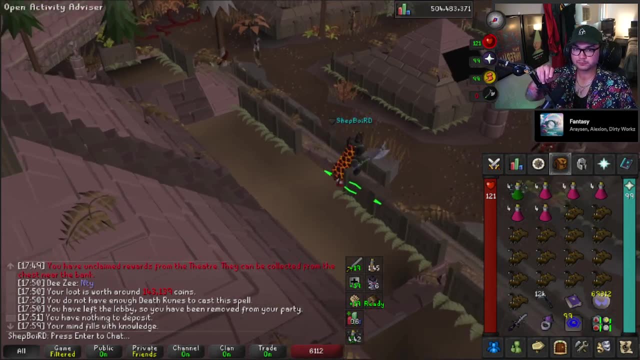 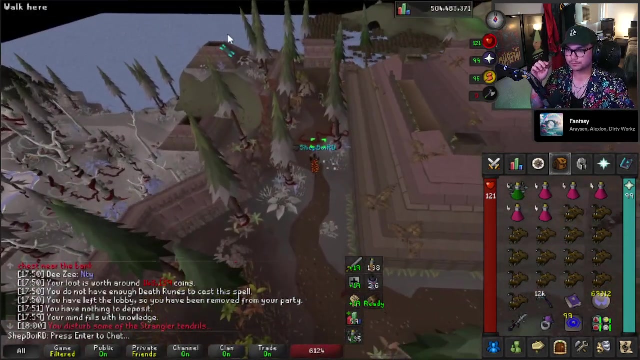 Some Vardossi is what I'm feeling today. I got like a bar of chocolate sitting next to me. it's like a whole thing. So like I feel like chocolate that is hard is better than chocolate that is like warm. 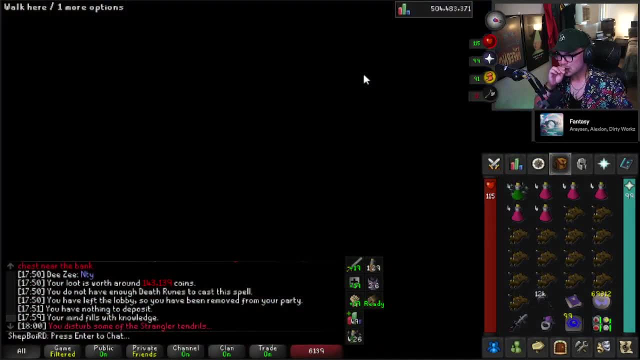 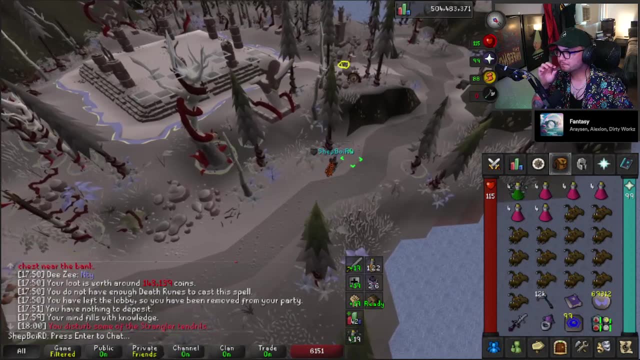 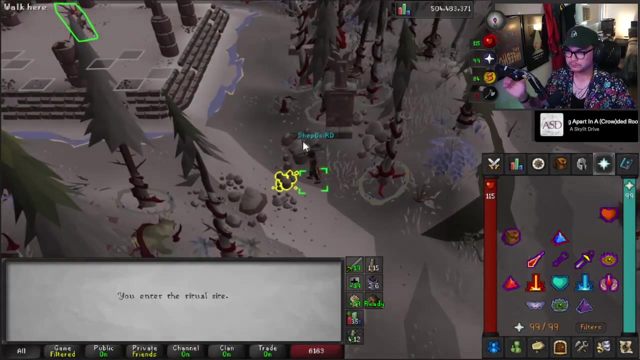 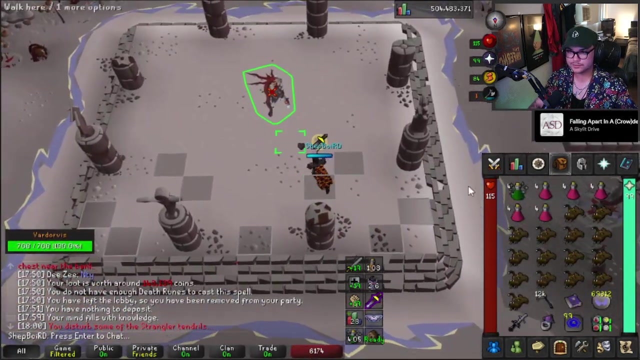 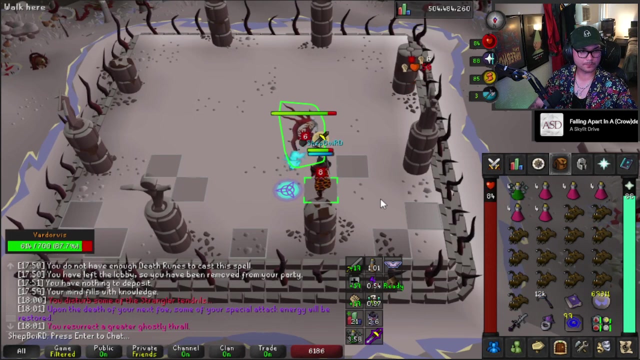 and soft. I don't know if that's weird. I don't think I'm feeling that. Okay, Okay, Okay, Okay, Okay, No, yeah, Doing some Vardossi. Turn Varoobite down a little bit too. 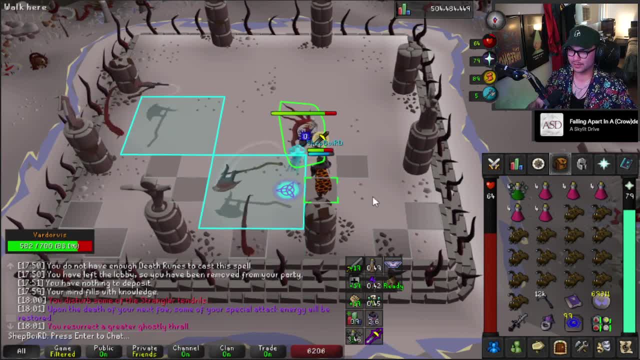 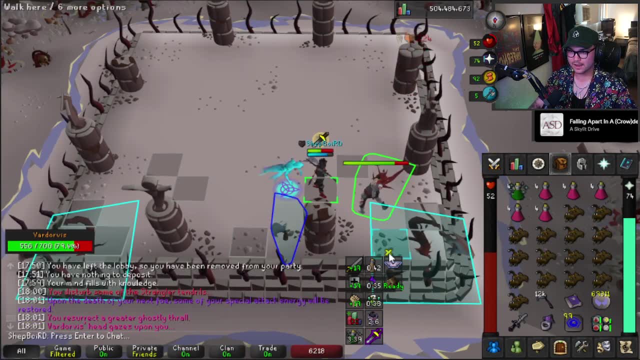 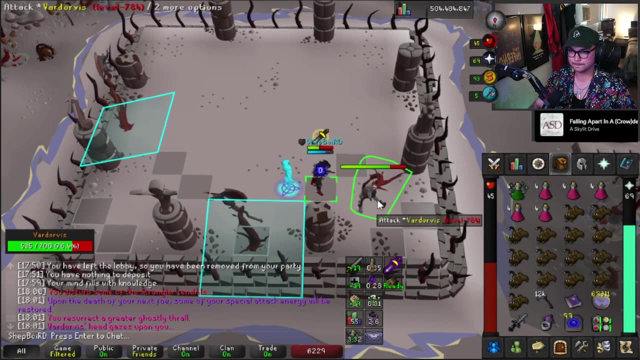 I didn't realize runescape was so fucking loud through OBS, Did not even realize. Dude, this ax sucks. this ax does not hit any numbers, I swear to God, god. And I really wish it did because, like I don't know, there's some times where it 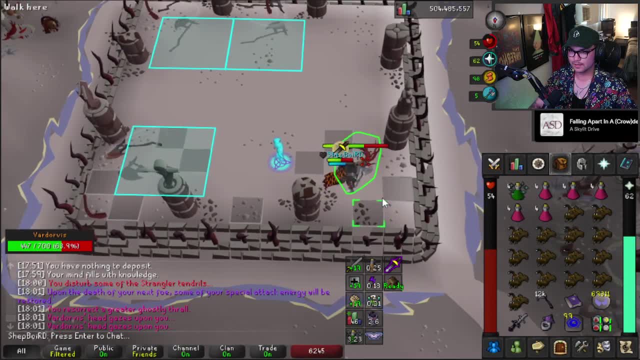 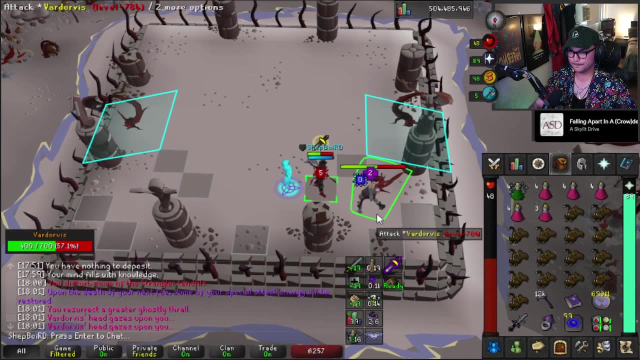 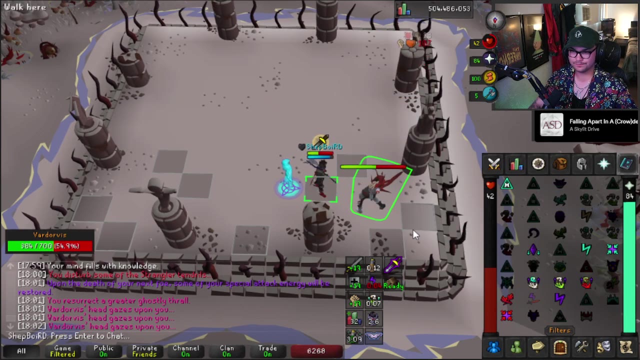 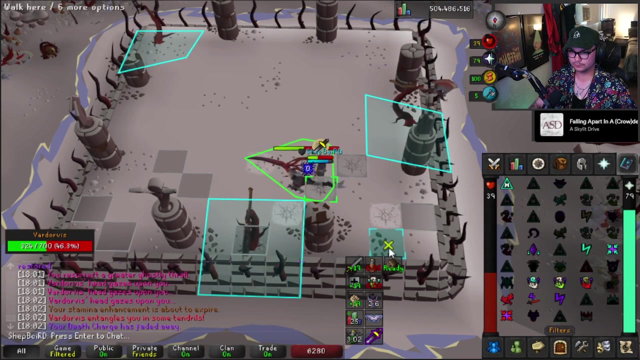 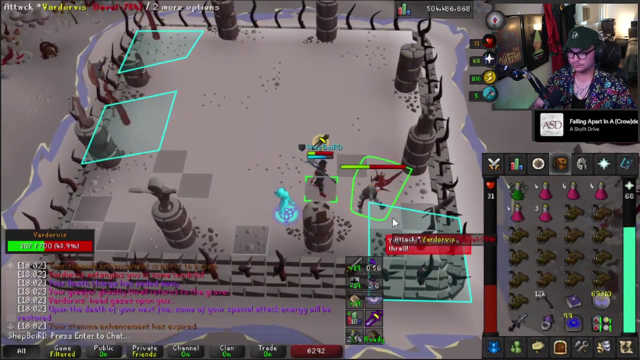 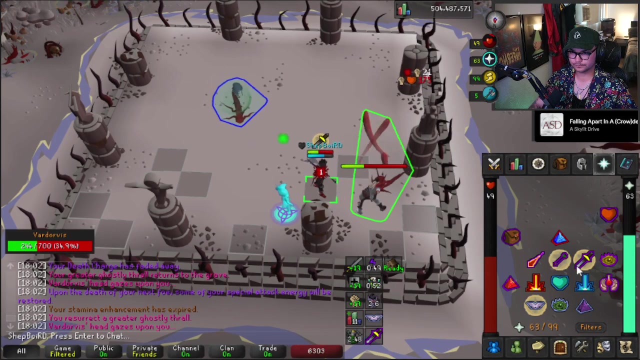 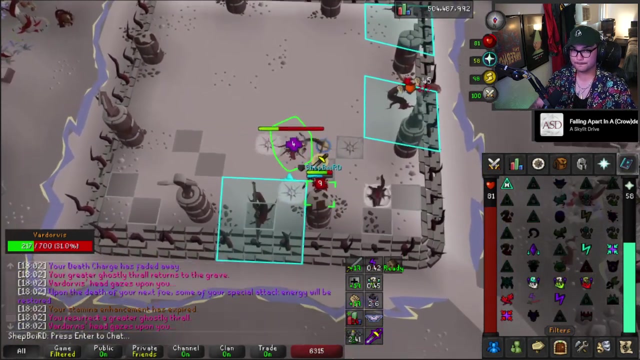 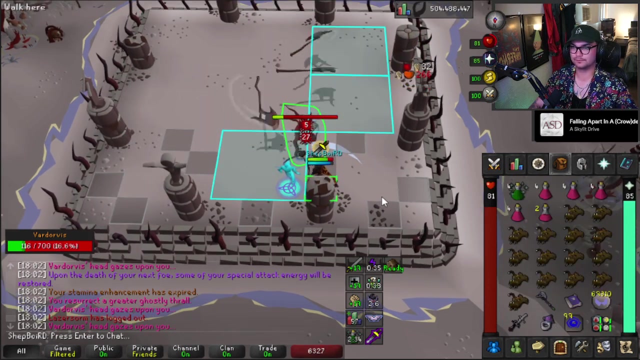 just smacks and then most of the time it just doesn't. That makes me sad. Makes me sad. Axe, no, hitty Axe. can you hitty Axe, please hitty, There we go, Axe is hitty. We put on scythe, We click moss, We do thing. Dude, I swear, I think. 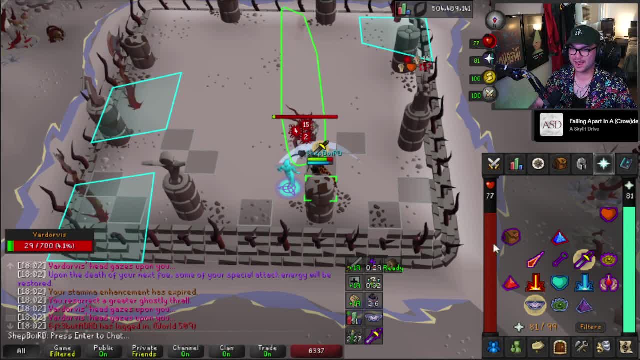 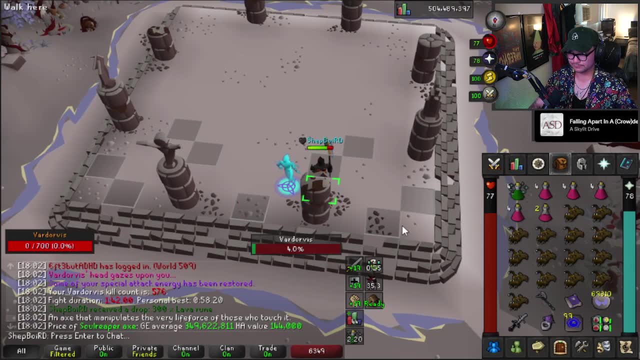 I hit harder with the scythe than I do the actual axe and it really sucks because the fucking axe is like 400 mil or something. Soul Reaper axe is the worst item in the game. Yeah, no, I agree, Churchy, I agree. 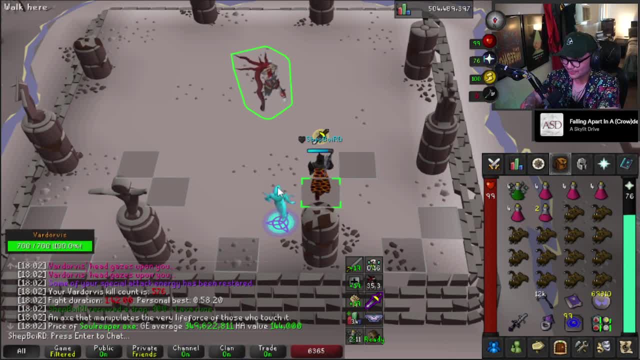 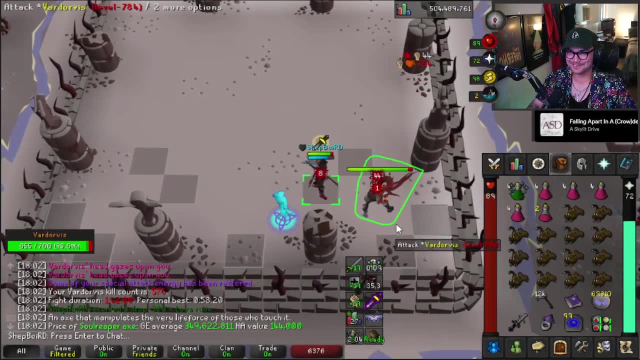 Also, I saw your DMs. I didn't mean to ego, We were, we were taubing, right, We were taubing. so I want you to know, like I promise, it wasn't an intentional ego, but I feel really. 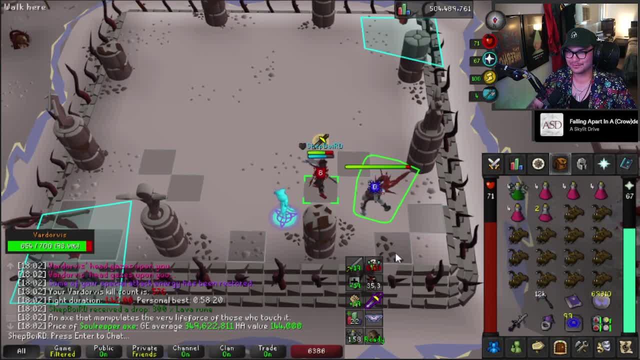 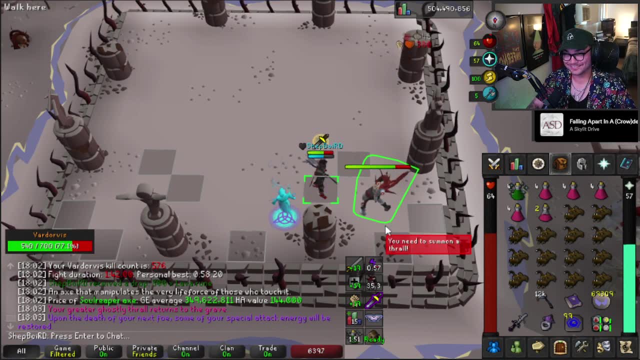 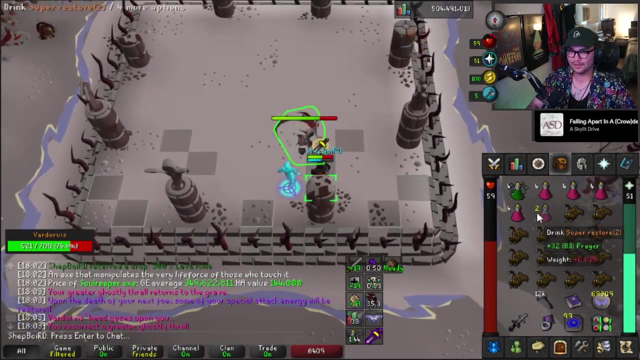 bad for you And, uh, I think we'll get your nib soon. I believe I have faith. Does it get better? Oh, brother, you're 10.. 10 times the KC. I got 10 times the KC. Um, I still need to go do like the the one. 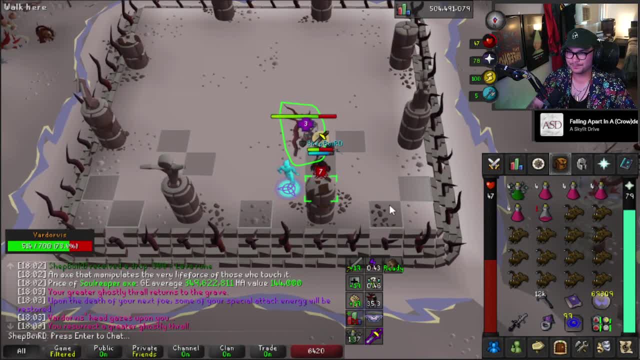 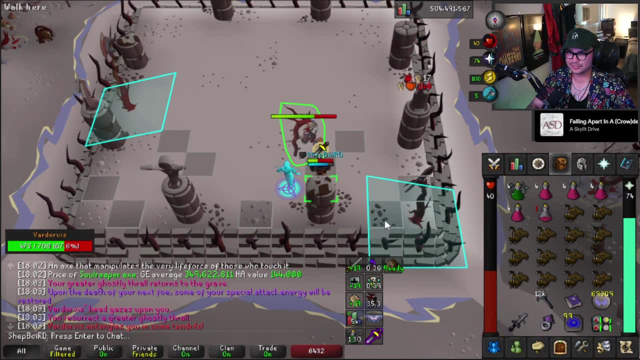 where, like, the melees don't dig, and then the one where, uh, let's see the jad skip, and then I don't remember what else the speed run like all that shit I have. so 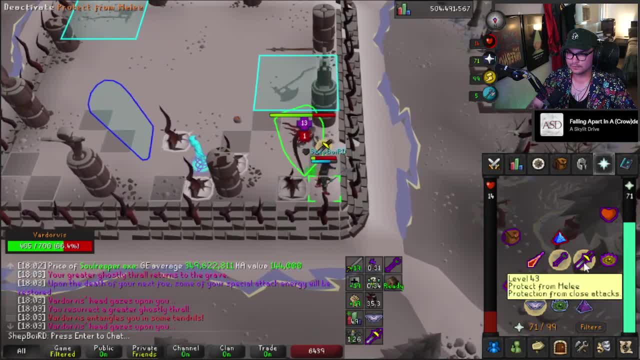 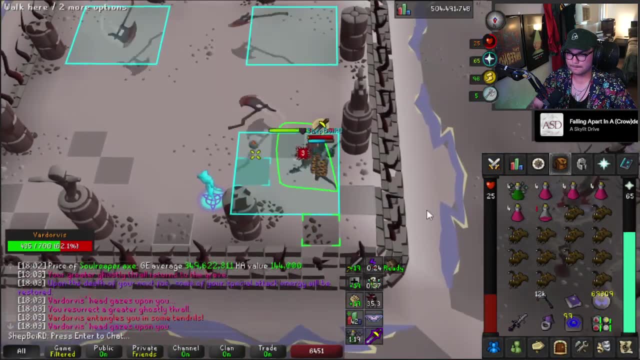 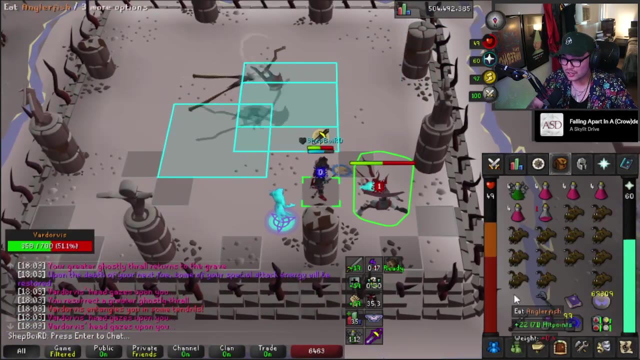 many achievements I have to do there. Okay, I definitely thought I'd click, but I guess not. I'm just gonna Gonna do that. Almost got a no no set. Holy shit, dude Fucking A. The last one I did. 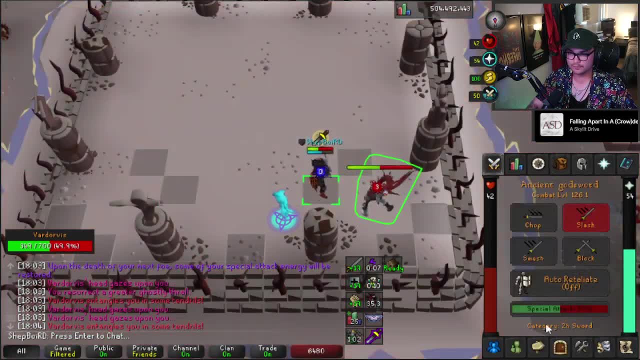 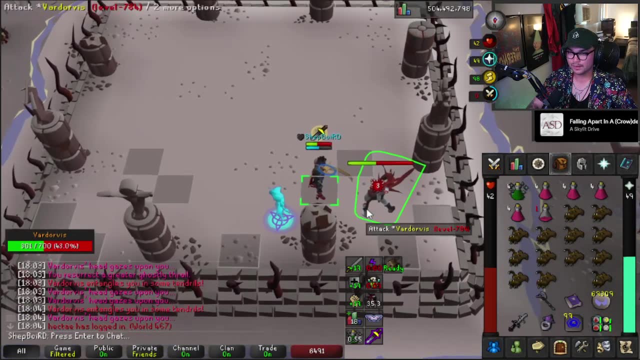 the zuck itself was uh pretty quick, But okay, nevermind. And of course we don't hit. We don't hit our AGS specs and that makes me sad. I wonder if it'd be better instead. 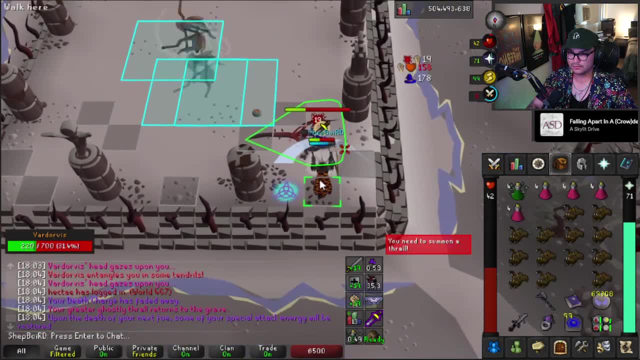 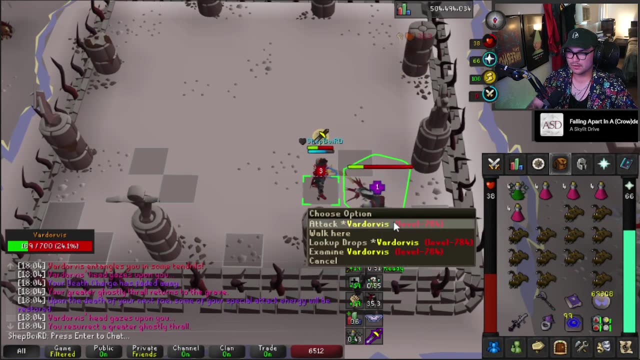 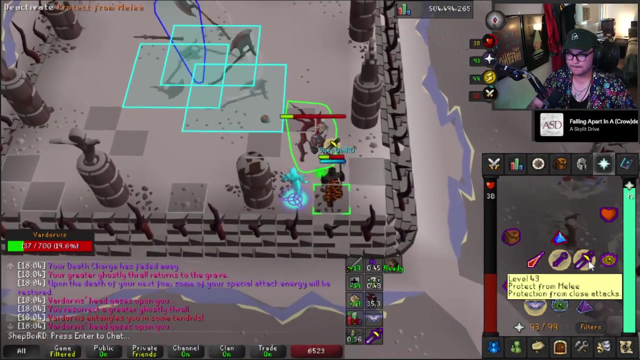 of being on, uh, The strength one, To be on accurate, So it's like the damage doesn't matter, But all my godswords are on strength. so, like I don't know, I wasn't sure if we had another. 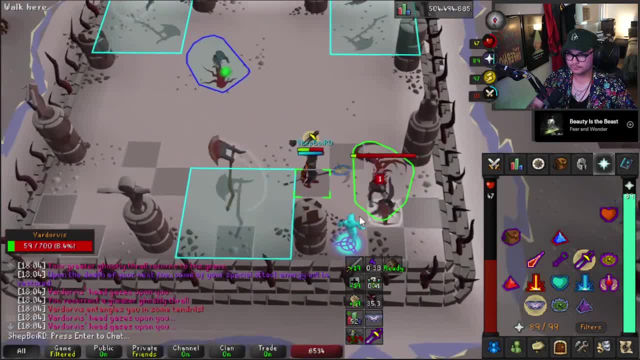 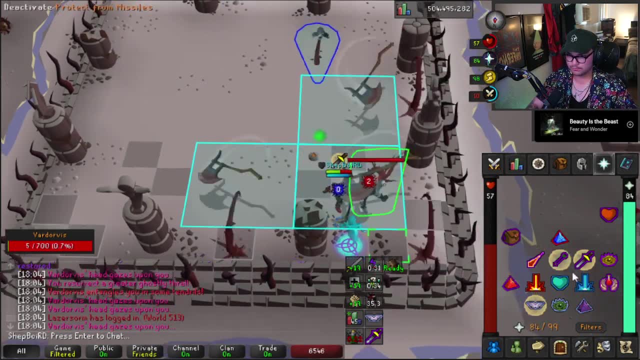 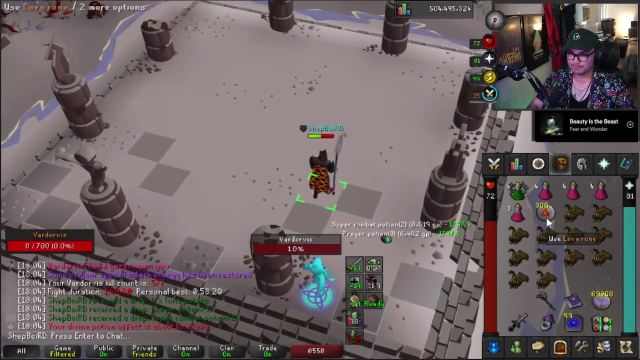 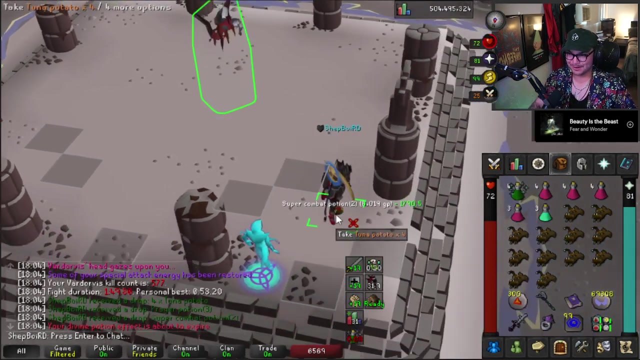 one coming. Maybe, Maybe we win the game. There we go. So I always I still pick up, like the lava runes and everything I get dropped Like I. I pick them up every time. I'm not gonna lie, I pick up everything, Even. 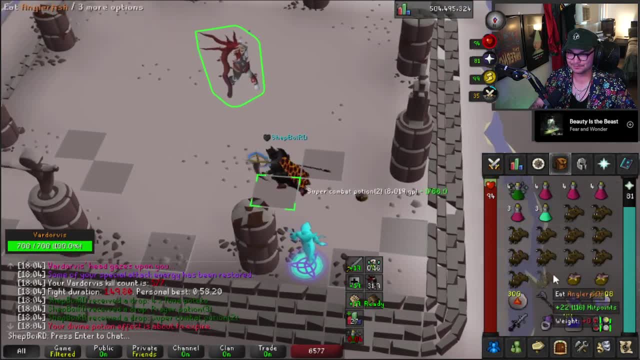 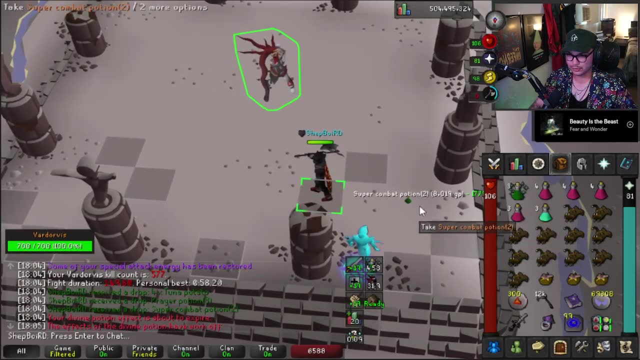 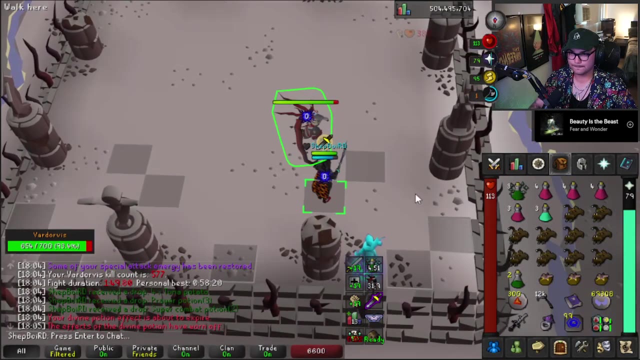 the uh, like shitty javelins and stuff Like I, I pick them up. Bam bam, Bam, bam bam, We'll eat another angler. Fuck it, Fuck it, Dude. I I've been kinda sleepy today. I'm not gonna lie. I got a lot of shit done, Like. 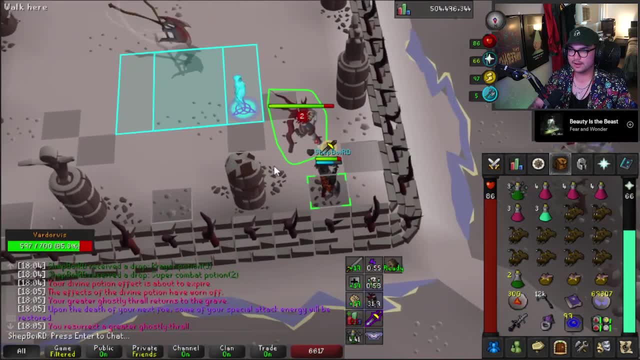 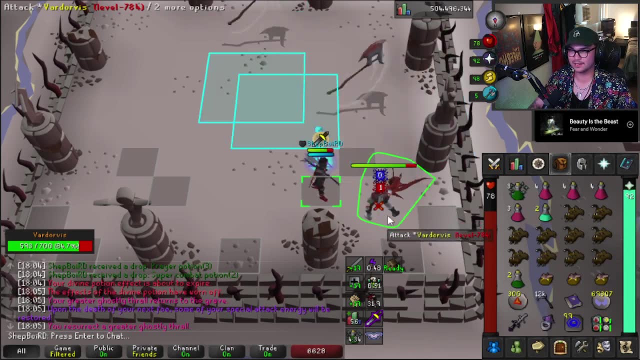 a lot of the chores I needed to get done. I got done, Played some helldivers. I didn't go grocery shopping like I needed to, So that's, that's a thing, And I I don't really feel like going. I don't feel like being a responsible adult. I guess It's just a whole. 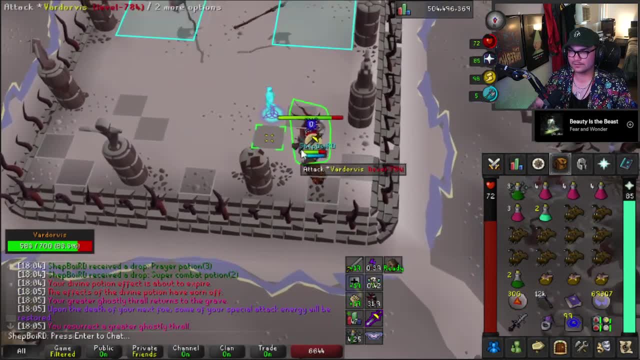 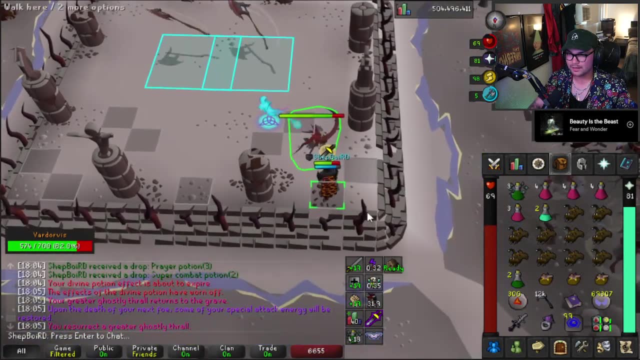 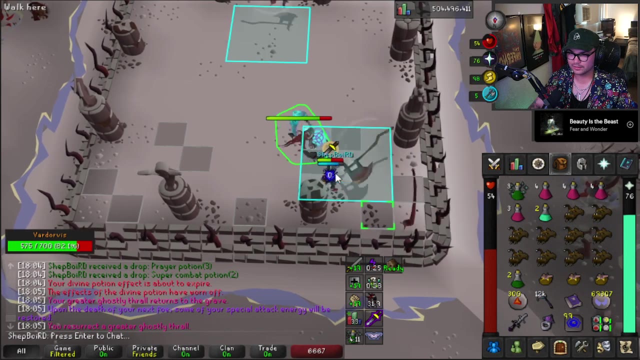 thing Like it'd be nice if the soul reaper was like actually accurate, Because like I know it gets accuracy uh, like as it charges. but it really doesn't fucking feel like it. It's like I'm sitting here just zeroes, constantly, Constantly zeroes. I haven't even 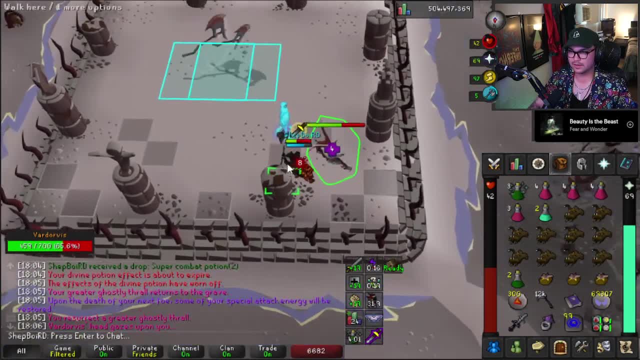 done the speedrun yet either. and, um, I mean, I've done a couple attempts and it's just like I'll hit a really good claw and then I'll be axing, and then it's like I hit nothing. Don't you down here. I'd just do that early Dude. my damage is. I don't know where my DPS is, but that's because it- uh, it doesn't. I thought it does. I could've swore it got. 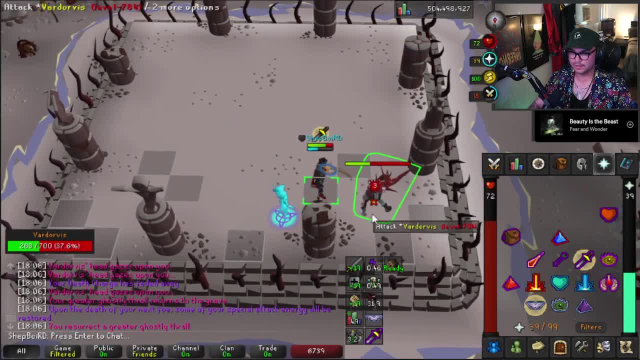 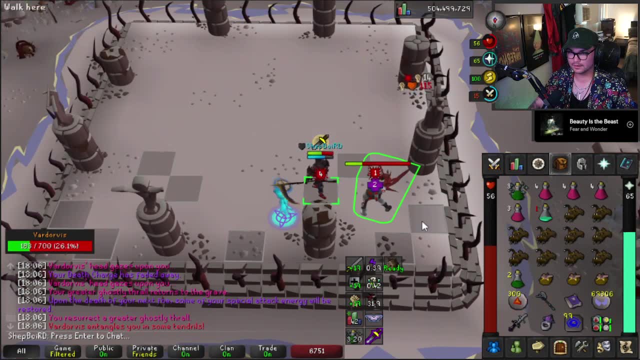 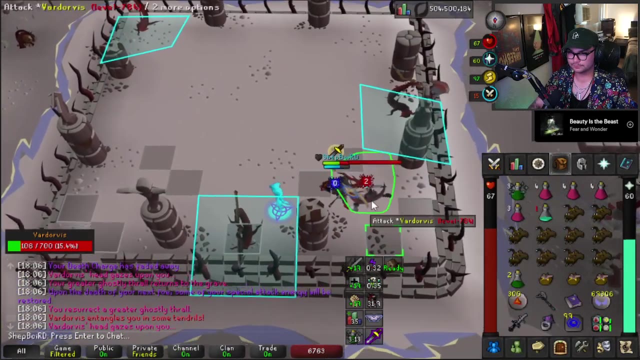 accuracy and damage, as it charges. But I could be wrong. You're better than me, You're better at the game than me. so, like you're probably right, Cause I, or is it just the spec? And the spec gives accuracy? Okay, Yeah, Yeah, cause I thought it was both. but Cause if 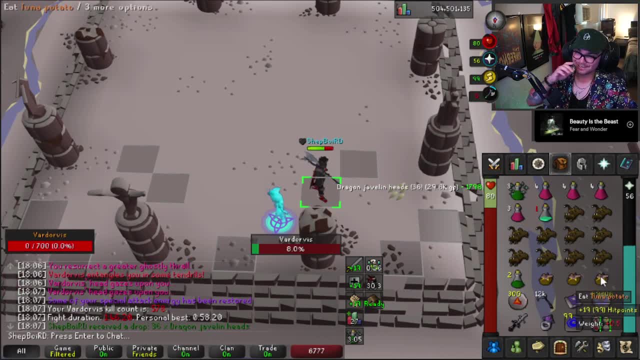 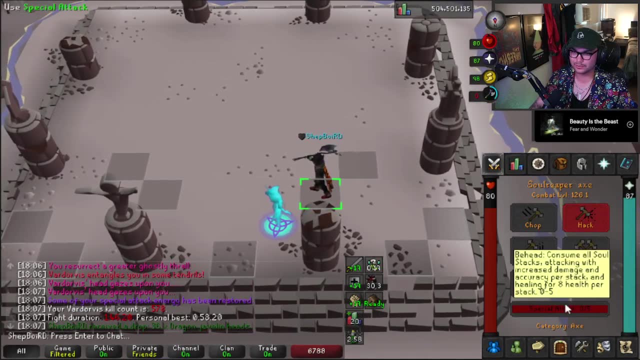 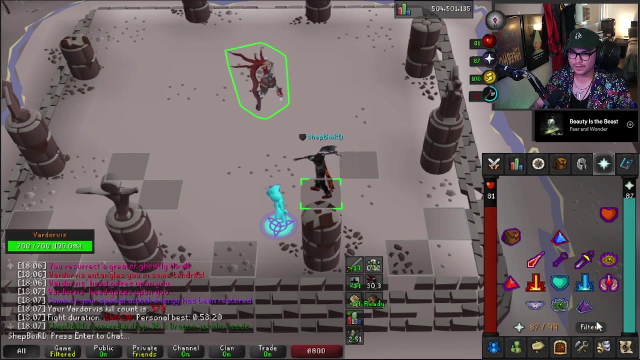 it doesn't, then it needs to Like. it needs to Cause it is so bad and it like- I know it's like still like listed as the highest DPS, but attacking with increased damage and accuracy. yeah, Oh wait. no, never mind. Okay, so it's just the the spec that gets. 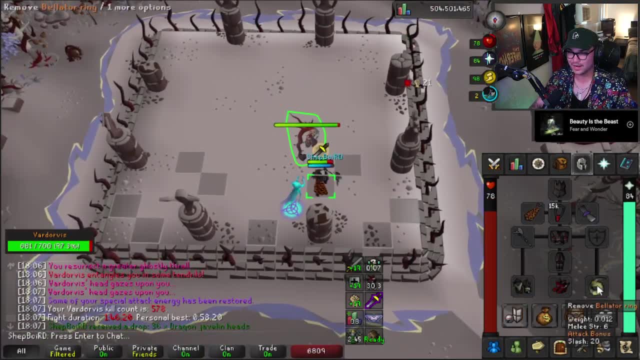 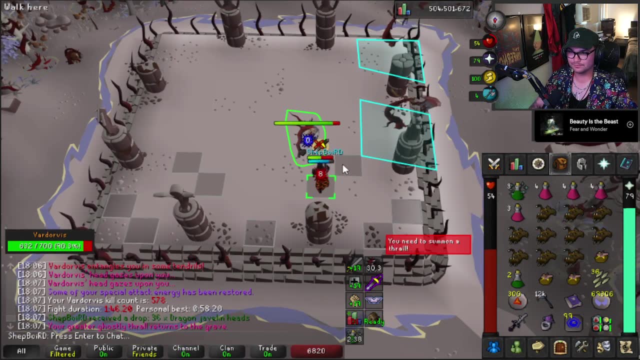 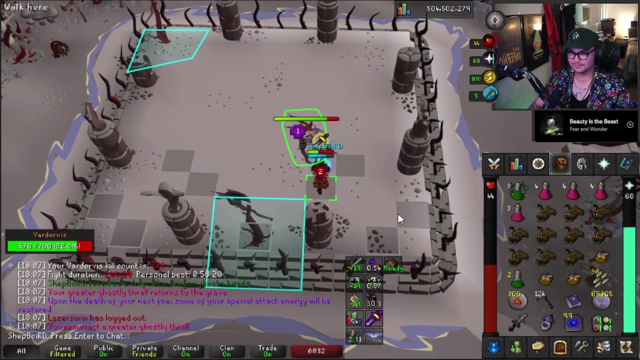 the accuracy buff, but even still like it just feels really bad. I don't know I got a bellator on and everything too Like it's just a whole fucking thing. Axe sucks, But this one I handcrafted myself. I went and collected all the pieces And I did it And 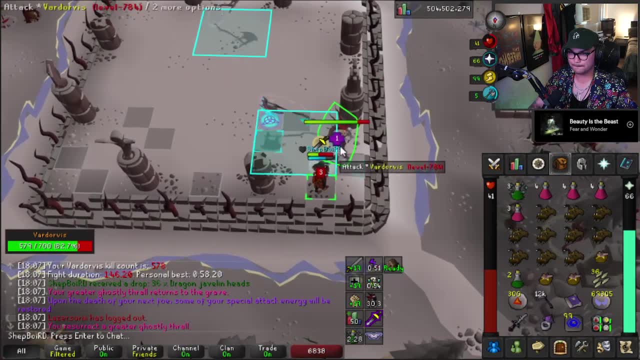 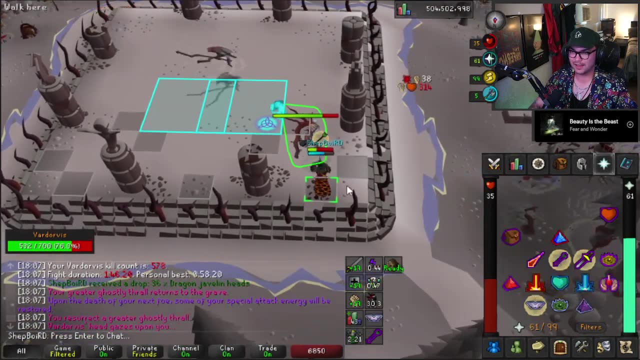 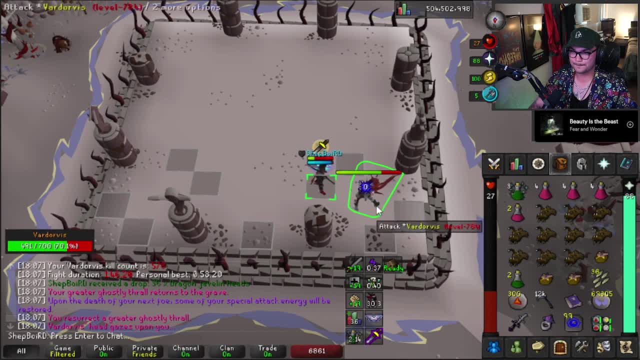 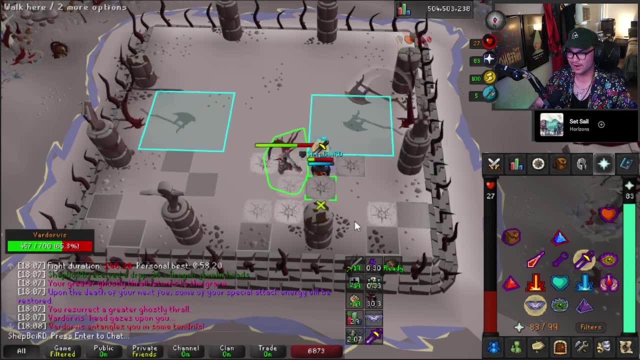 was the only one I got spooned and I got turbo-spooned, so I got it at like uh 100 and some KC. Uh duke, I got at 1500.. Levi, I got at 2064.. Whisper, I got at like. 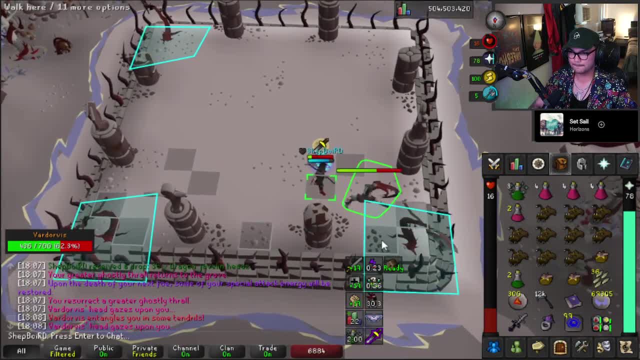 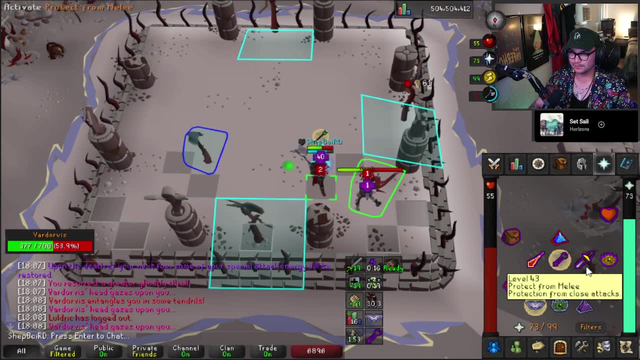 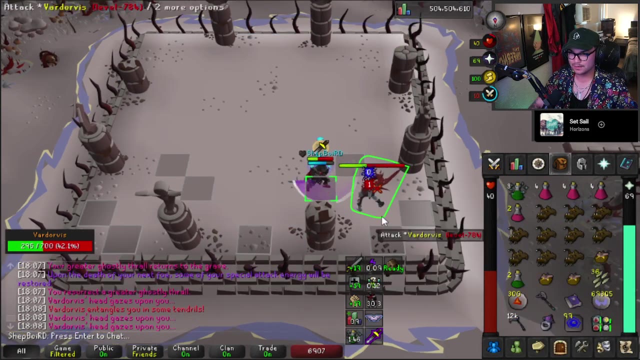 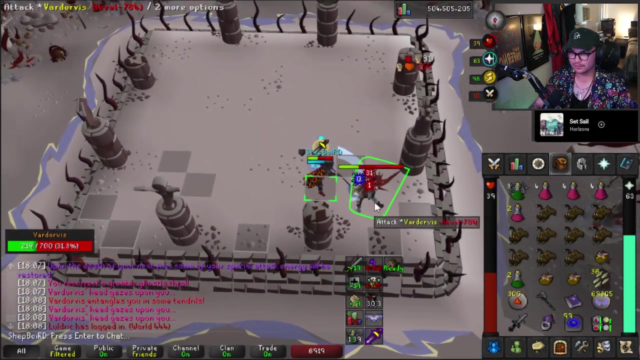 800. And my bloodfury isn't rocking either. I'm going to just spec and then scythe. I think Get some HP back, Get the HP-er back. AGS never hits. Blood Fury is now proccing at least, so that's good, I guess. 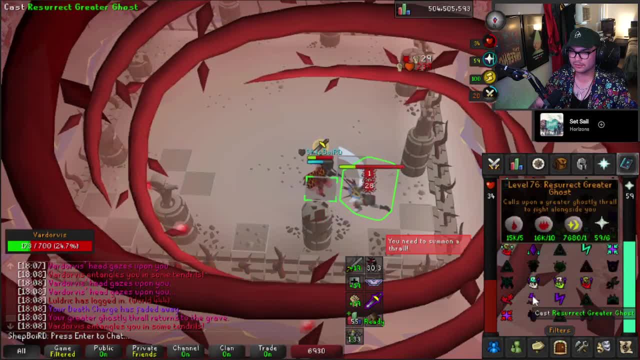 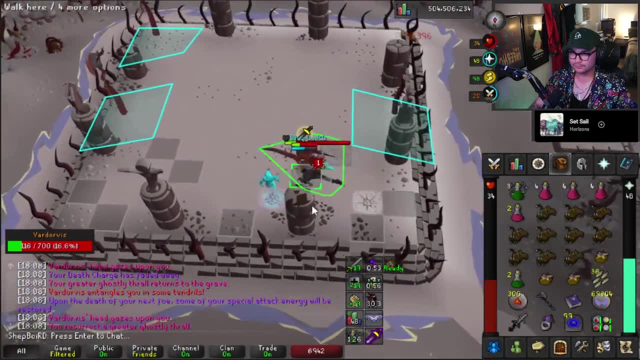 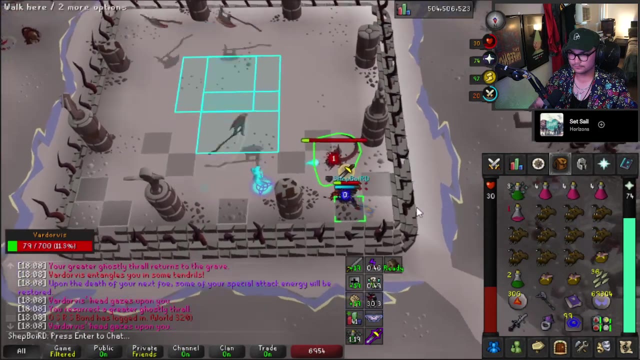 Dude. I kind of like I got to the point. now I can like sit here and like fall asleep at Bard. It's kind of nice. It's kind of nice. It's kind of nice, We're clicking. 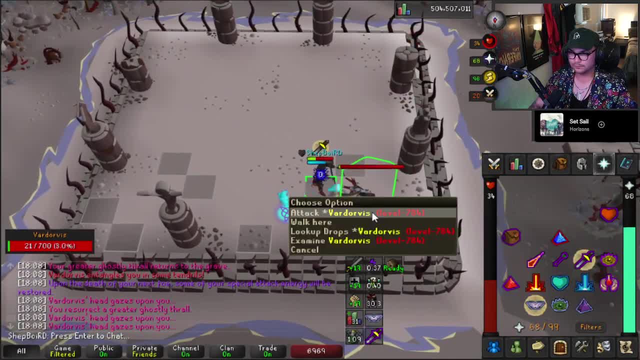 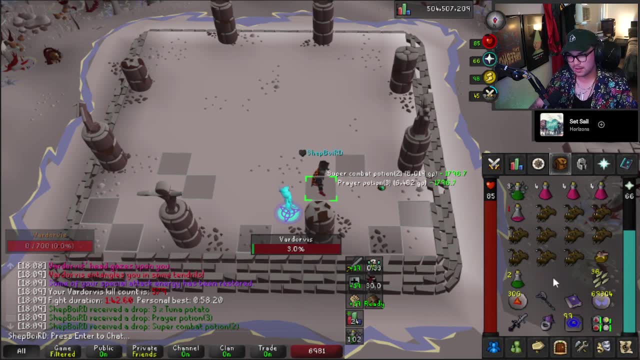 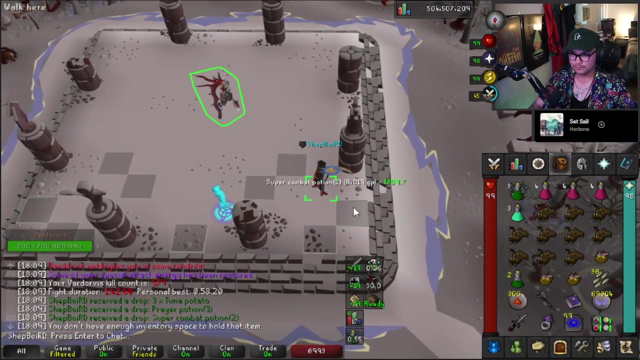 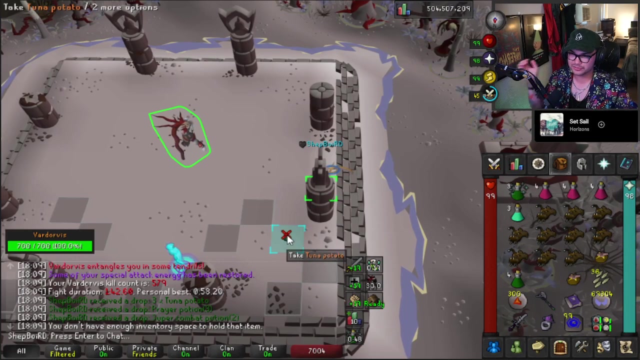 We're clicking So many supplies. I'm sad to be done with this boss. I really liked it. Yeah, it's uh. so when all the Desert Treasure 2 bosses came out at first, I didn't really like this boss that much. 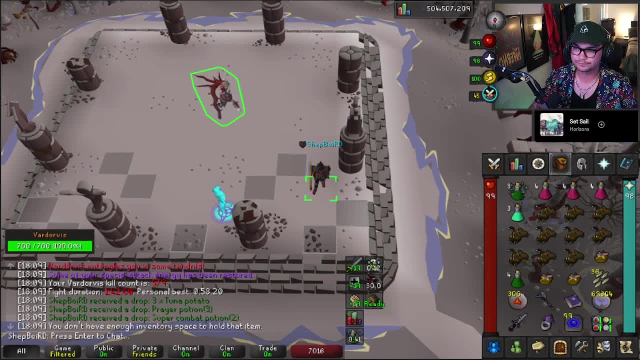 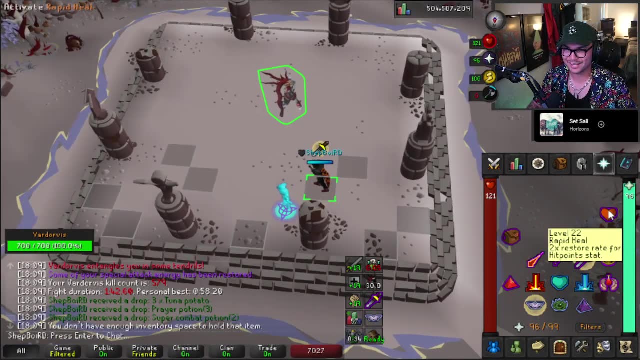 Like I wasn't like a huge fan of it, Um, and then I did 2KKC at uh, fucking at Duke and um at Duke and Levi, and now I'm like you know what. 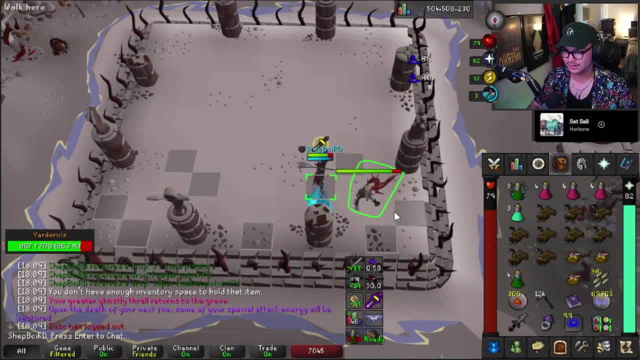 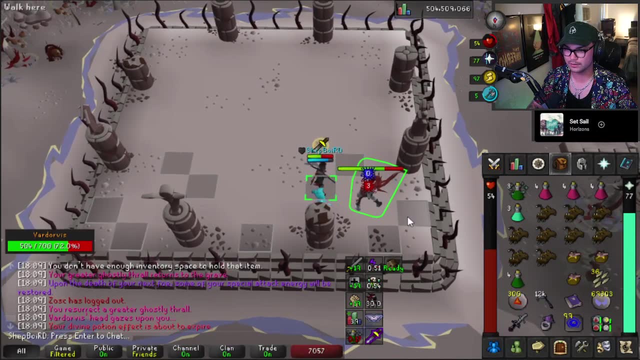 I did like 800. At Whisper and I'm like you know, I I think, I think Bard's okay I'm, I'm definitely like enjoying it more now than I was, That is for sure. 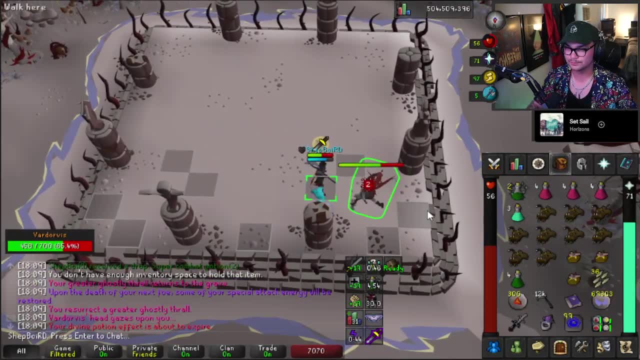 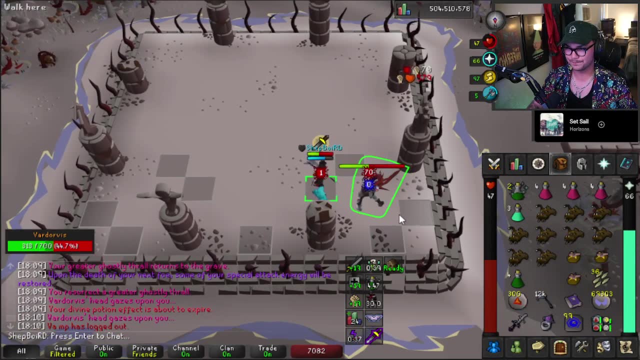 Because before, like yeah, I was just like I wasn't really having fun here, Um, but and then, like, when it came to Awaken, this was the one I struggled the most with. Um, I'm done with Levi and Bard. 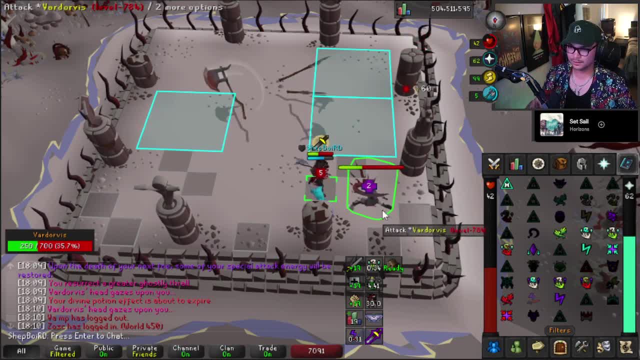 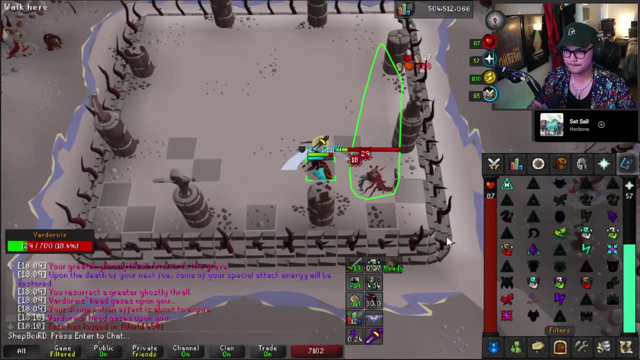 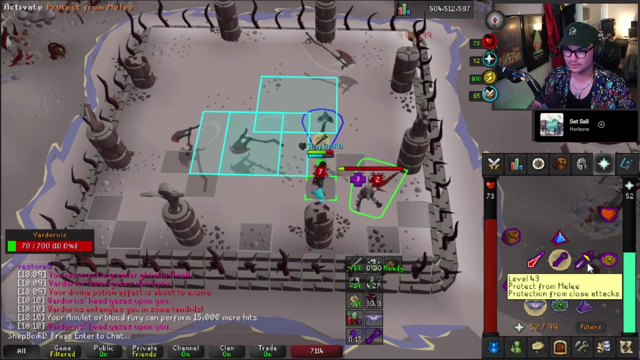 I really dislike Whisper. Yeah, I, uh, I mean I still have all the like GM speedruns. Holy shit, we're kind of cooking, Kind of cooking Dude. I, I like looked away and then all his health is like gone. 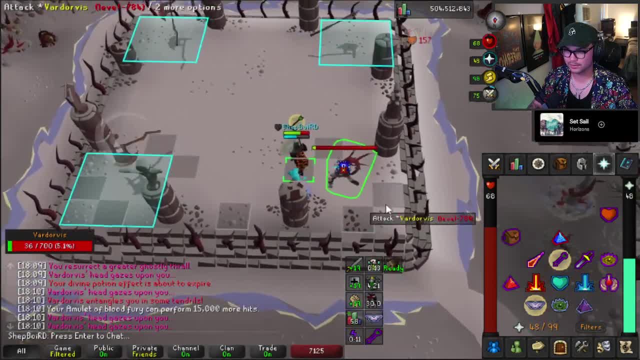 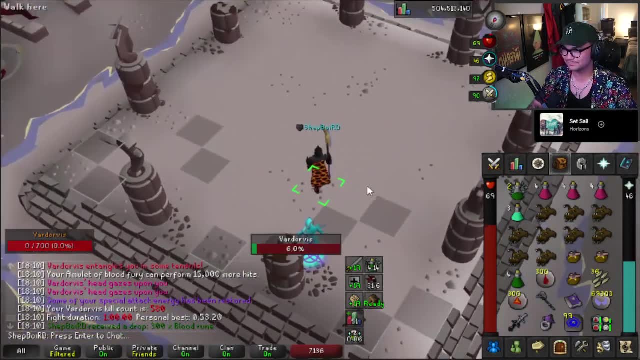 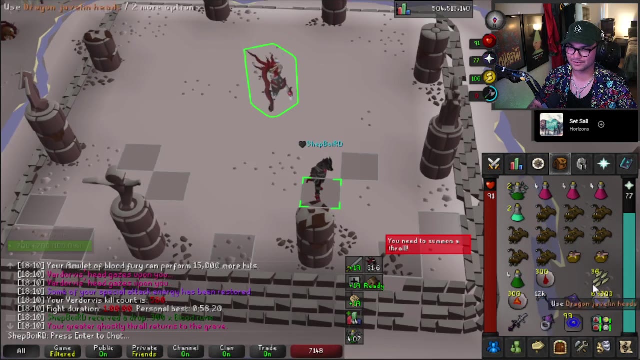 Let's see, I'm clicking hard as fuck. I'm clicking so hard. That was that felt fast, I don't know Exactly one minute. I did the GM speedrun before the babies won. I mean I haven't got er, I haven't gotten any of the speedruns. 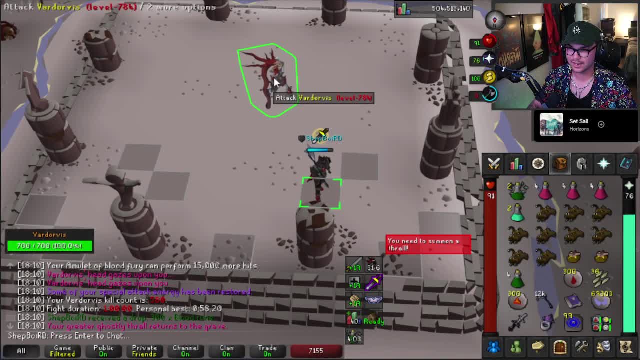 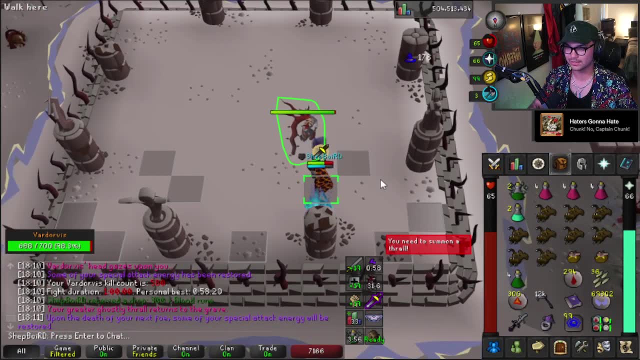 Like I don't know, I did 2,000 KC at Levi and I my PB is still like a 113 or something Because, like I don't know, I never get the like 12 ZCB specs or Ruby Bolt procs. 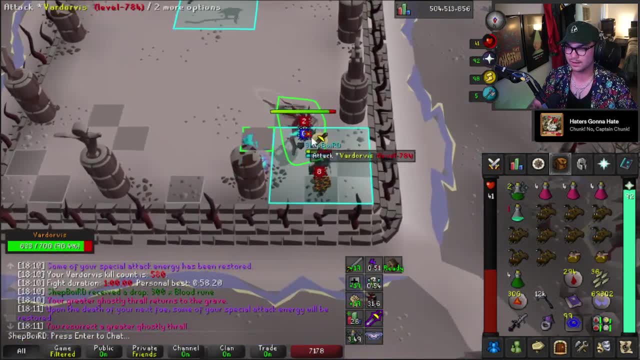 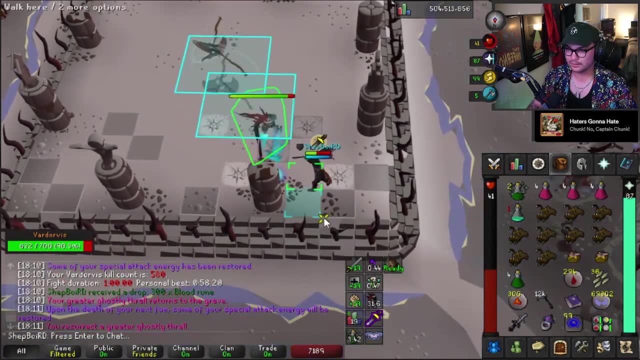 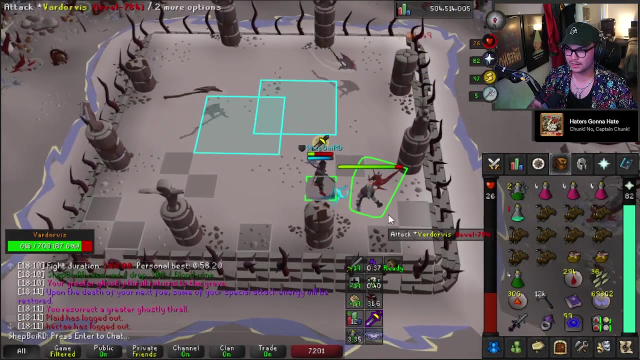 I mean, like I think the most I got was like four- I I'm not sure, And so I don't, I don't know, But I guess, like to be fair, I also never uh, I never uh ZCB and brought uh the thing. 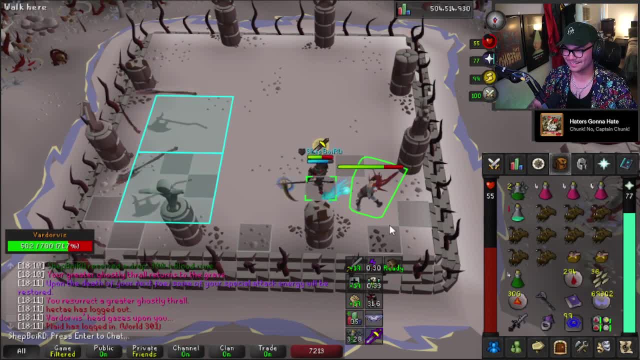 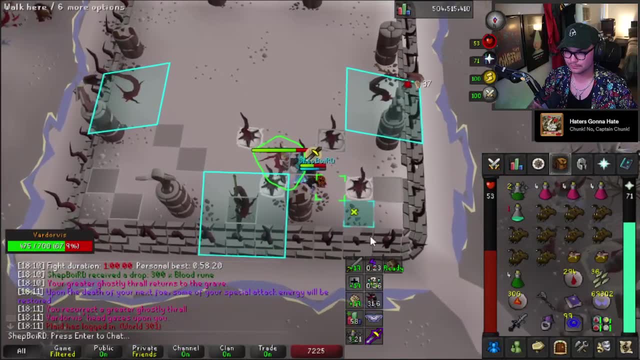 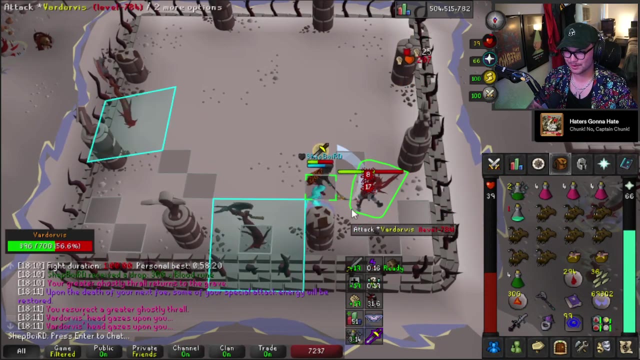 Herb GM. Dude, I literally just talked to you. PB is insane, Did it off the ass. ZCB just went hog wild. Dude, I fucking win, I fucking win. So like when Bard is not in this 2x2 square like I, I get a little annoyed. 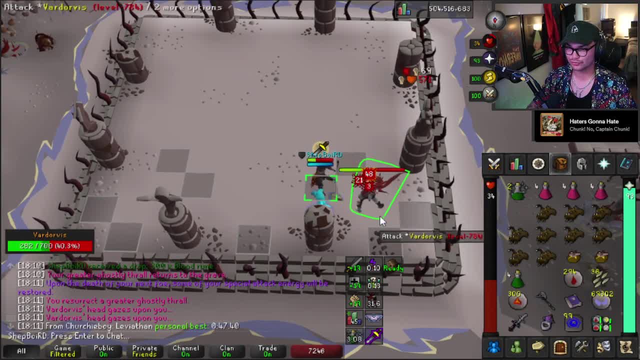 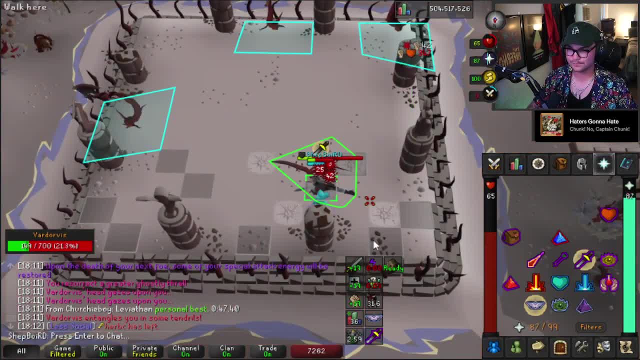 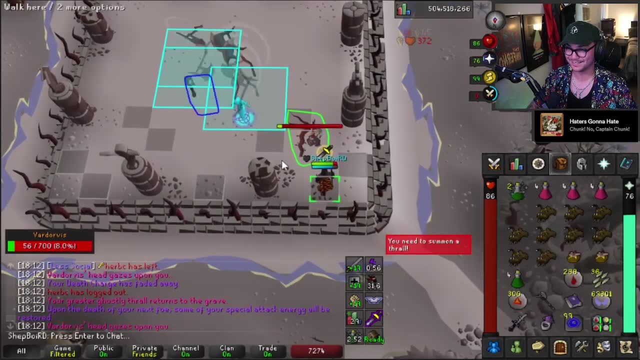 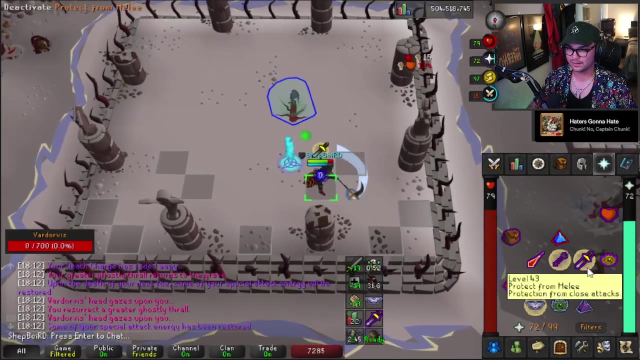 You fucking cooked him, Churchy. What the fuck? Yeah, that is a absolutely cracked PB dude. That is an absolutely cracked PB Like I don't want to like start going Bard again, um to try to get this speed run. 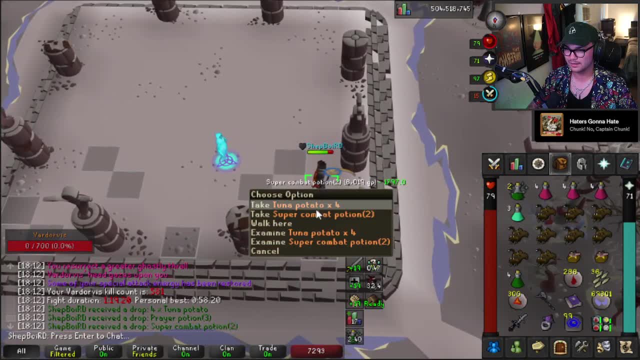 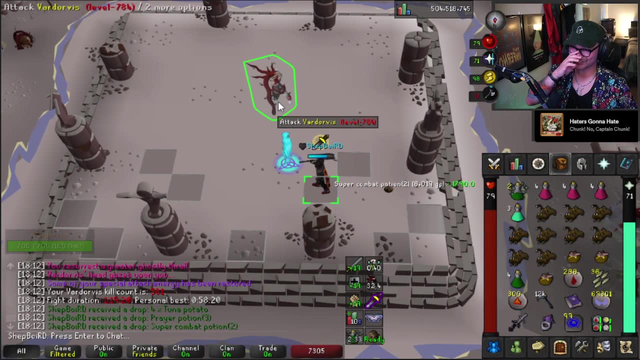 Like I have all the other combat achievements I just don't have. I just don't have, um the the thingy, the speed run, I got the GM doing the five perfect kills, Shit, dude, Yeah. and like I would never bring both. 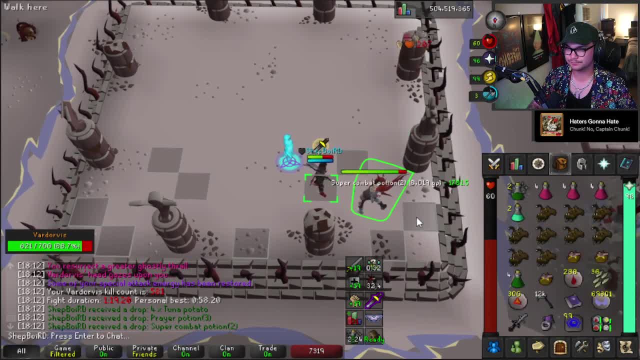 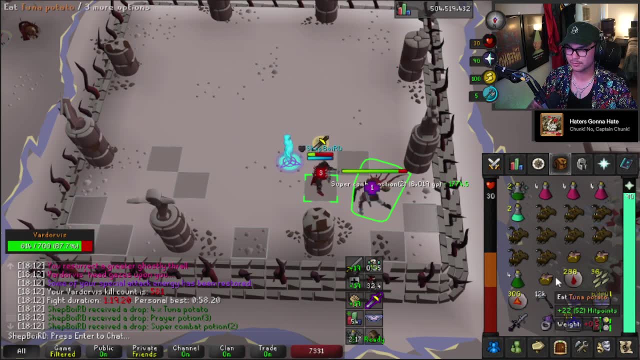 Like I would never bring both ZCB and- um, what's it called? Uh, or I might have on like one or two trips, but ZCB and Webweaver, because most of the time I was like, well, I'm going to use my ZCB spec, you know. 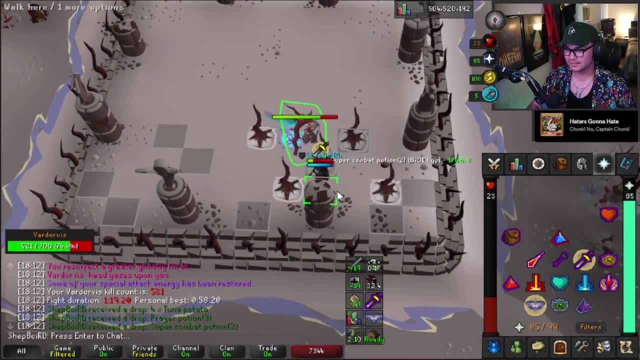 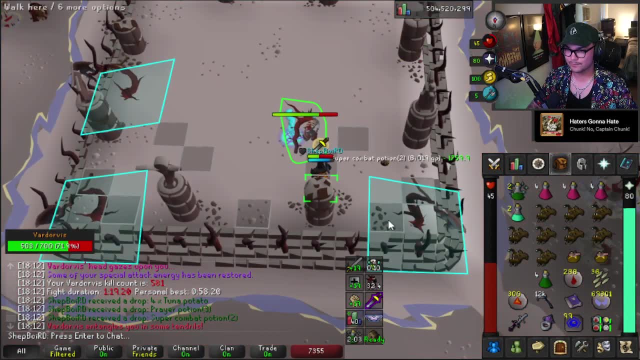 So I don't, I don't know, It's in the Oh freest. I thought you said fastest and I was like what the fuck I keep forgetting there's like a free eat there that you can do and like not lose. 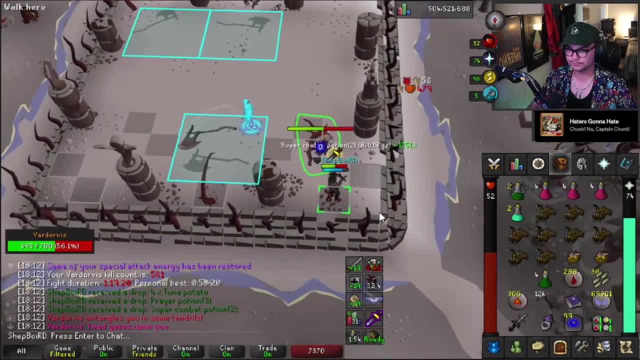 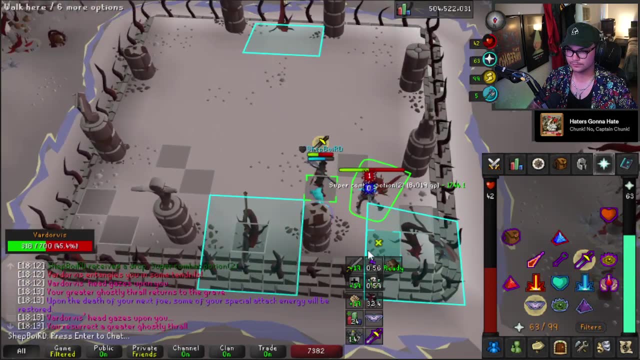 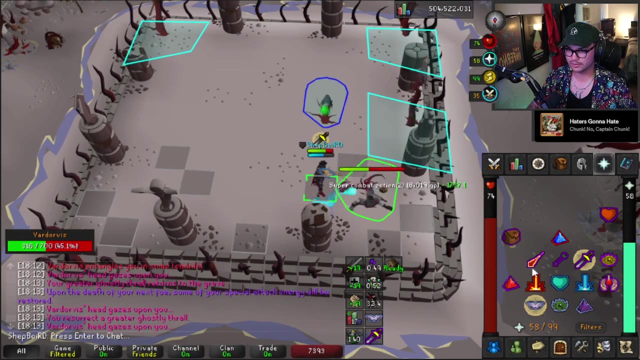 ticks and everything. I think it's at the end of it. I don't know. It's either free eat or free hit. I think you eat beforehand is the move. I don't remember. I remember as a thing like when I first did Desert Prover 2, but I'm not sure. 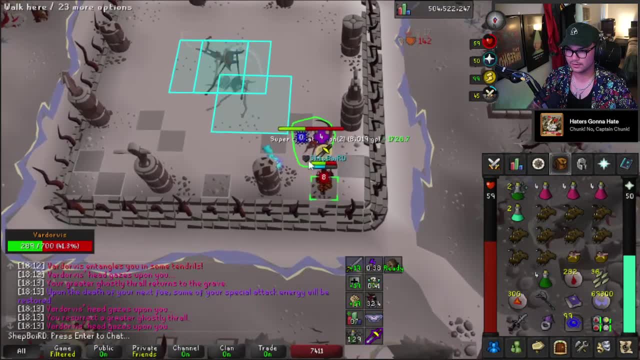 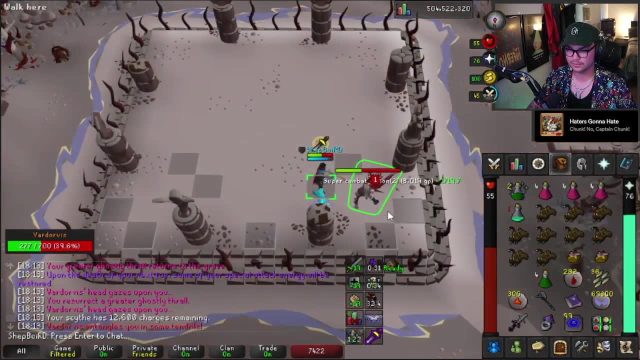 But yeah, I mean, it's mostly just, uh, get lucky on ZCB specs, and so I don't know Because I I want to try and hit GM this year. That's like the main goal. Uh, I know, during the charity stream I said I was going to like max this year. 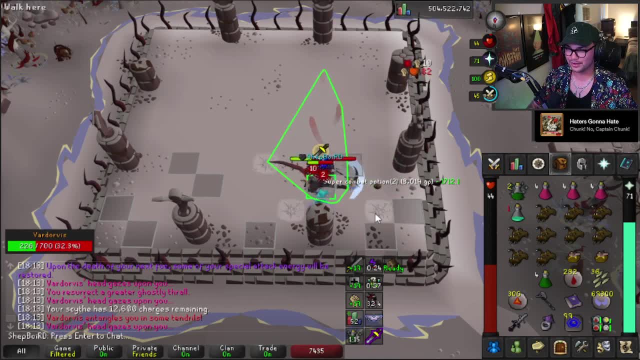 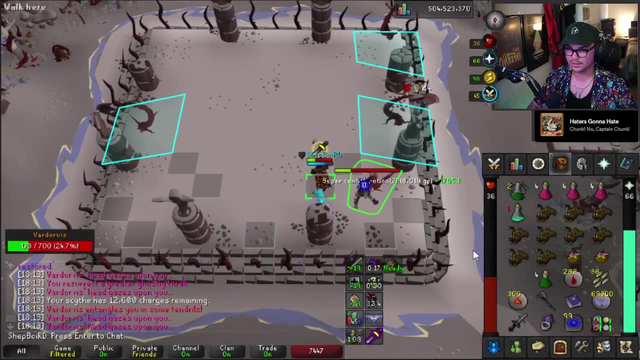 I don't think I could Like there are theoretically enough hours in the year That I would be able to max. Uh, if I like did max efficiency stuff all the fucking time, But I don't want to three tick mine. 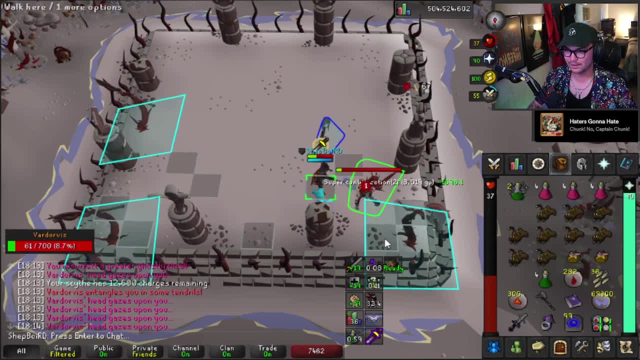 Like I don't want to, like do the- uh, what is it? Uh, one and a half tick. Like one and a half tick ticks. Like I don't want to do that shit, I'm not going to lie. 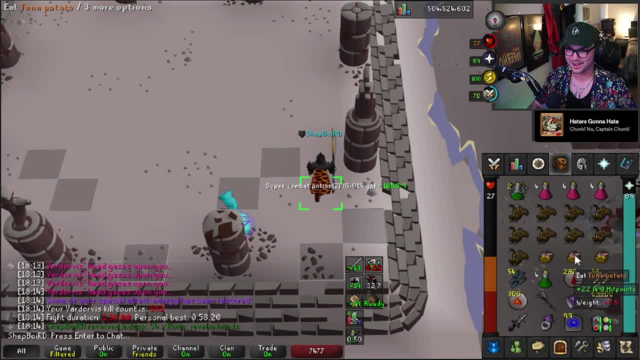 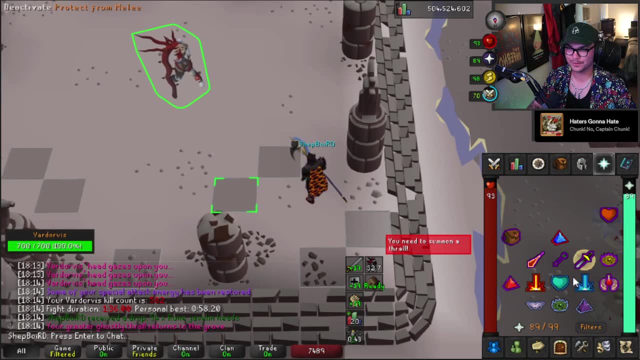 Like. I am not a max efficiency player by any means. I'm not good at the game, You know what I mean. Just a whole thing, And so, uh, I don't know, Eventually we'll max, but uh, 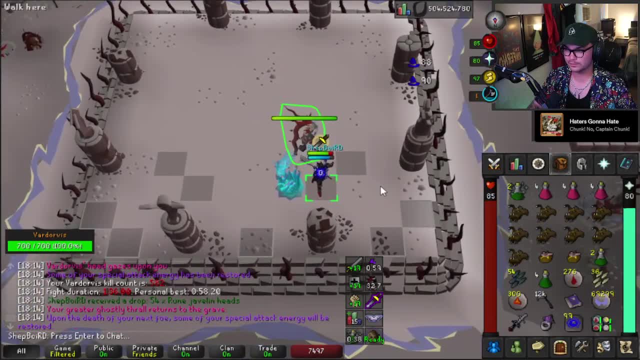 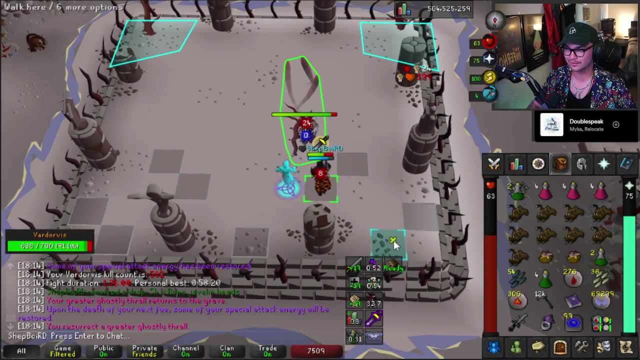 We will start working on it. We will start working on it. Gotta get those Toa CAs. Yeah, I know Those are going to be like near the end. I'm not going to lie. Woodcutting is fun. 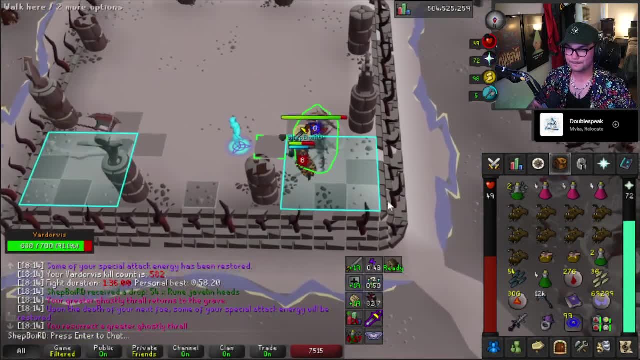 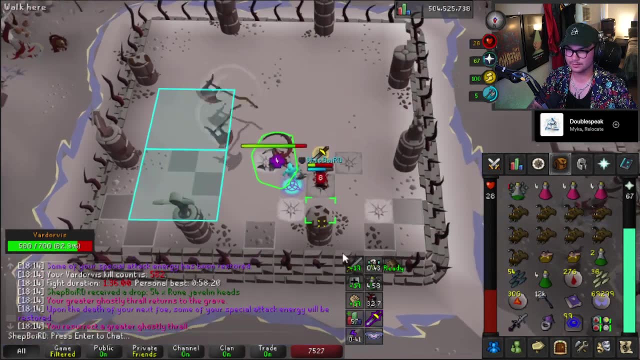 I have a lot of experience in it. Uh-oh, Uh-oh. Now what we might do. What we might do, Uh, is start PBMing on the ult Once there's two more kits I want to get. 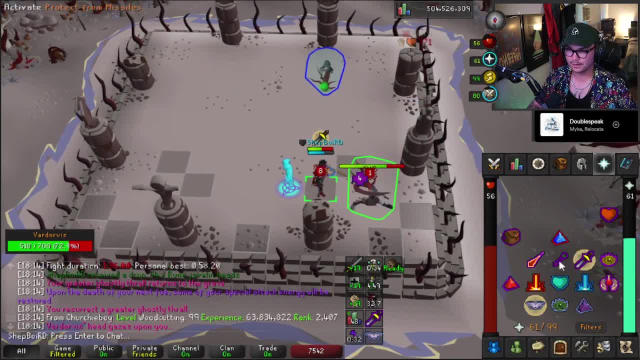 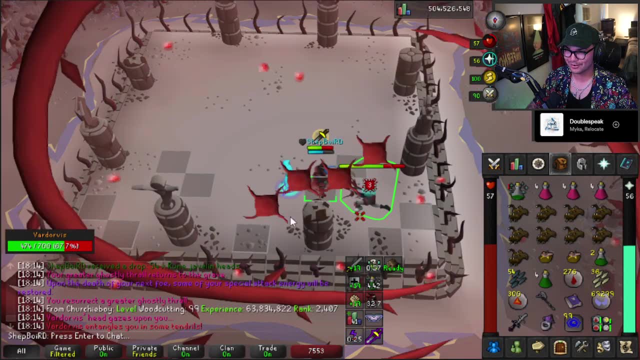 Um, like I want to get my Sankit. Um, and I want 64 million Churchy. what the fuck are you doing? Are you like playing on an iron or something Like I'm just woodcutting on the main. 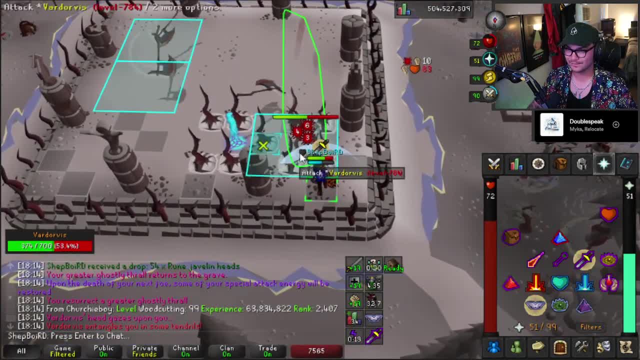 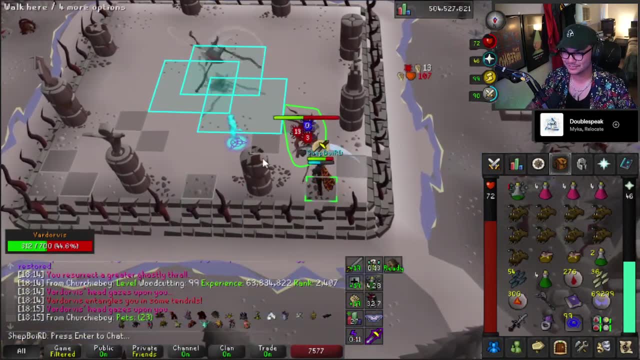 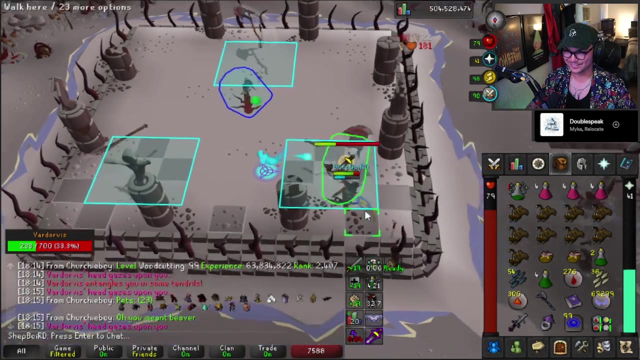 How many pets do you have? I feel like that's like a two-petter Clicking trees. obviously I mean okay, smartass, Okay, Pet Jesus Christ dude Clicking trees. But yeah, um, I meant beaver. 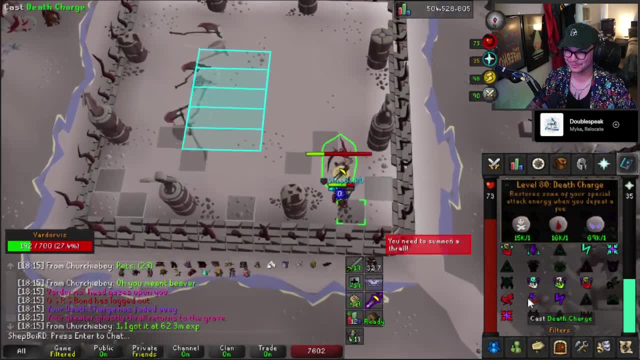 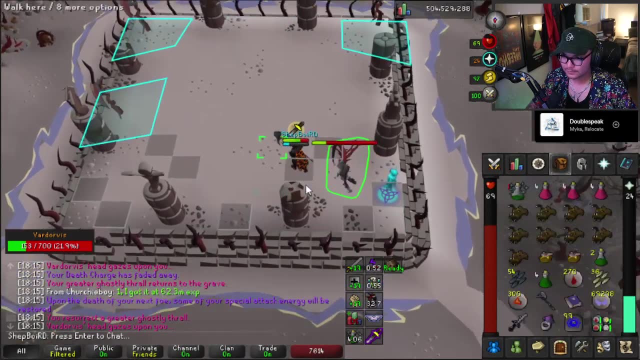 Yeah, Yeah, I meant how many beavers, babe? One One, That's it. That sucks, I'm sorry. I'm sorry, I didn't mean to bring up, like you know, a touchy subject. It's my bad. 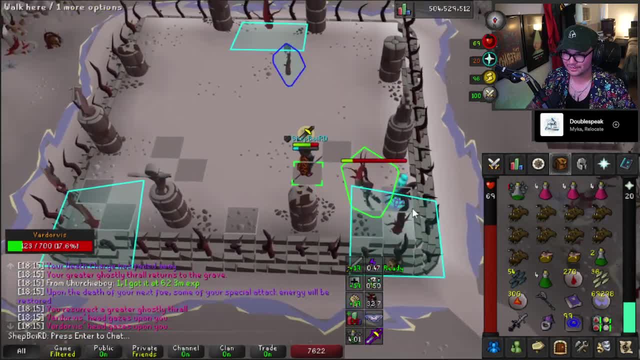 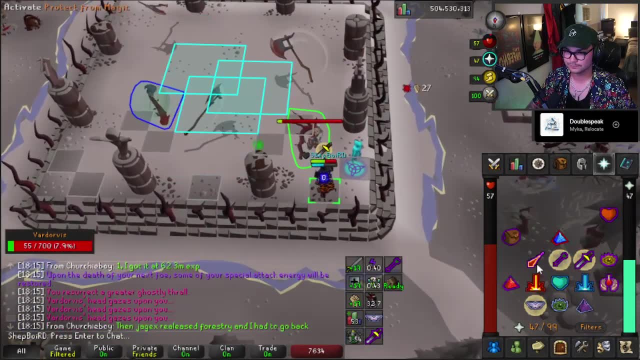 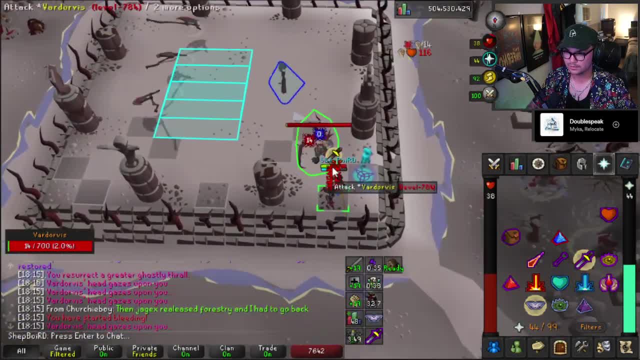 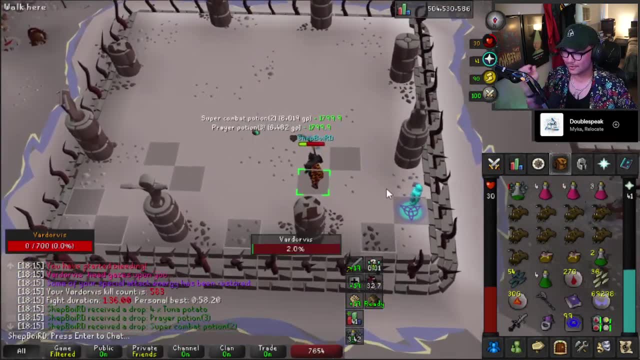 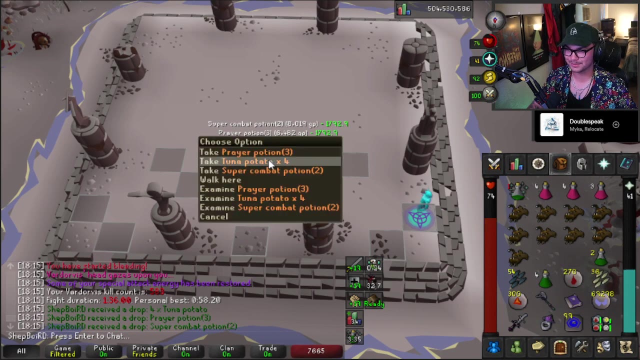 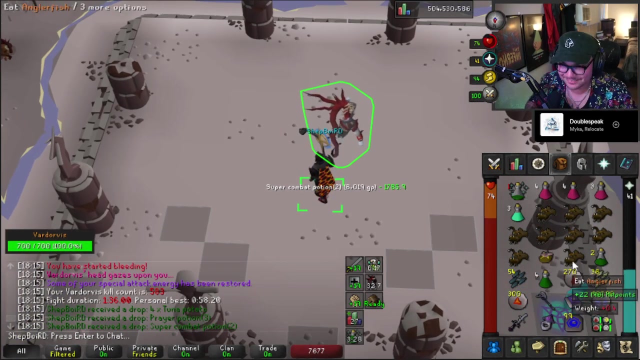 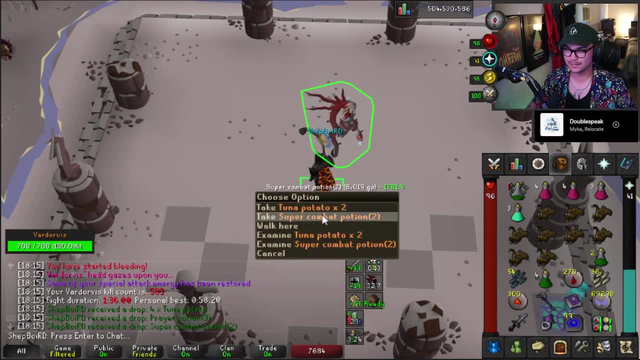 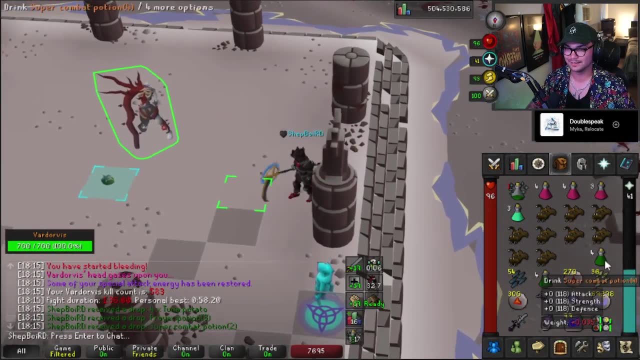 I could not do that. I could not do that. Although I am probably going to hit 200 mil range, like before I max, I'm not going to lie Like look at that, i got 504 mil total. like it's kind of a lot, i feel like i feel like it is anyway. 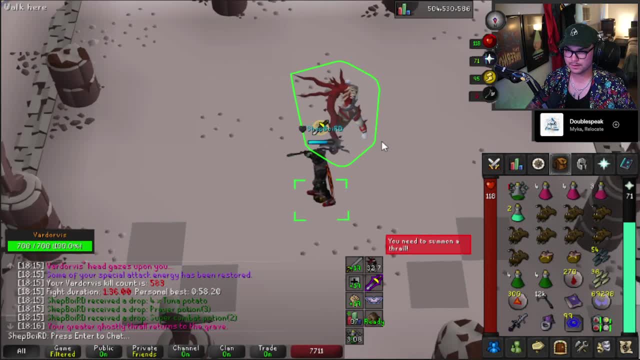 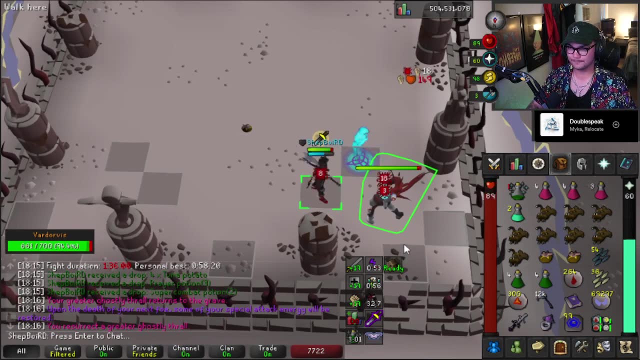 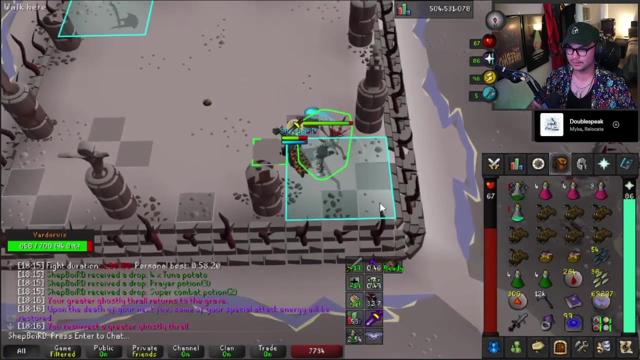 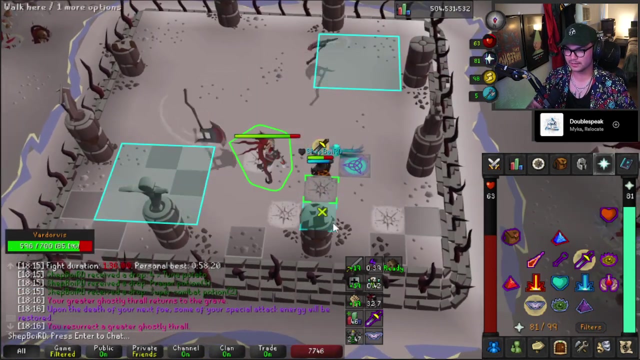 uh bam, bip, bop, bippity, bop blam. but yeah, i definitely need to just start multi-logging and, uh like, pbming on the alt. we could do like a little alt progression series. i don't know, because i still don't have a desert treasure 2- and then, uh like, since it's basically, i mean, it's going to be a main, it's not? 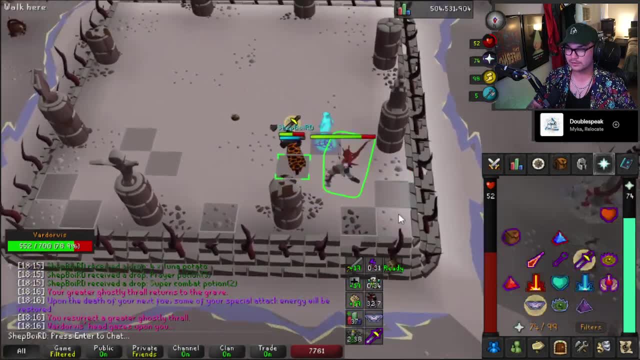 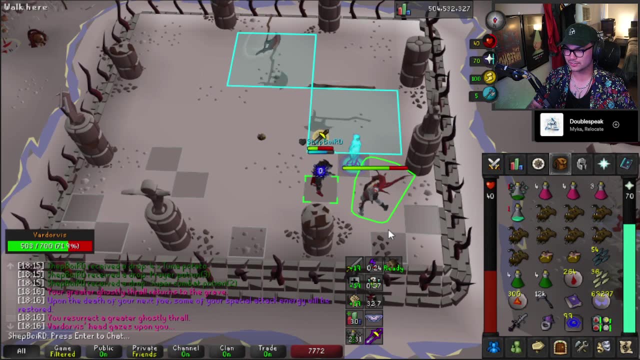 gonna be any bracketed thing or anything i could start. uh, something i kind of wanted to do was do like a zerker. i'm gonna do toa with a completed version of my alt. yeah, like i mean, i don't know, because my alt right now is just like a general pbm alt right. 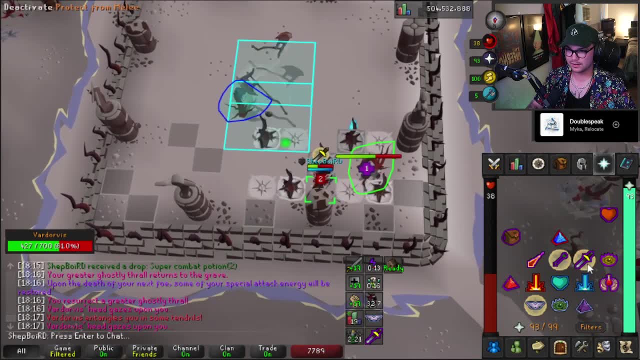 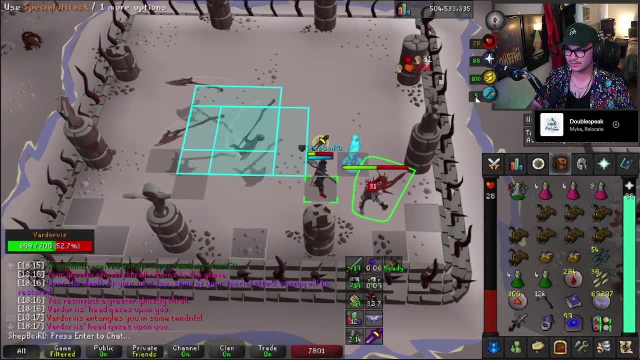 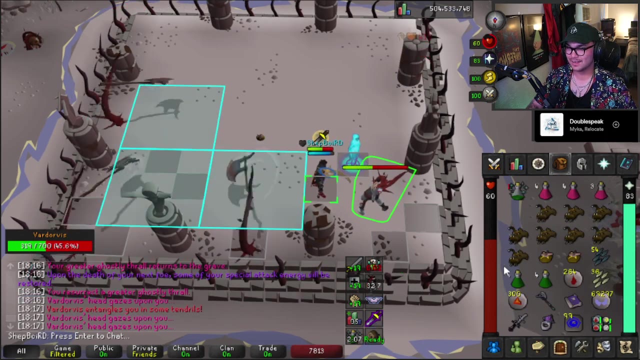 um. so it's nice like having banj and um, i would like to get the desert treasure 2 done, just so that i can like have a supply alt out here, um, because i don't have one. my second alt is chilling in nightmare zone still, yeah, and i mean like i don't know. it could be fun. 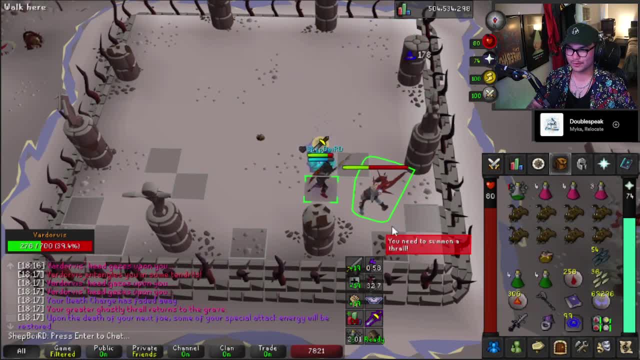 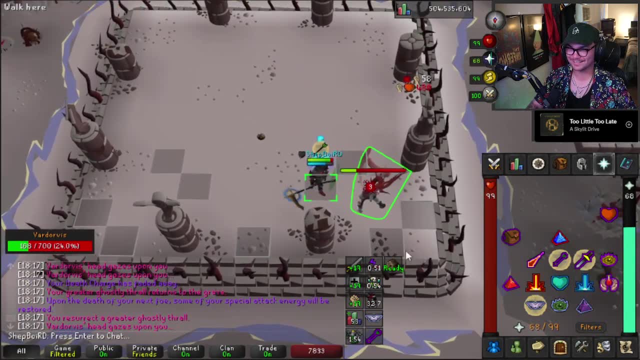 what if i? what if i made a hardcore? what's your thoughts on that? i'm just kidding, it'd be a nice like. what if i made a hardcore? what if i made a hardcore? or two streams? you know, do it, you won't uh for 750 000 channel points. i will. 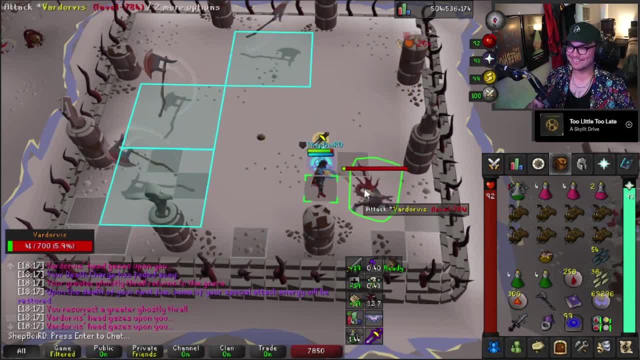 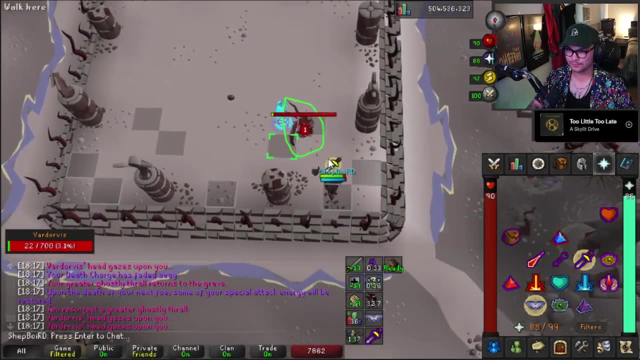 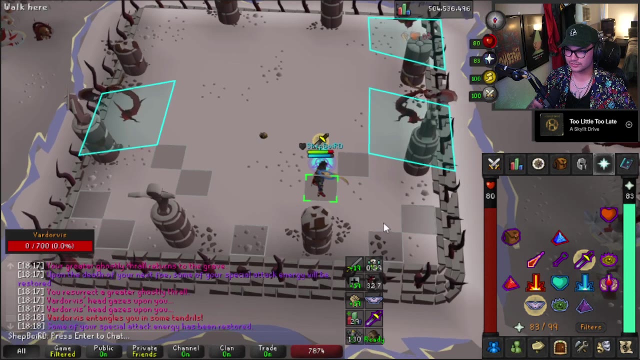 750 000. i feel like i feel like a content creator. uh group hardcore would be fun. i feel like that would be really fun. both my alts have desert treasure 2 done, so it's just a matter of time. uh, before the dude grind starts: oh shit, that's my alt, so i'm gonna do it. 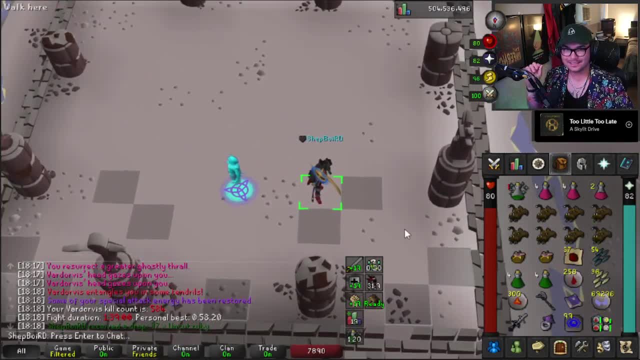 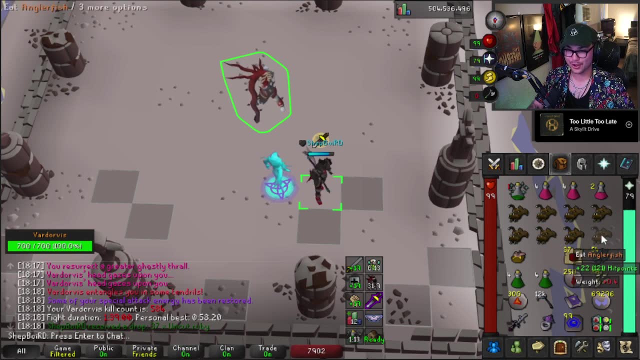 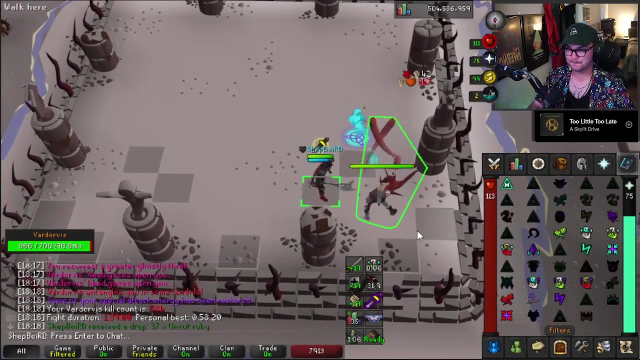 i'm gonna do it. i'm gonna do it. you know what i think? i think that's my favorite pet in the game is the dukerton. i do a group hardcore. oh bet bunk would do it with us. i don't know, i don't think bunk would do it with us. 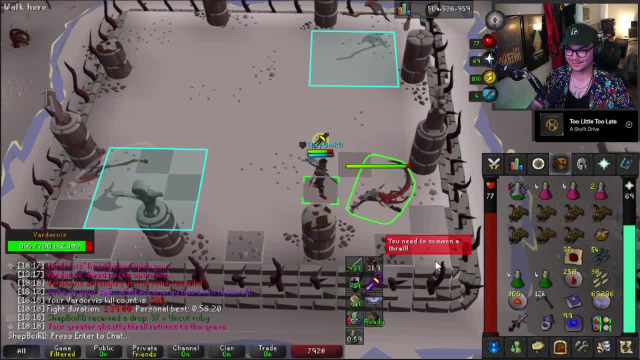 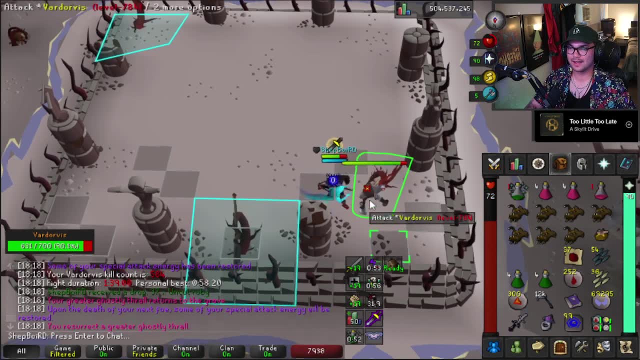 i think that's a little more faith than uh, uh, than i got, i don't know, i don't think i'm gonna do it with this, i don't think i'm gonna do it with this, i don't know. i feel like i feel like for content, like uh, i mean, i watched a little bit of the. 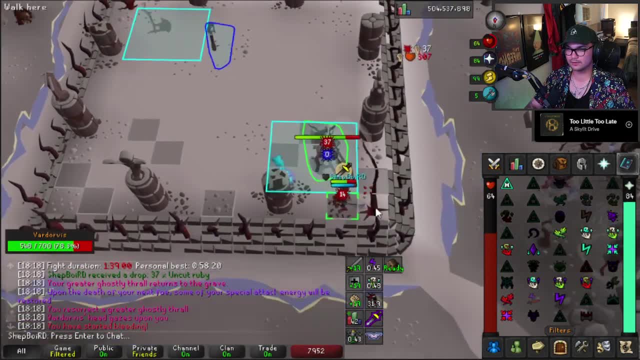 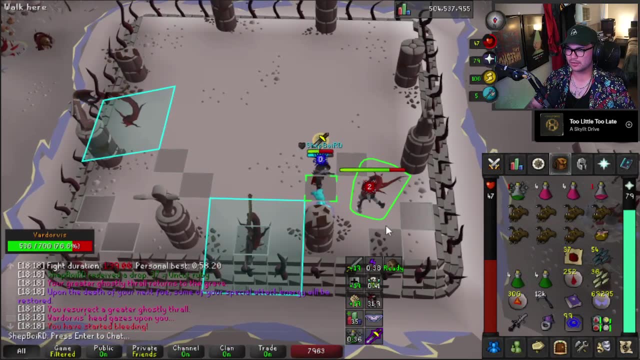 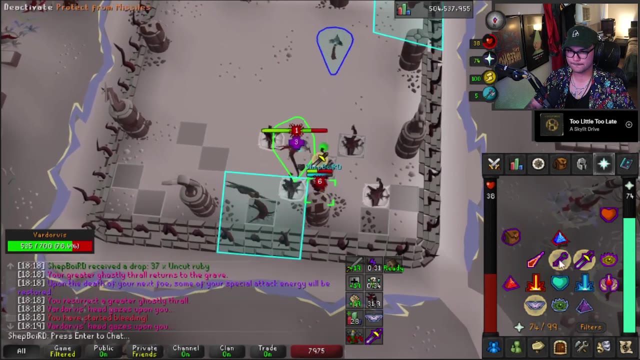 farmers. but like i watched a lot of odas- i moved so early. i watched a lot of odas, uh, group hardcore, the one, like are pretty much all of them, yeah, like uh, even this last one, i don't know, and uh, i think it'd be, i think it'd be neat. 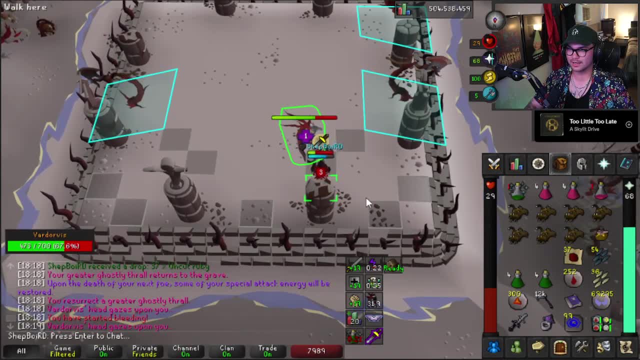 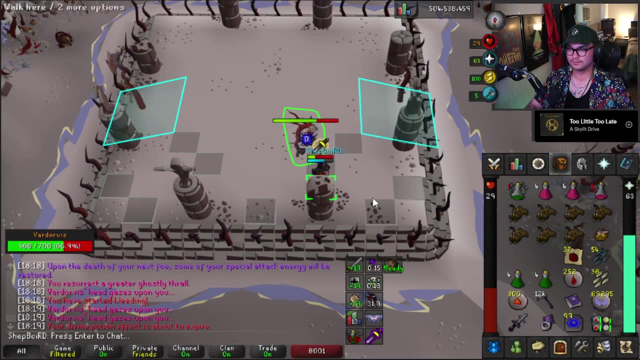 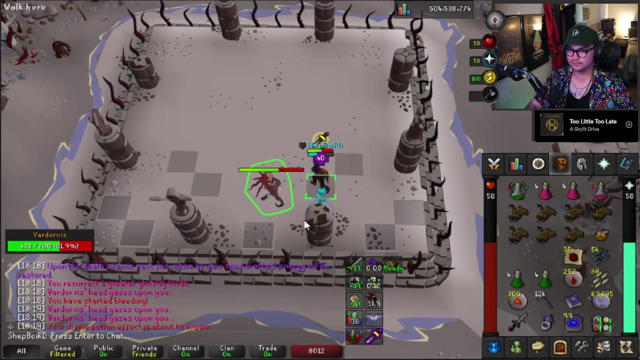 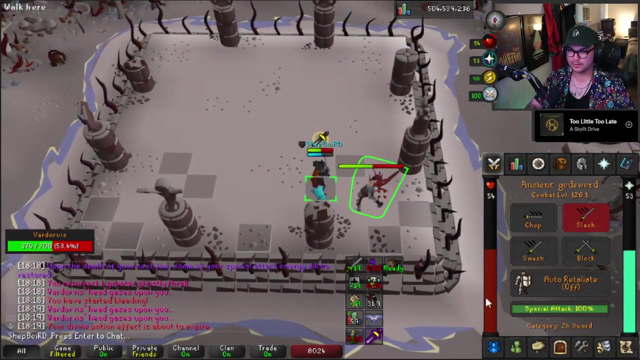 i'm not particularly good at the game either, and so you know it. probably i would be leeching a lot of lives, i think, and i think, like a zircon could be fun. the only thing i don't want to do as an iron man, though, is: 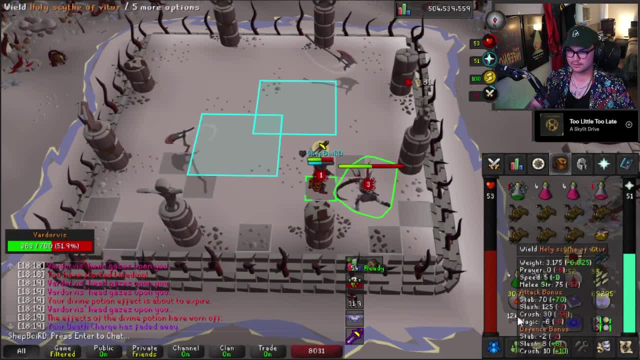 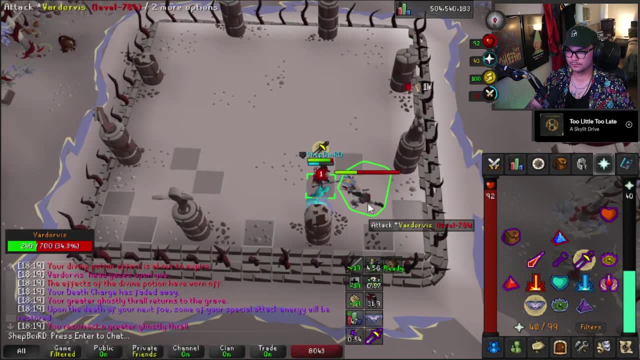 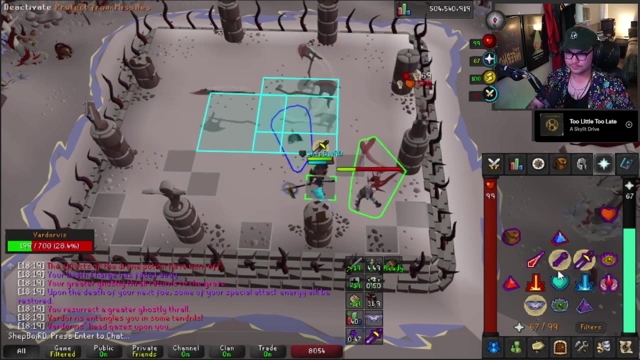 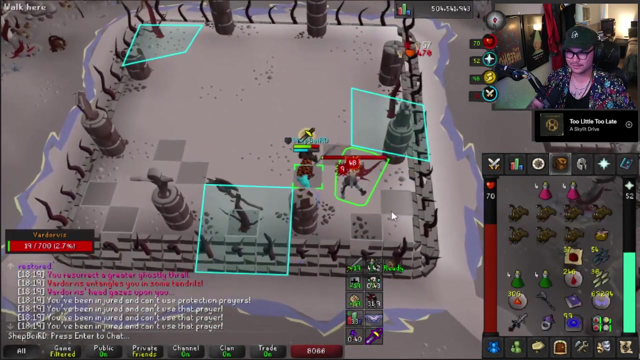 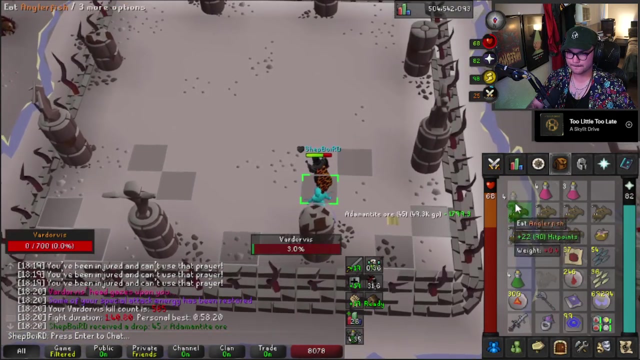 because i don't have fun with gauntlet 99 hp and working on max combat there's or on the second ult dude, the adjusting my glasses man, the adjusting my glasses man, it just does it to you. it just does it to you. at least it wasn't like. 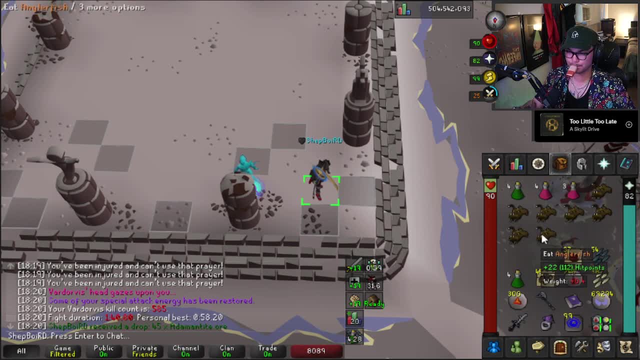 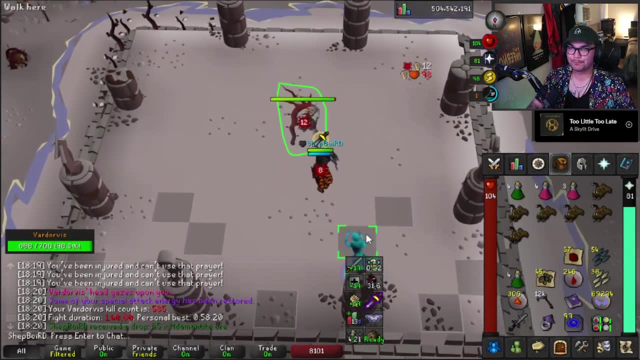 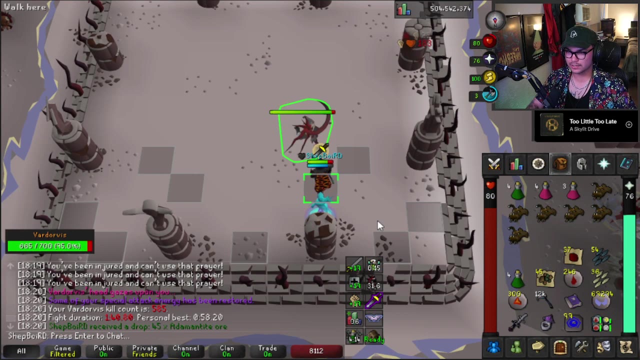 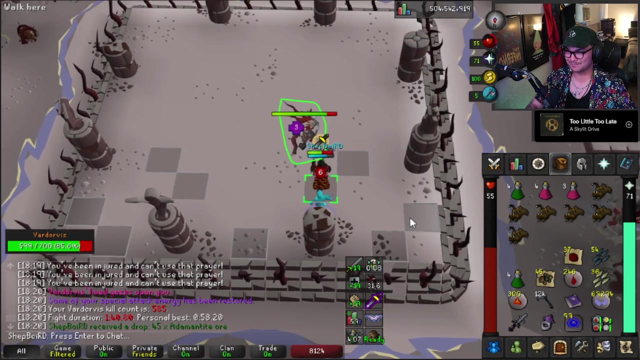 evade. that killed me. that time nightmare zone is love nightmares on his life. i definitely think, um, i think i would do a lot of stories low key, like i feel like it'd be like really good, my first hole as a faster zuck pb than a jad pb ain't no way. 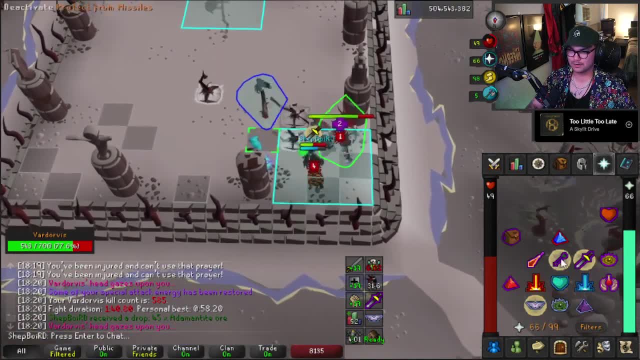 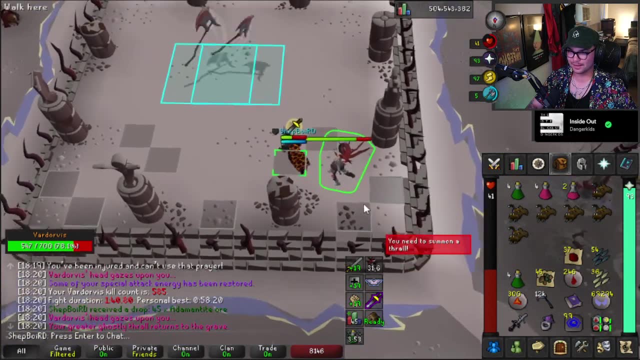 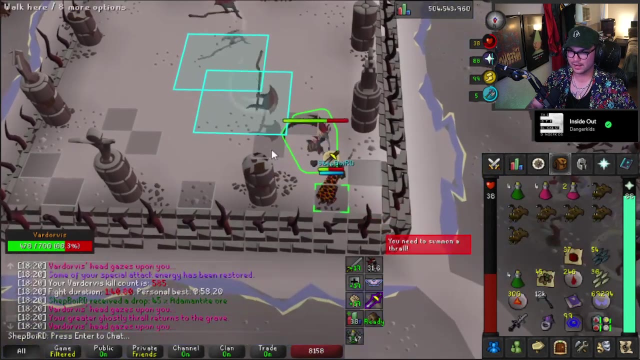 dude, my zuck pb on, uh, my ult is not not great. it is not great, i'm not gonna lie. it's like, uh, i mean my zuck pb is not great in general on this account either, uh, but i haven't got into like speed runs or anything yet. 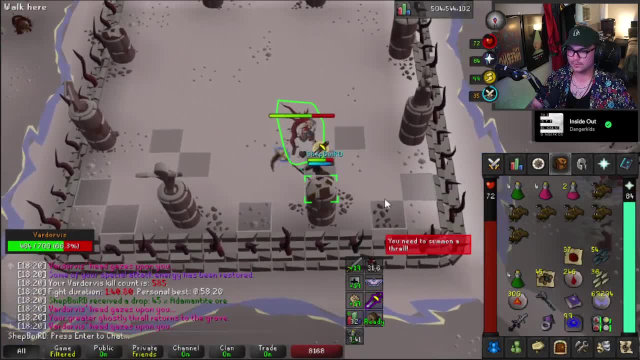 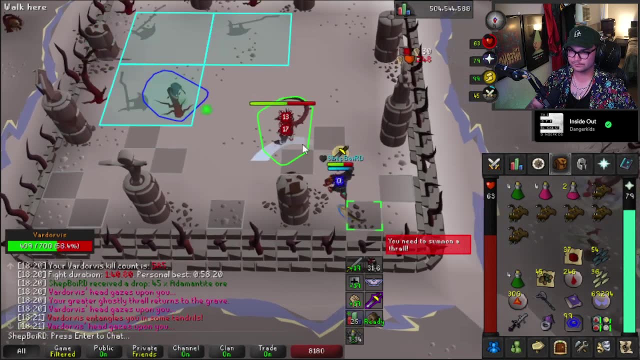 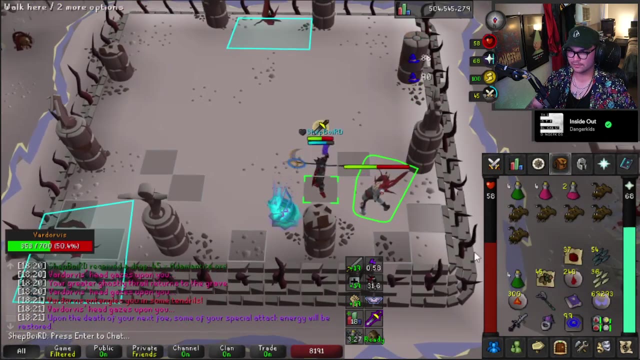 either. um, i kind of want to my next. uh, since i have the pet now, like now, i figure it's like might as well yellow, some fucking, um, what's it called? yellow, some speed runs, because, like you know, now it's like i don't really have anything to go for. 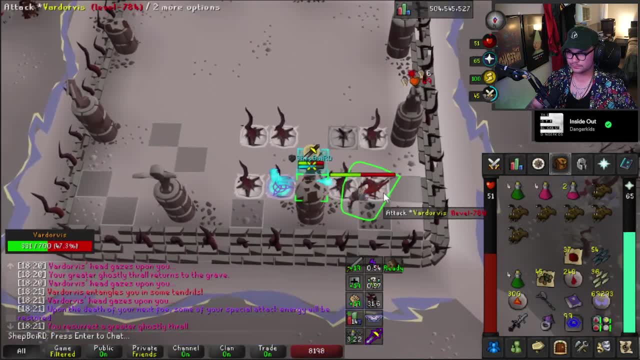 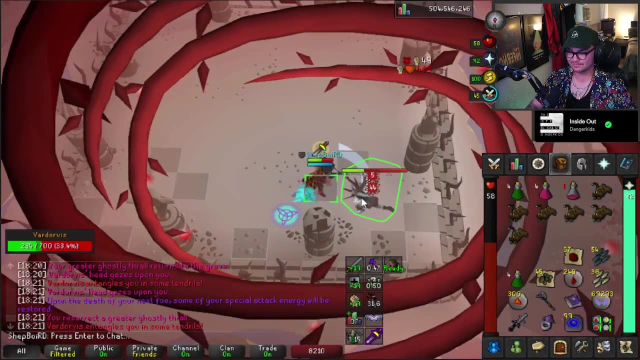 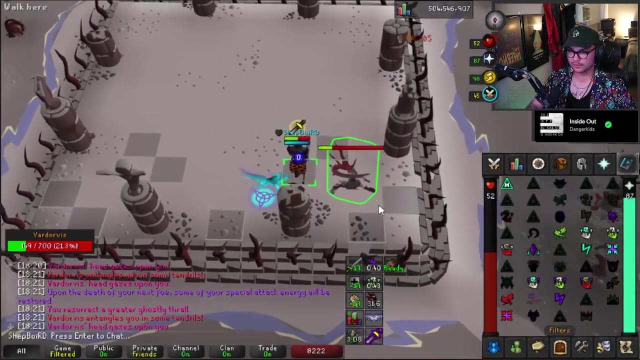 outside of combat achievements. uh, the speed run, because like i still haven't done like the jad skip, like- and that's like not supposed to be that hard, i don't know, versus like some of the other ones, i don't know. and then even dude my last triple. 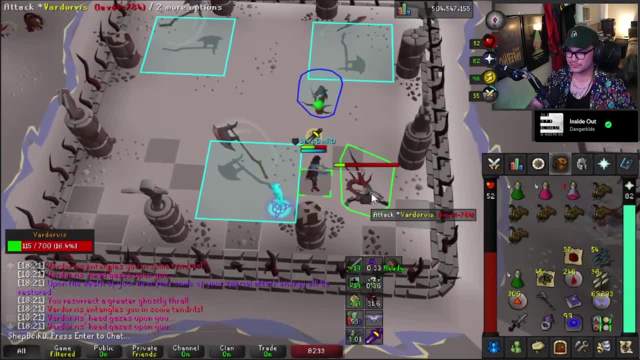 uh, the uh. one that's like the playing no shock, inspgrips and then even dude my last triples. the one that's like the playing no strike varsity. marina like hello vai, i wanna have another. damn lisa k castle with Jads. it took me a minute to kill all three Like or from when the first one died. 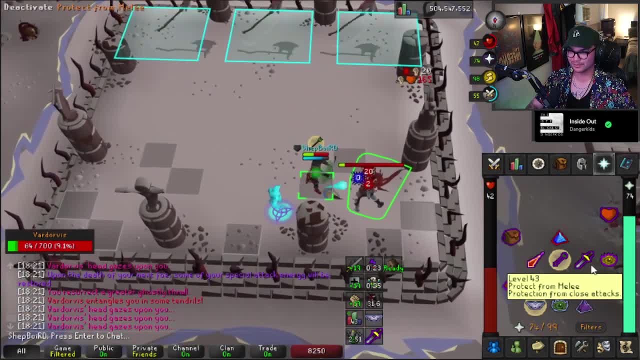 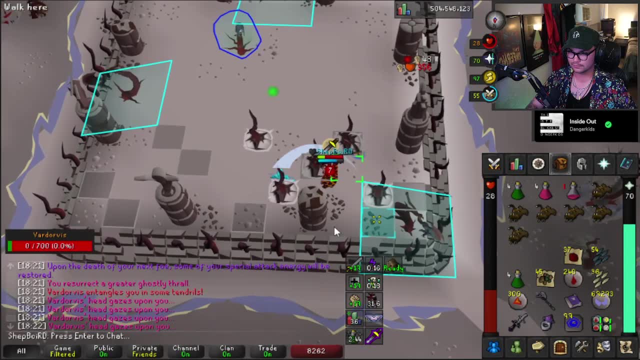 it took me a minute. A minute and 18 seconds and I remember seeing that and being like dude, I didn't even like leave him alive and like do the thing for any particular reason. They're a little hairy, I'm not gonna lie. They're at the end. 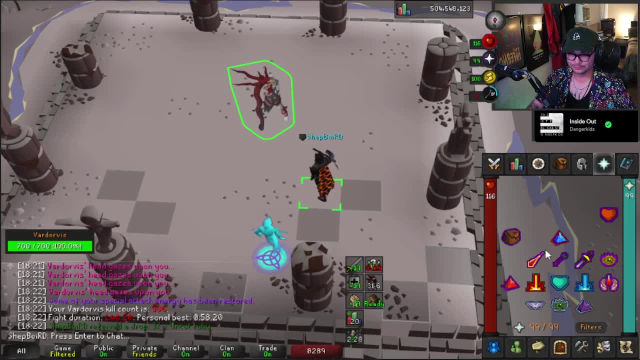 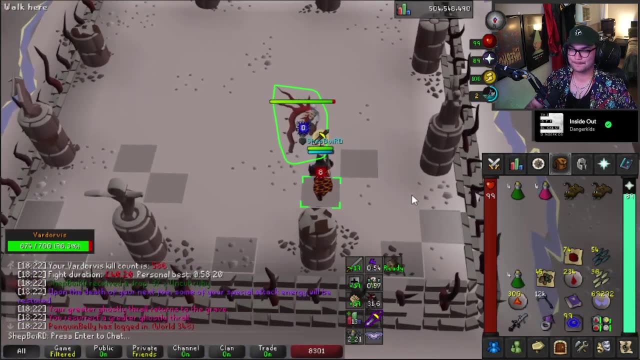 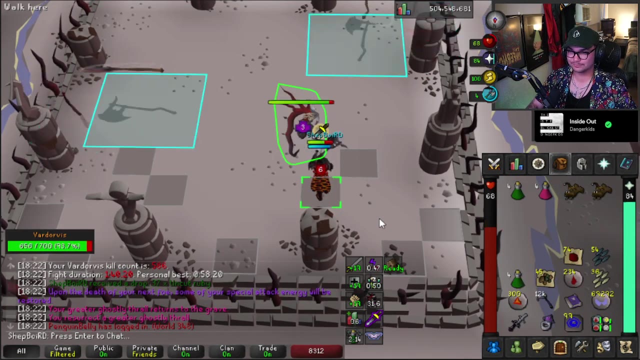 I don't want an Inferno lock. You said you would. You said you would, Although I do think Blorva, Blorva, Fire, Cape Sang Scythe would go incredibly hard. I have to, You don't have to. Nobody is telling you. you have to. 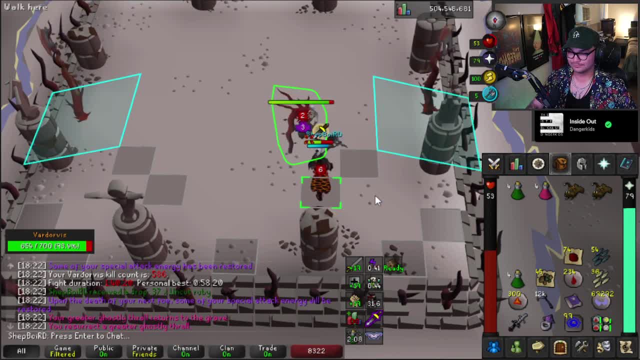 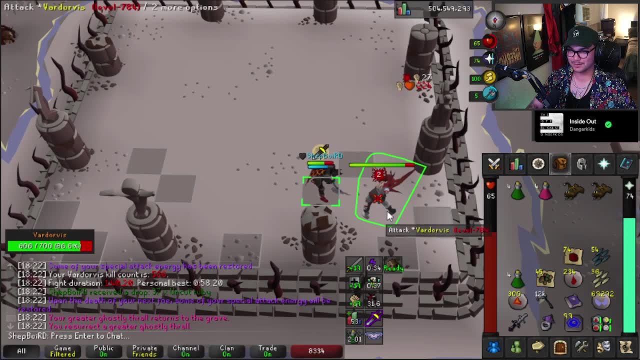 Beat the waves, so just gotta, I mean you can be a cheese caper the rest of your life. Mr NoSleeve's still a cheese caper, you know, and he plays the game I'm telling me I have to. I mean you could? you could continue to be a little piss baby. 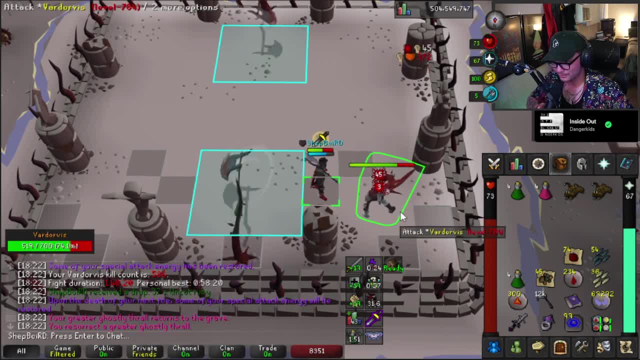 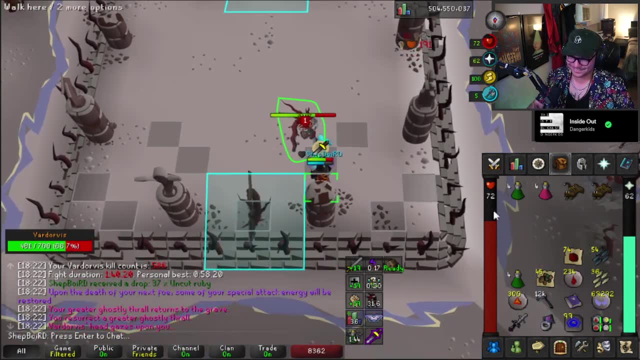 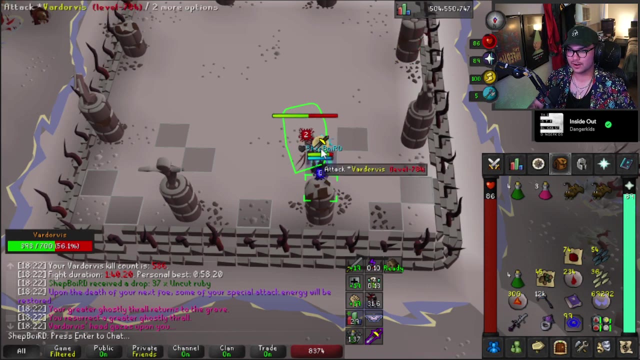 fire caper, or you could just man the fuck up and grow up and get an Inferno cape. you know, That's all I'm saying. That's all I'm saying, You know what. So yesterday too I saw, uh, I was watching Phoenix and uh, she uh Wardkitten. 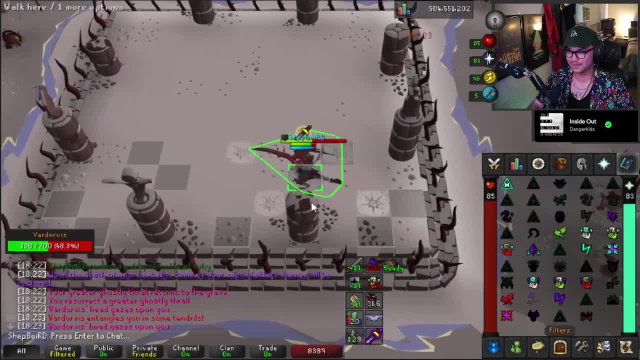 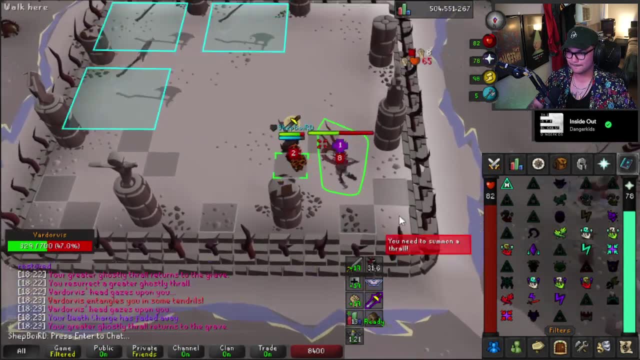 never no, and I don't really care about the OA kits. It's more of something I feel like I have to do just because, like I have Blorva, but like I don't really care If you need a heal and spec transfer, oh my god, Oh my god. 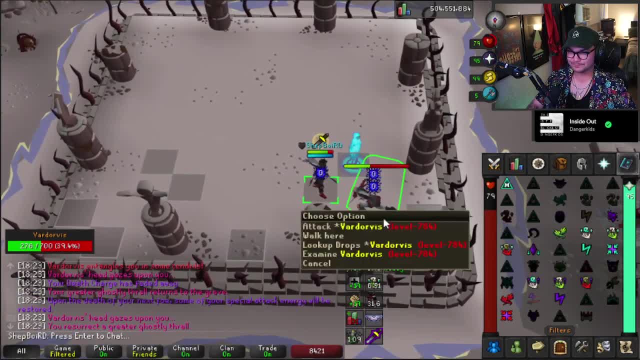 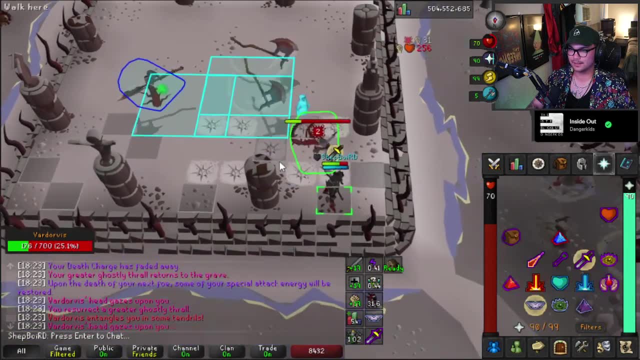 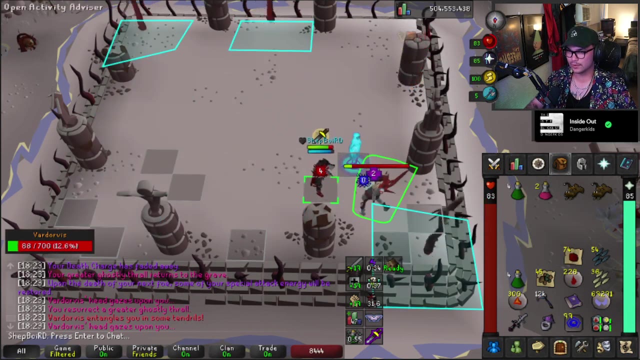 What if? what if we do that? What if we play on the ult today And like get to where we can? Bardos it right, Because, like I would like to have like a Fang like before the charity stream, um, because I was like I'm gonna do like giveaways and stuff. 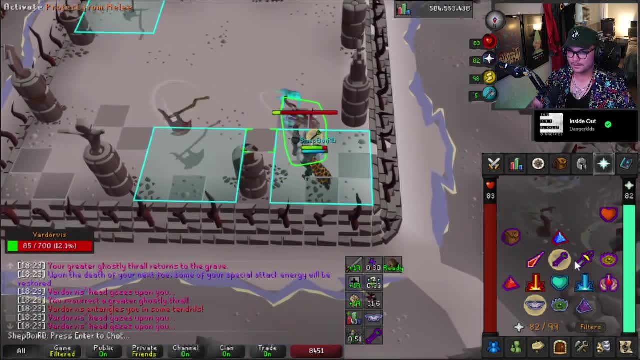 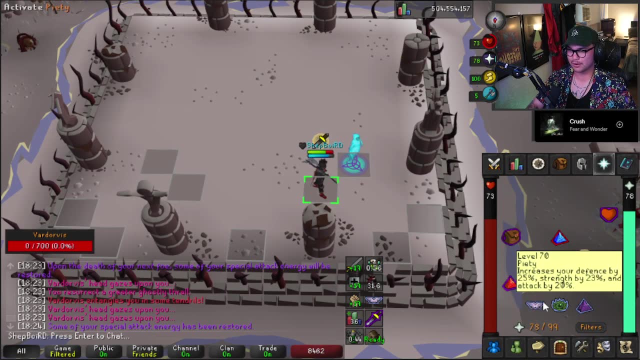 so I was like saving money: Um, takes forever to get the RC level requirements. Yeah, I don't. I don't know what my RC is. Step row RD though, Just like, uh, here I'll log in and then you. 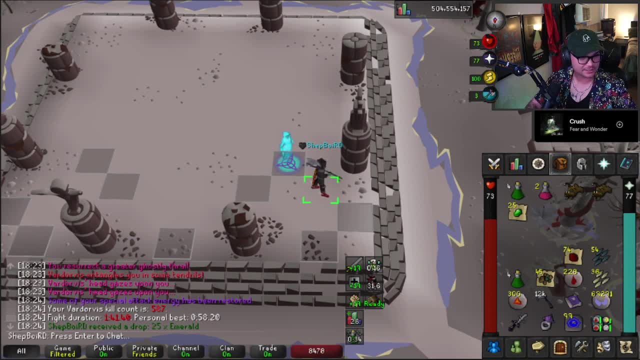 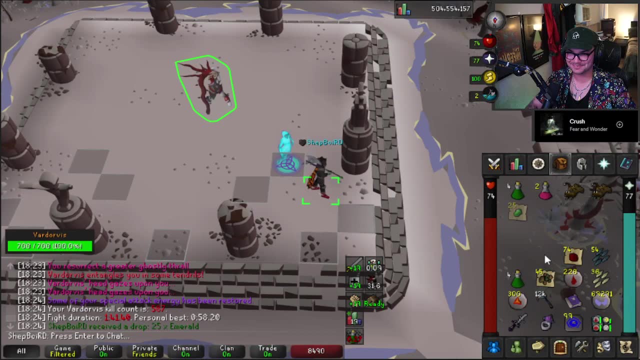 guys can see it. Hang on, Although, shit, I don't have a scene, dude, I don't have a scene anymore because I had to reinstall Windows. That makes me sad. That makes me sad. Uh, I mean, I'll take, I'll take spec, I'll take spec. 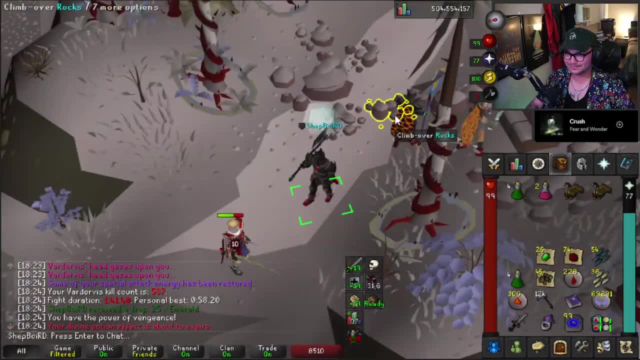 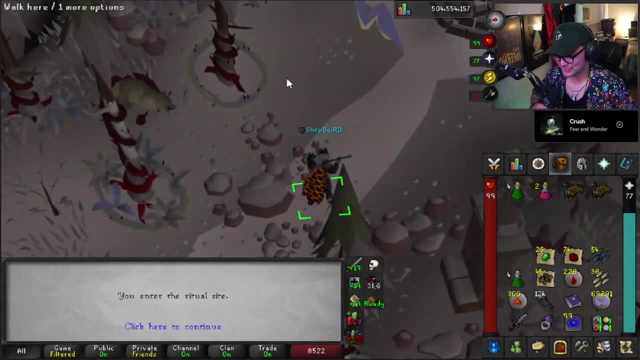 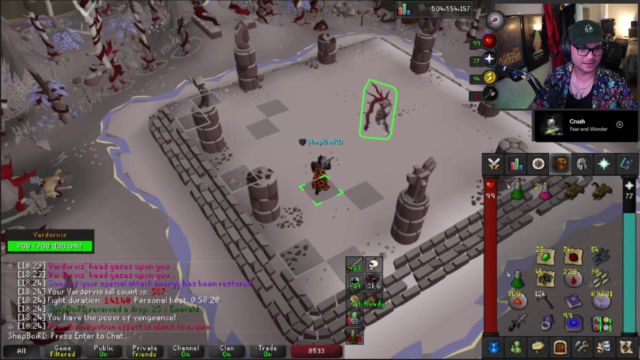 Oh my god, Oh my god, See why? Fucking gamer, Fucking gamer. Thank you, Churchy, I love you. Let's see Here, I'm gonna do this real quick. Give me like two seconds, I'm gonna. I'm a cook, I'm a cook. 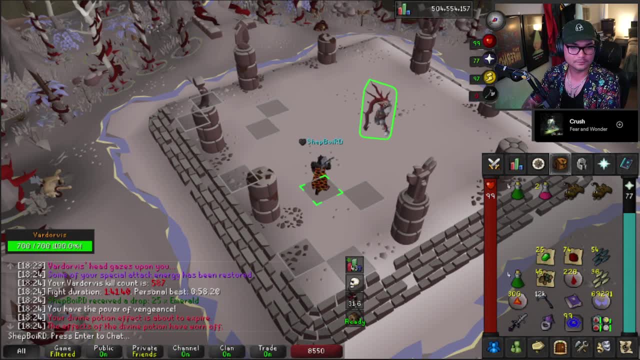 Uh, Fuck, dude, I don't have. I had that going for the Bard pet and it was sick as fuck. Yeah, dude, I love alting. honestly, I don't have membership on the alt right now. Uh, let's see Alt. 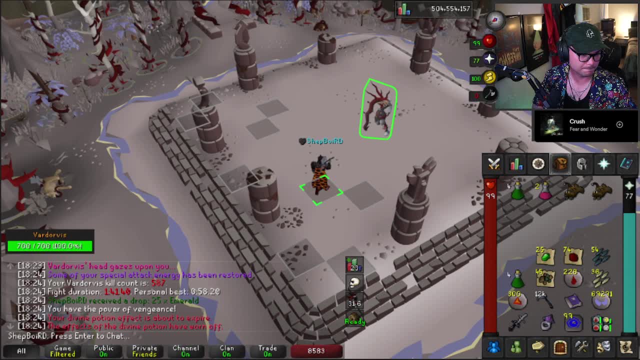 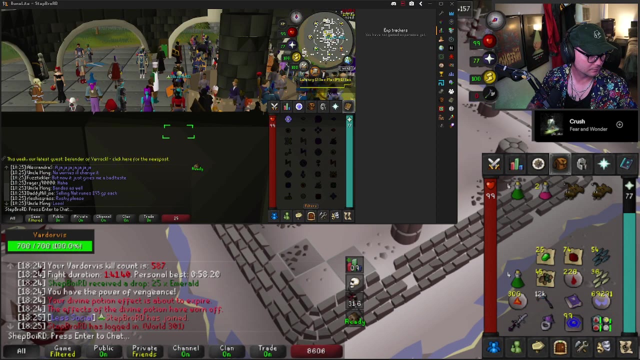 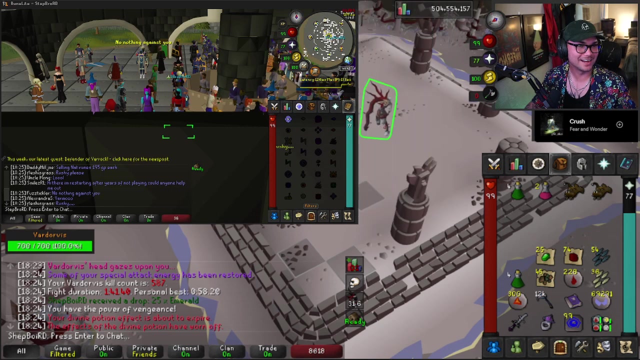 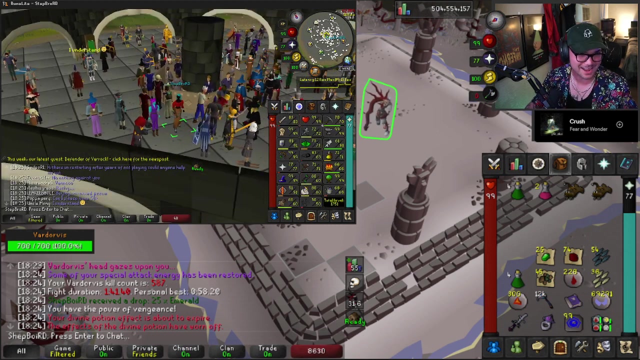 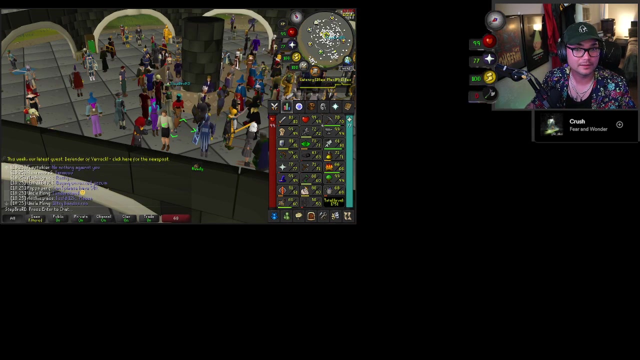 Pain, Let's Window Bam Fuck. Give me one second. Give me one second. I gotta, I gotta cook. While while I'm getting this together, here's the the stats. right, Let's see. Delete That. We'll put that. We'll do this. 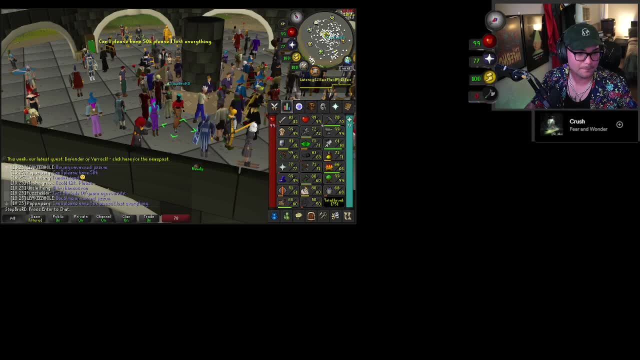 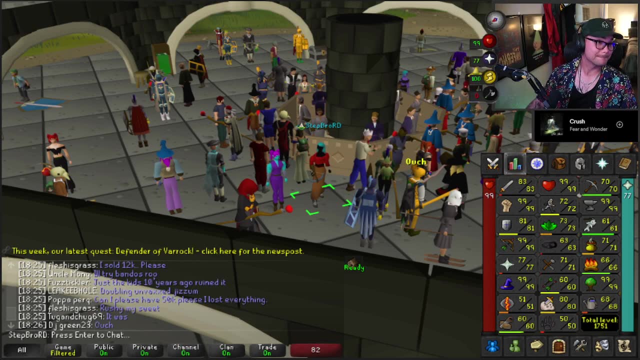 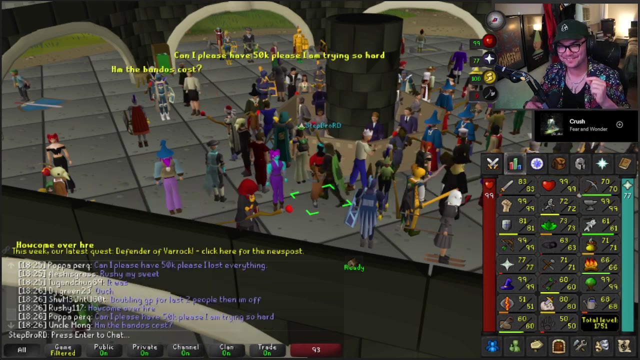 This Transform And then we gotta move that down Alt scene setup. Dude I am, I am getting so good, I'm getting so good with OBS and you guys have no idea how happy that fucking makes me. How happy it makes me. 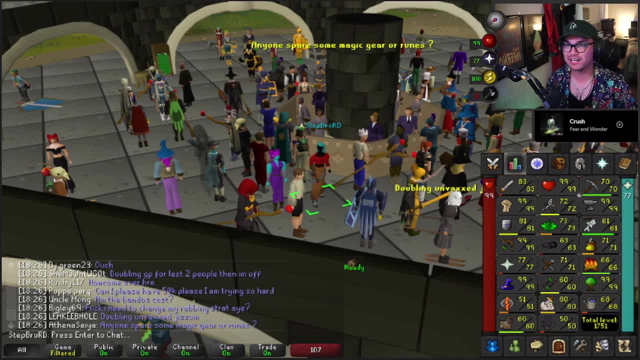 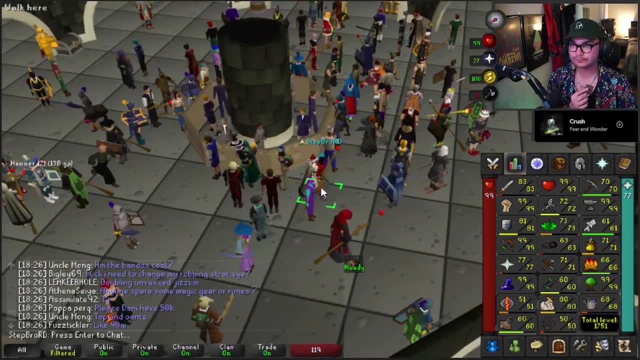 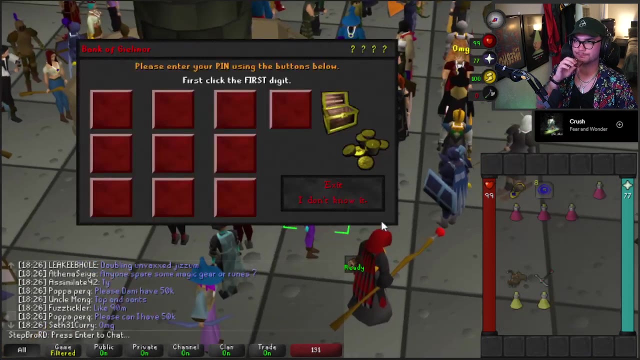 Although the uh orbs aren't right, so But that's okay. But yeah, check that out. You see the rune crossbow, Uh, stats quests. I'm at 233.. Because it's just a rune dragon ult right now. 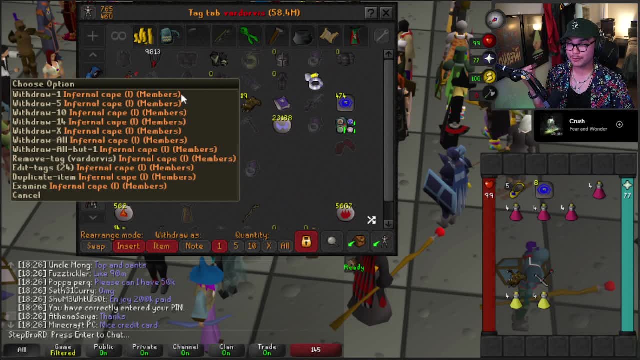 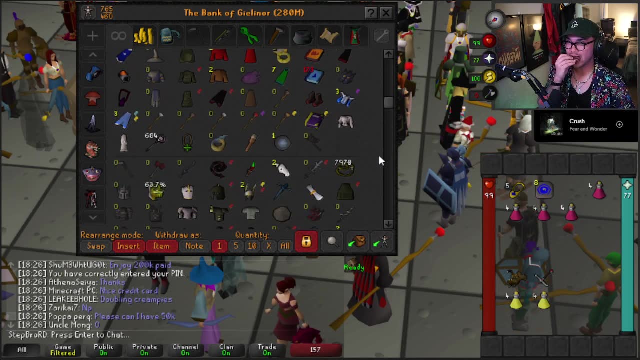 Inferno cap, Inferno cap, Pretty good. Um, I'm on the rune crossbow. I am only about 20.. Um, I'm very lucky. I'm going to take this time. Here we go. I'm going to take this time. 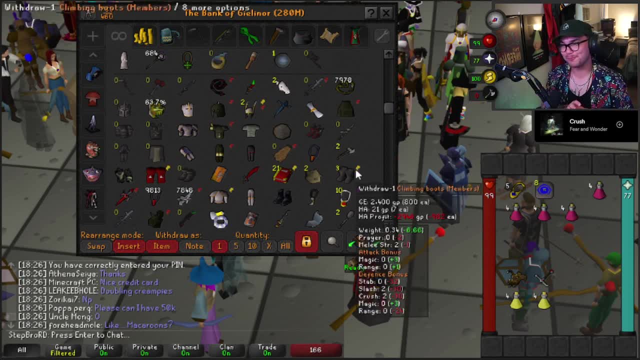 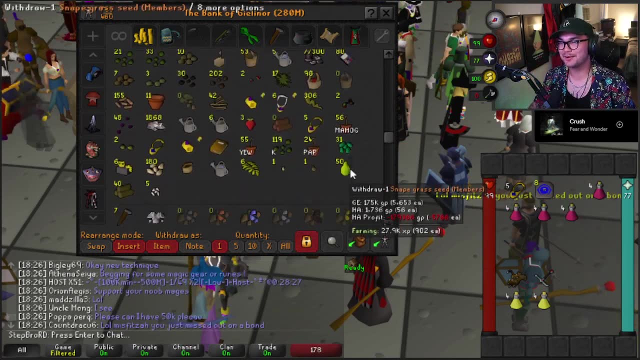 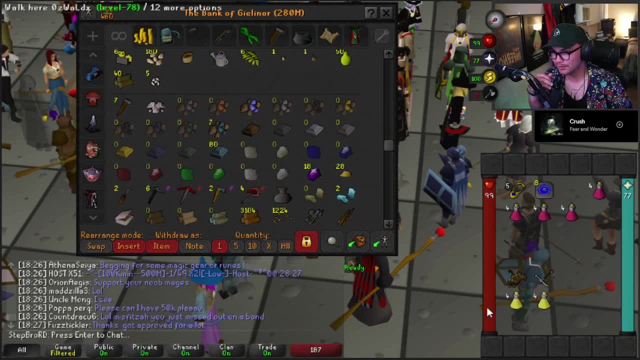 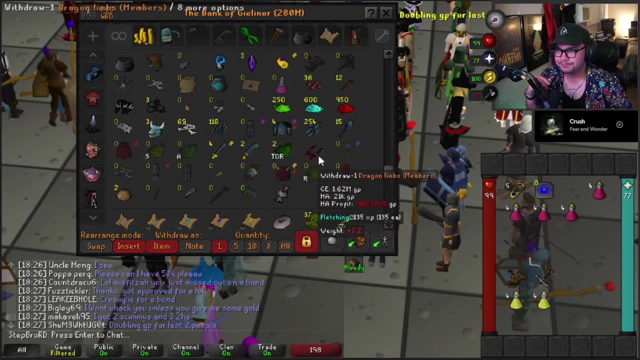 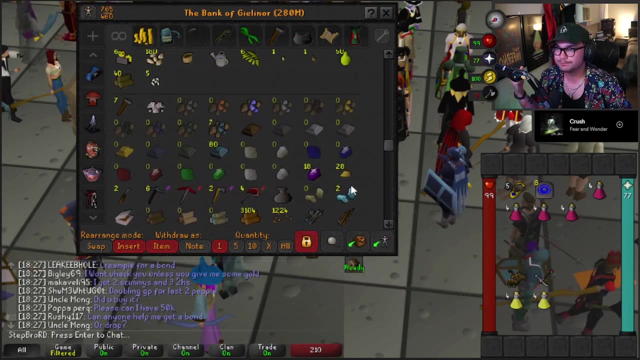 I'm not going to lie, I'm only missing Levi on the old dude. That's kind of huge. It's kind of huge. um, I might be able to. I mean I'll do it later- but I think I have enough money to. I mean, I have 280 mil on the account, which I think to be fair. 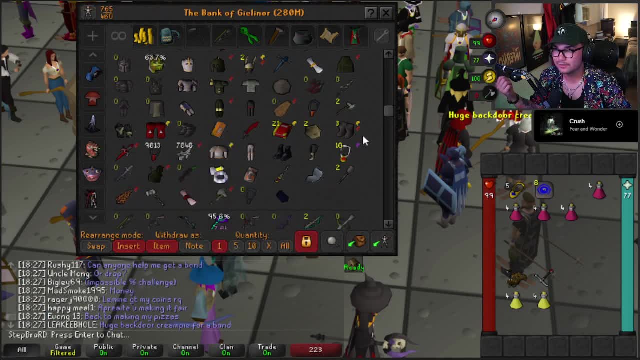 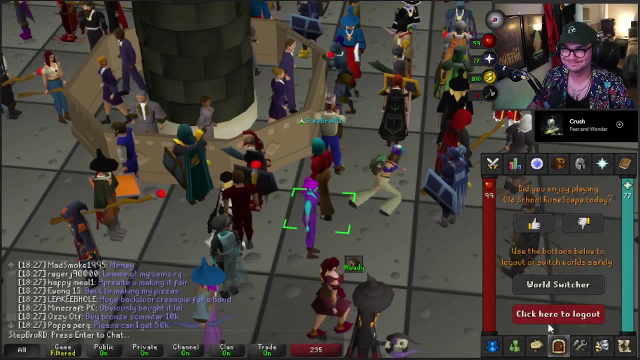 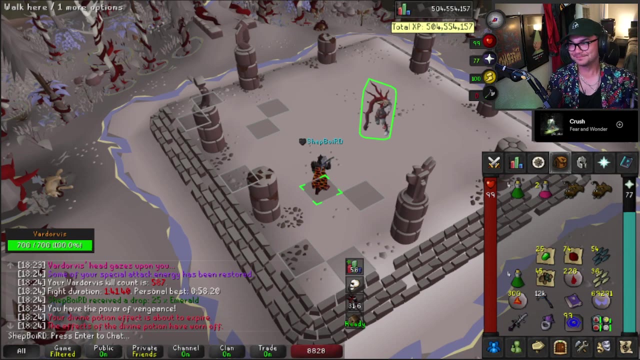 Jesse's like kind of high right now too. I have all my zenites over here too, so it's just like I don't know. I'm like getting the feeling of coming in the gym. I'm getting the feeling of coming at home. I'm getting the feeling of coming backstage when I pump up, when I pose out in front. 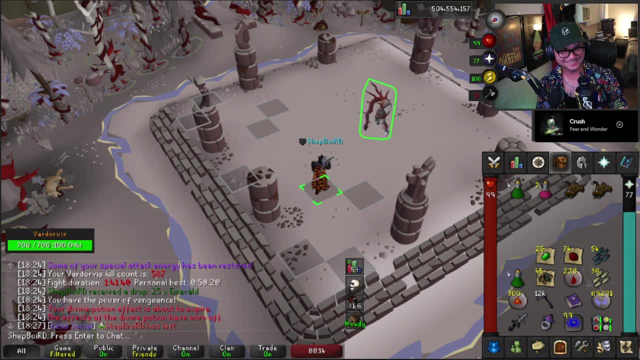 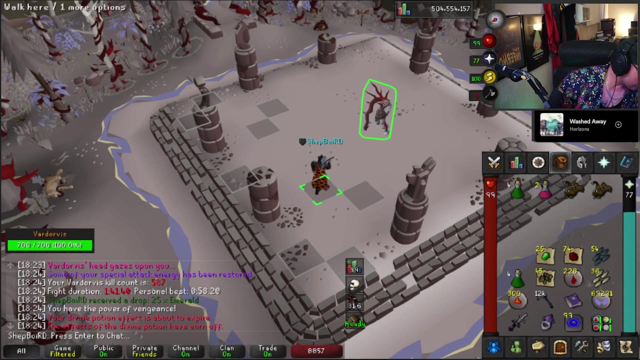 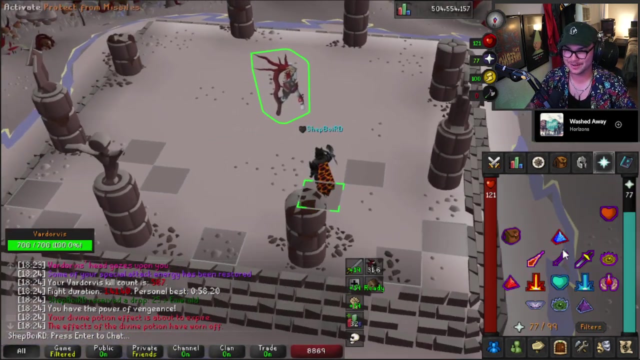 of 5,000 people. I get the same feeling, so I'm coming day and night. I mean it's terrific, right? Halute loves to come. he comes so much, dude. he comes so much and I love that you love to come. I got a question for you guys. if I were to sell out, always come first. 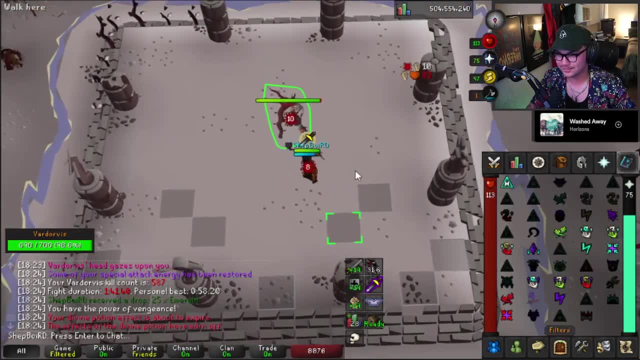 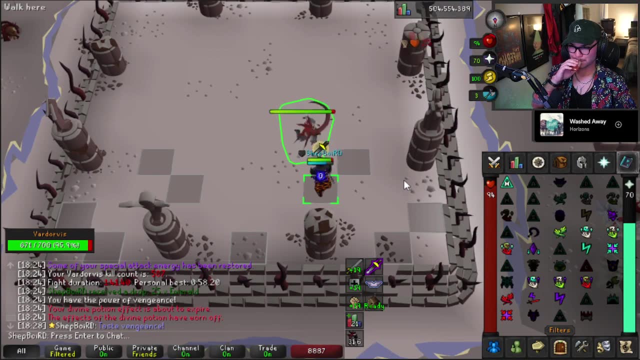 you would be the first one to come right. you would be the first one to come right. huge, huge. if I were to sell out and take a sponsorship, what would you guys think of me? what would you guys think of me? oh, my god, you benched me, dude, do it. what the fuck. 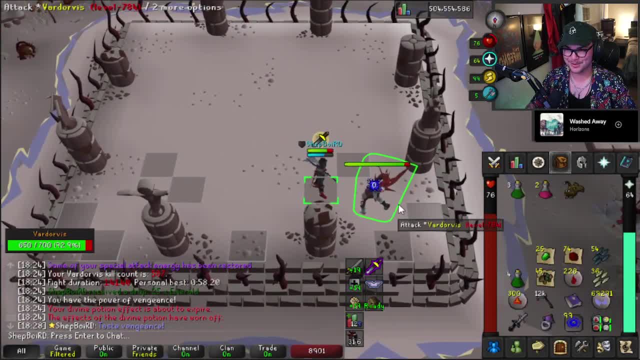 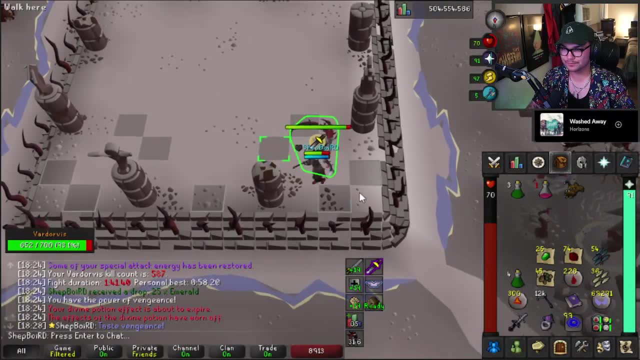 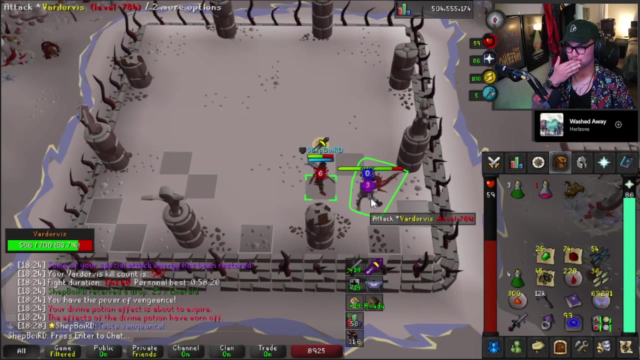 maybe you'll pay us unsub, unfollow. what if I started streaming on kick? because, uh, that is something I have set up. I just haven't done? is, uh depends on the sponsor. um, I wouldn't do a mobile game. I would not do a mobile game and. 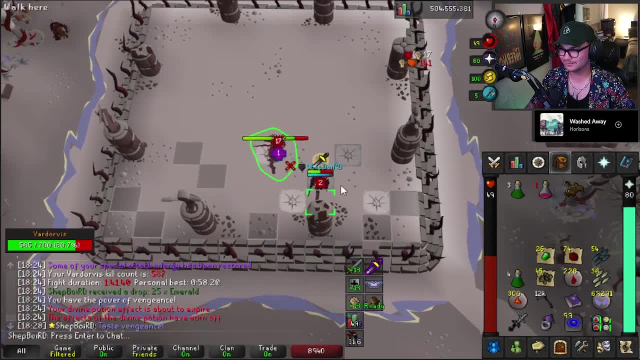 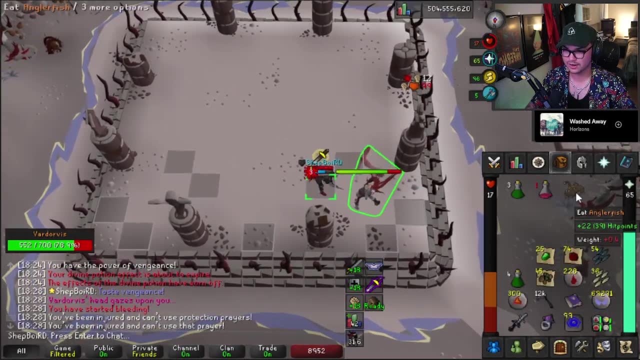 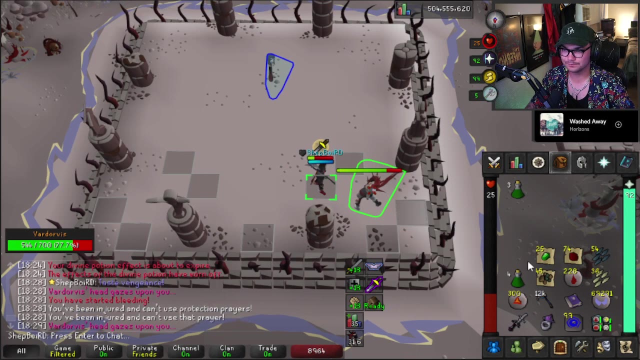 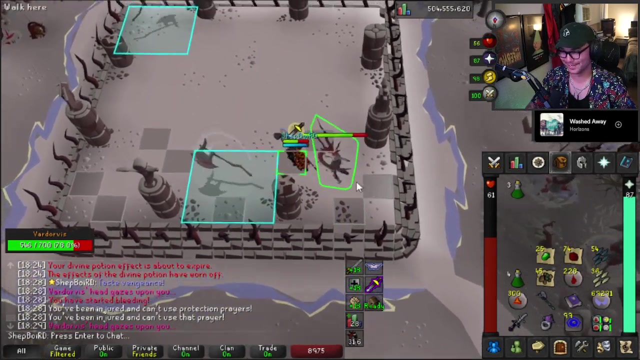 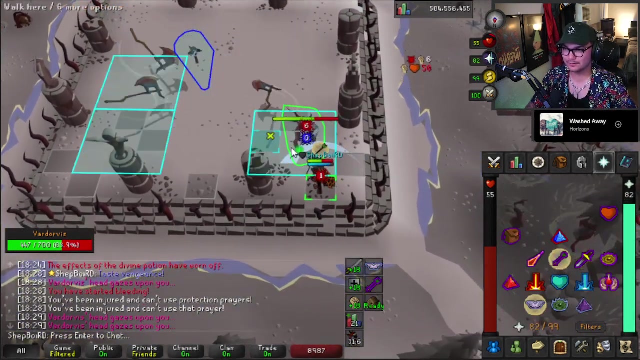 it'd probably be a food service that everybody does. kicks lame, I might die, Jesus Christ. that's what I get for reading chat. no, it would not be kick, though it would not be kick chance. yeah, oh yeah, I was reading too much, but I don't know I right now I just feel like like like I feel like I'm too small. 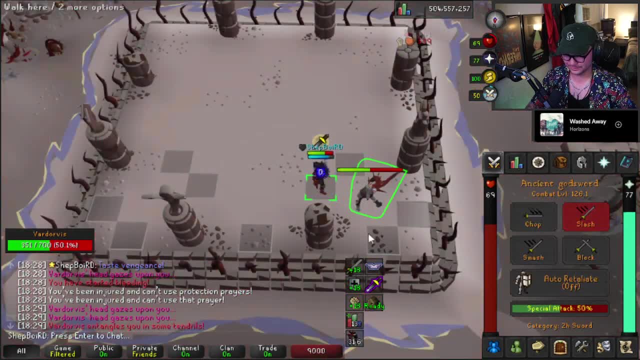 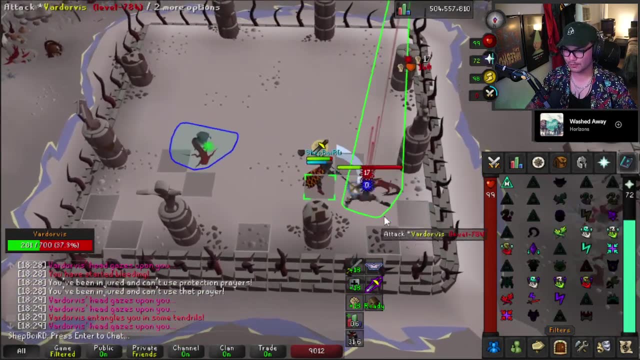 to like get a sponsorship, you know, and I feel like it'd be kind of shitty for me to take one, I don't know. that's why I haven't taken them yet. um, because I've seen the offers, like already, and I don't know. I don't know if I'm gonna be able to get them in the future, but I don't know. 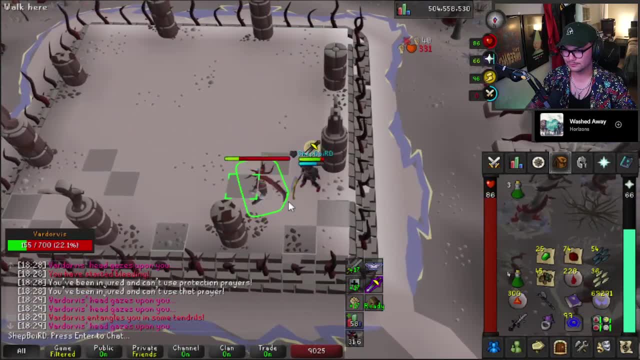 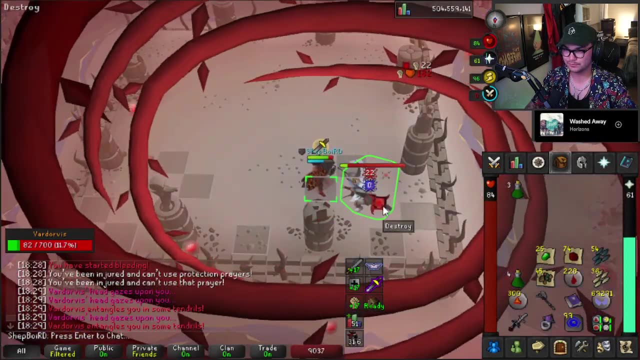 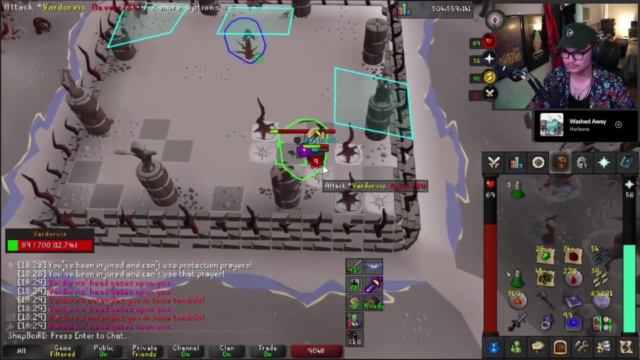 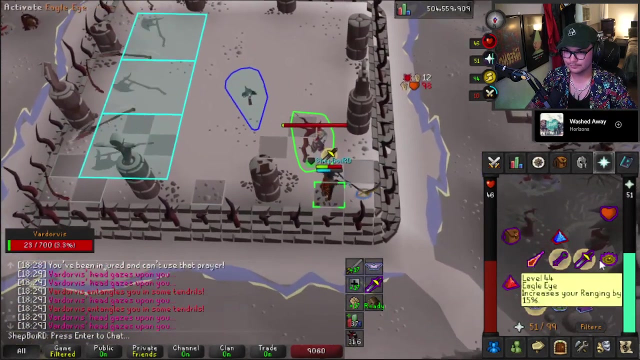 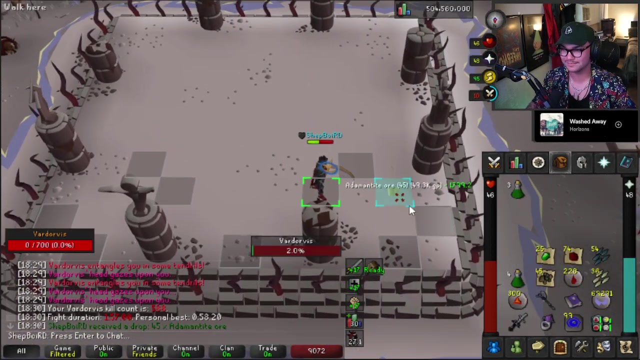 but I nearly have a white stack of all runes. that's huge. that's huge, dude. I tell you what I'm clicking. I am clicking ow. that means this one's a drop right, since this one was scuffed. scuffed equals stuff. scuffed did not equal stuff. 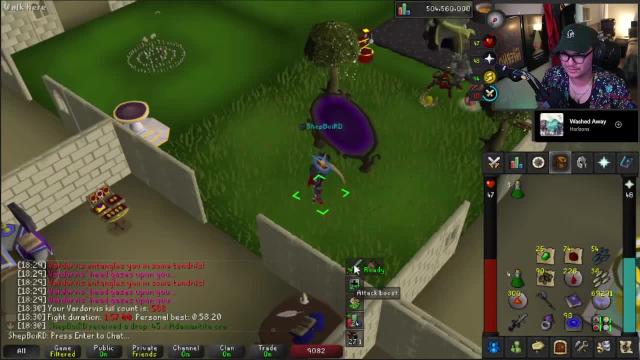 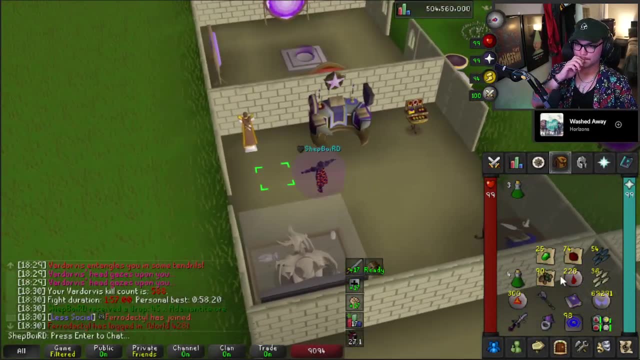 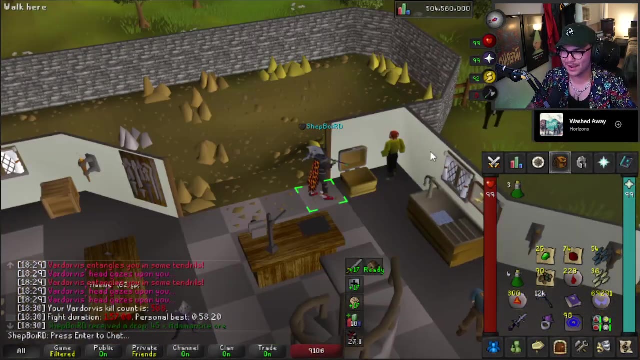 that makes me sad. dude, that was a long ass trip too, a 13 kill bard trip. I feel like that's pretty fucking long. I feel like that's pretty fucking long would I have to? so, if I do make a GIM, would I have to do a? 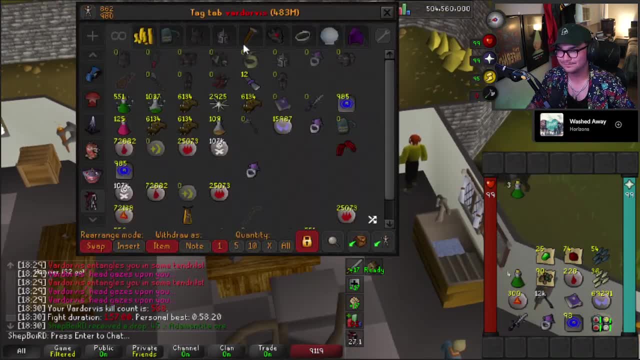 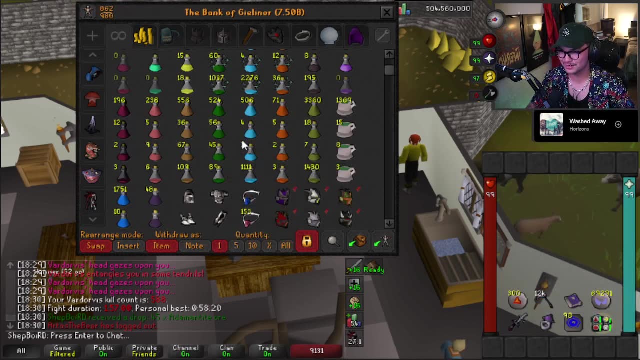 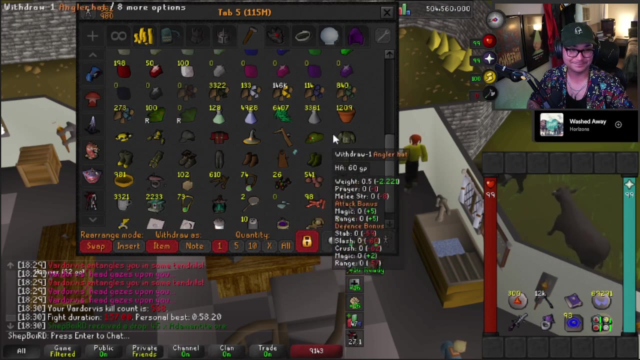 like HCGIM name. would I have to do that? would you guys like judge me if I did that? what's our thoughts? what's our thoughts? oh yeah, here's something huge for the account. you guys never would have guessed it. you guys have no idea how long that took me to. 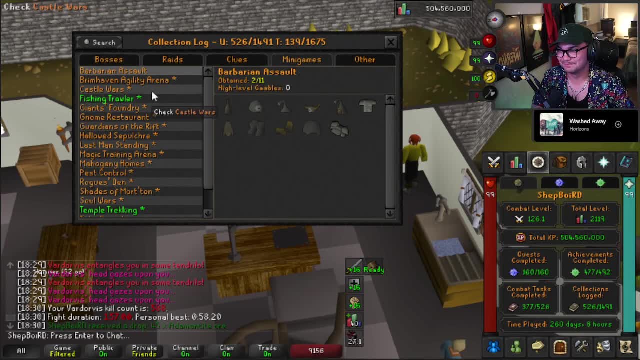 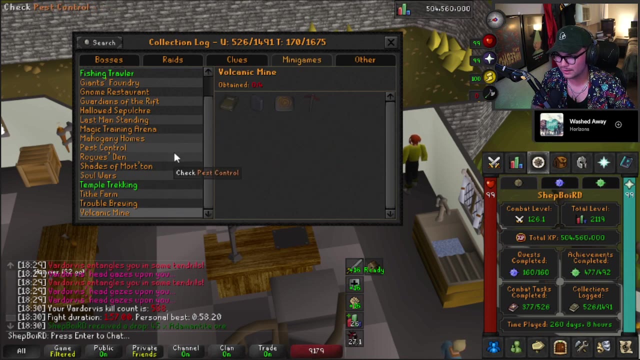 but you're about to. actually I need to update all this, all this shit anyways. so, like, give me a second. we gotta go click through, gotta go click through, we're clicking through, we're clicking through. what's the thing called dude? I forgot fishing trawler. 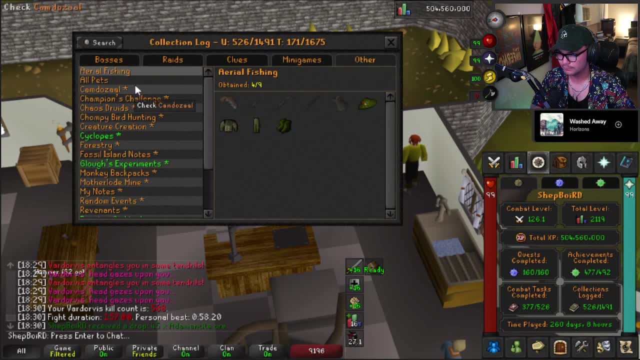 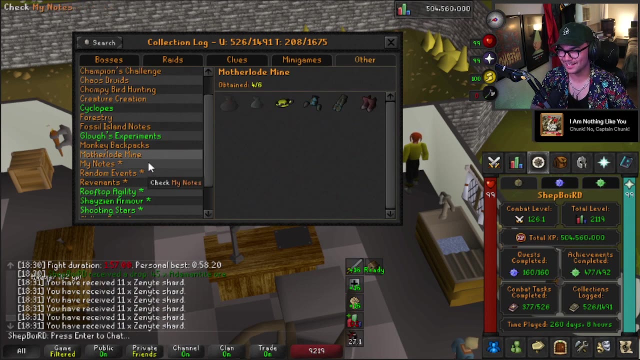 that's what it's called. is it not a minigame? is it not a? it is a collection log. where the fuck is it? oh, also, here's something like disgusting, disgusting, disgusting, disgusting. by the way, I made a lot of my like early money there too. 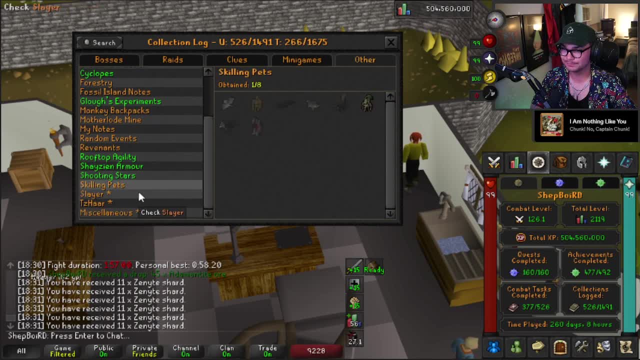 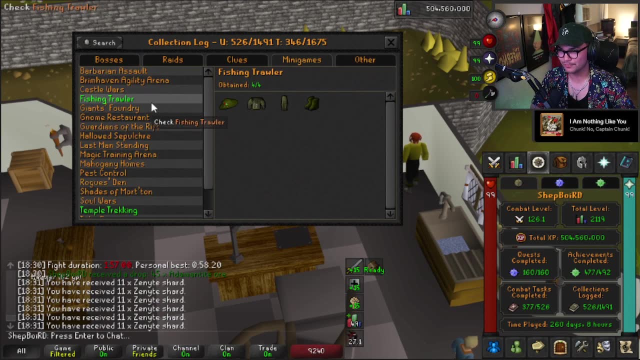 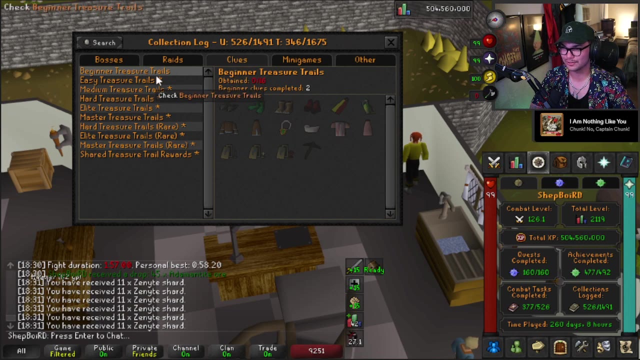 I made a lot of my early money there under minigames. oh, I'm dumb as fuck. oh, it doesn't tell you you're KC. damn it, dude. uh, it took me 29, took me 29. we got spooned on it, so that was good. 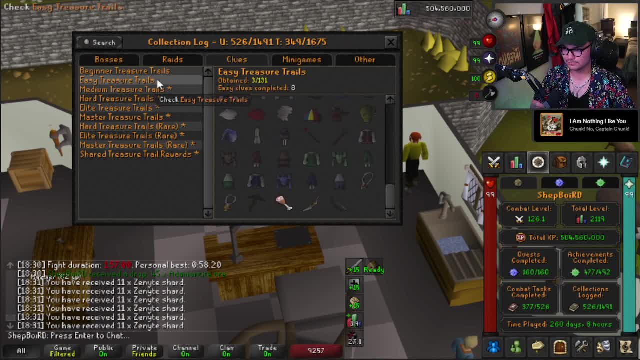 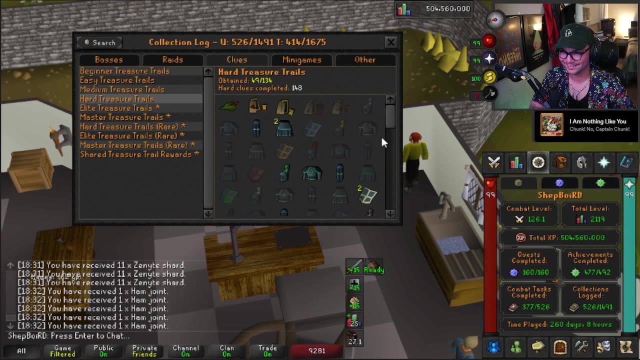 that was good, that made me happy. do I have to like: wait, I have a ham joint? wait, I never knew, I didn't know I had a ham joint in my fucking collection log. when the fuck did I get that like? I don't remember getting that like. 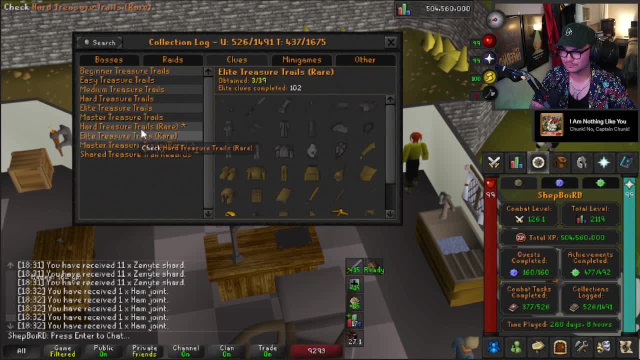 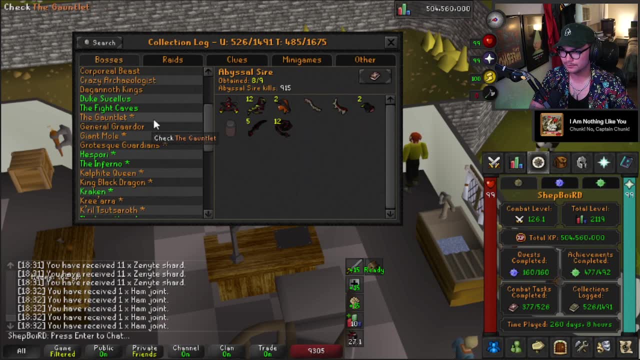 I don't think I actually have to like go through this right or like scroll down. I'm just trying to sync the plug in real quick. um, just because, like I see all the asterisks, here's, uh, another thing that's a not super disgusting, but but a little. 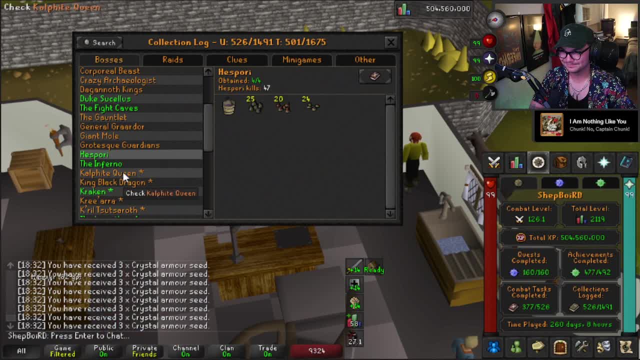 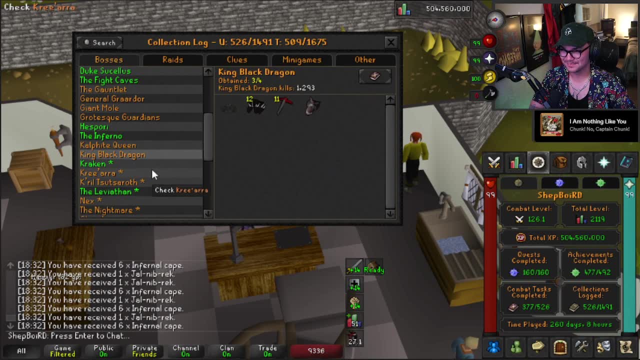 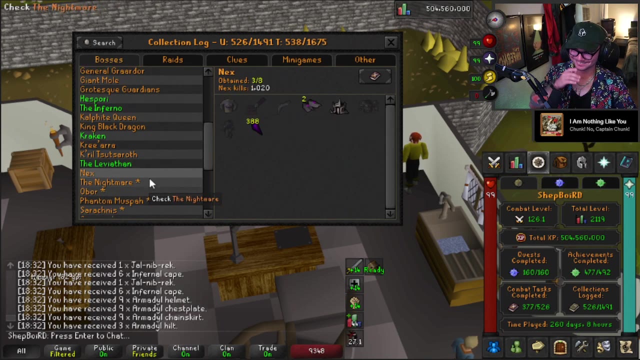 oh, this is. this is disgusting. I'm sorry, churchy, I apologize for that. that was rude of me. this one's also gross, dude. look at all this shit. put that shit away. what do you mean? I don't know what you're talking about. I don't know what you're talking about. 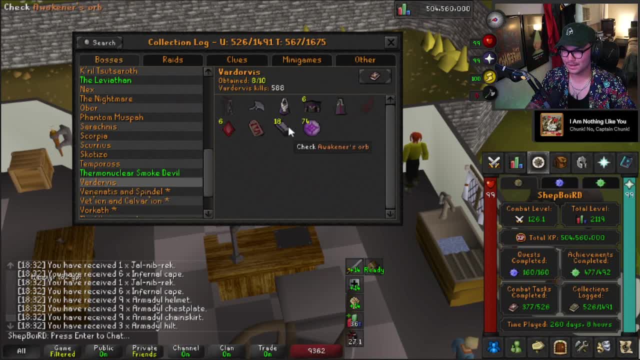 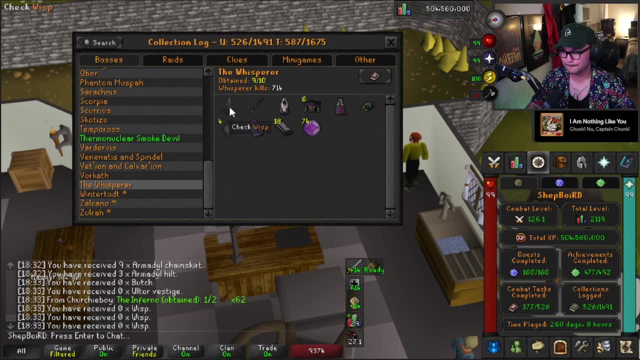 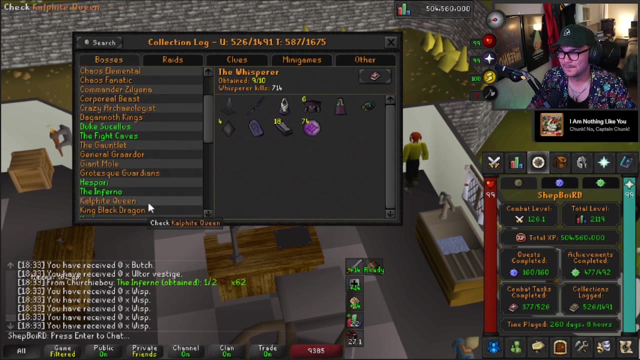 yeah, once I get pet and ult or bard as greenlaw, I don't know what you're talking about. yeah, atleast he's green logged as well. whisper is almost green logged. I'm sorry, churchy, sorry, uh, let's see. bam, bam, bam uh. combat tasks too. 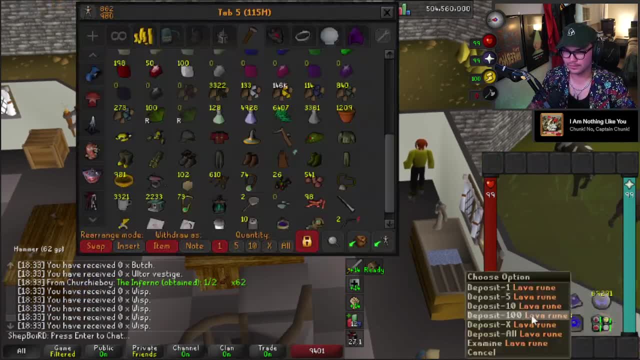 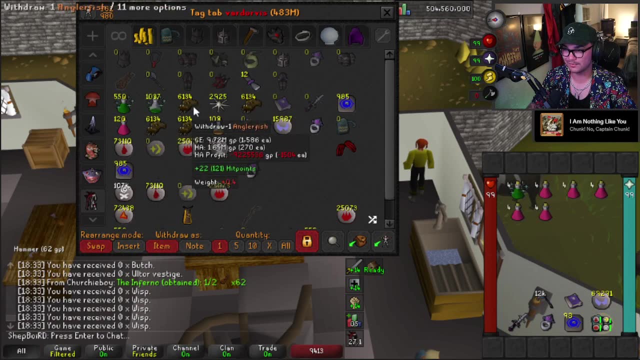 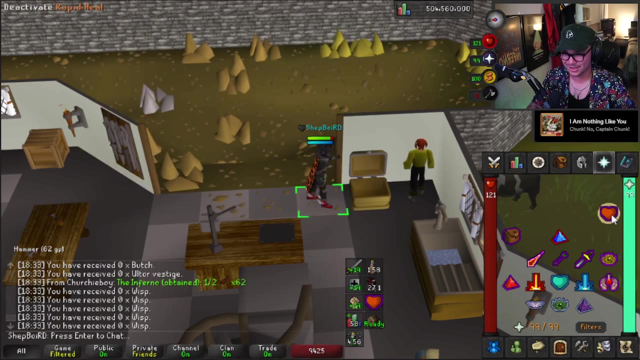 we're at 152, 152. I have like all the duke ones I still need to do too, and I just, I don't know, I haven't like been super motivated to do combat tasks. um, I really, like I don't know, play runescape lately because, uh, hell, divers came out. i've been playing a lot of that. i've been 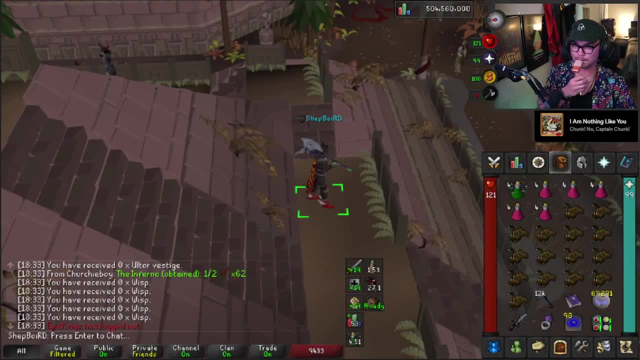 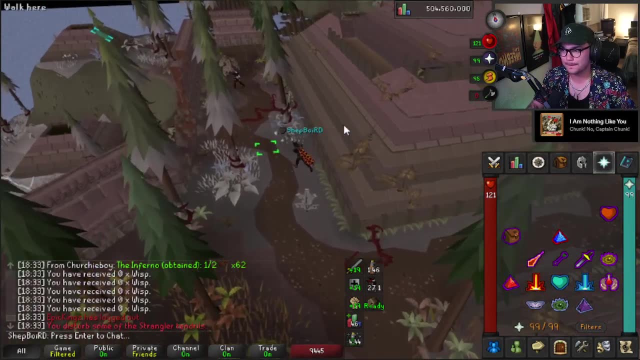 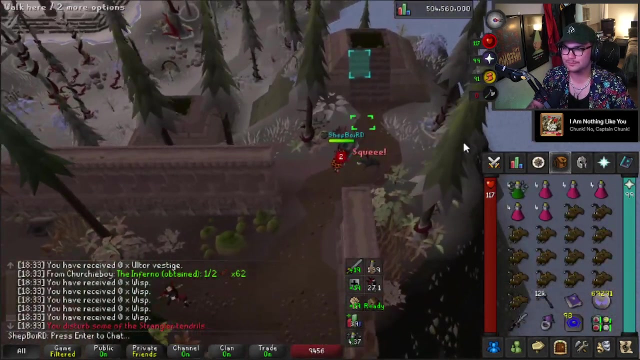 playing a lot of that. i've been playing a lot of runescape too, though it's just like i don't know. i'll like come on and then i'll just like, you know, just uh, do the whole, do some var trips, do some hard mode top, and that's like really it like i haven't. i haven't really done a whole lot. 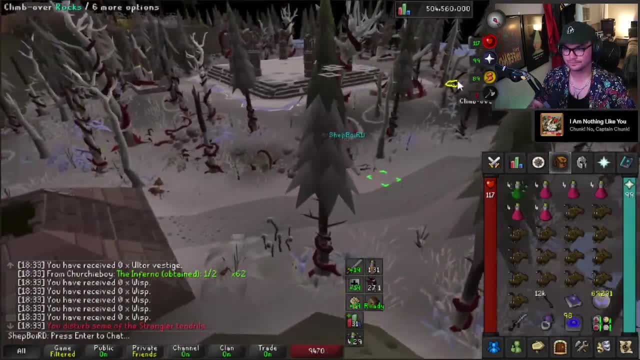 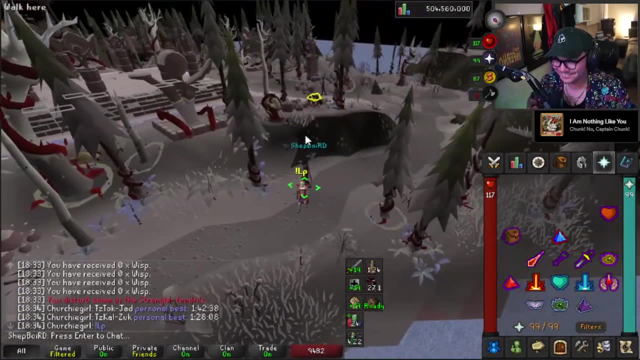 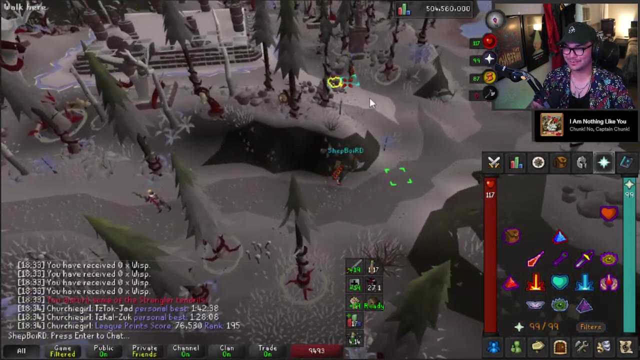 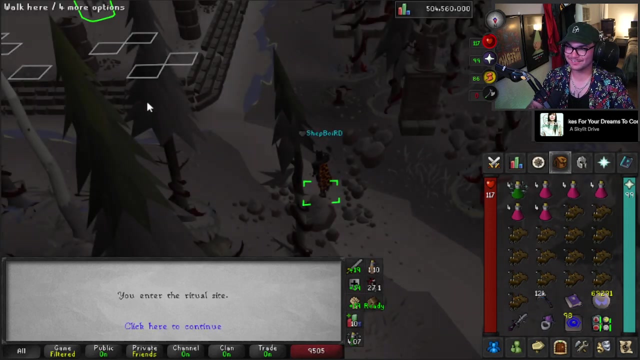 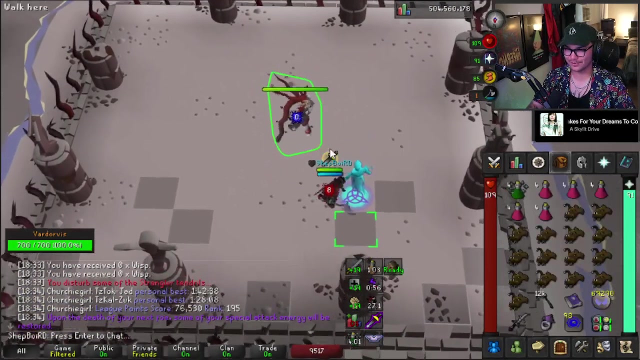 pbjad- what the fuck is that dude? huh huh, 76k league points- though that's kind of nuts, kind of nutty dude. i want my blood scythe. i really do. i need a blood scythe in my life. okay, i did my zog with 85 range dude. like that's fucking great. i mean, i guess like with a tivo. 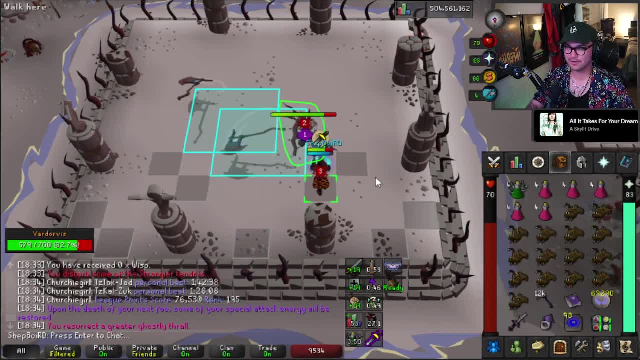 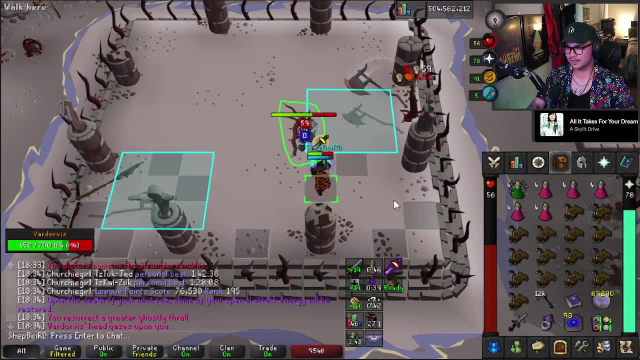 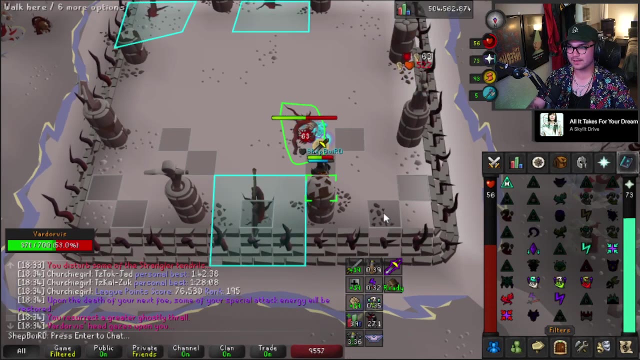 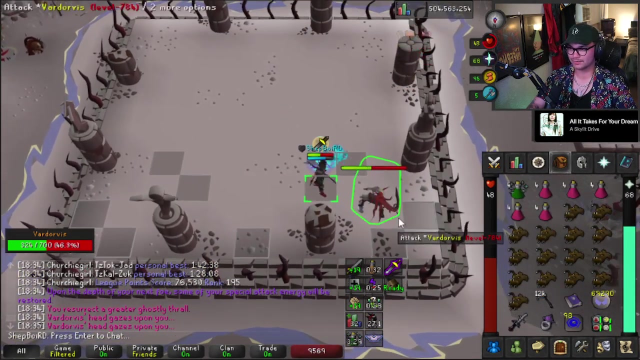 like, how much in those 14 range levels? how much does your dps? i would assume a lot like i would assume anyway, i don't know. oh, here's some uh good news. uh, i want a base hat on their uh, uh, what's it? they're 200 patreon special. pretty large difference, especially off task. yeah, i bet. 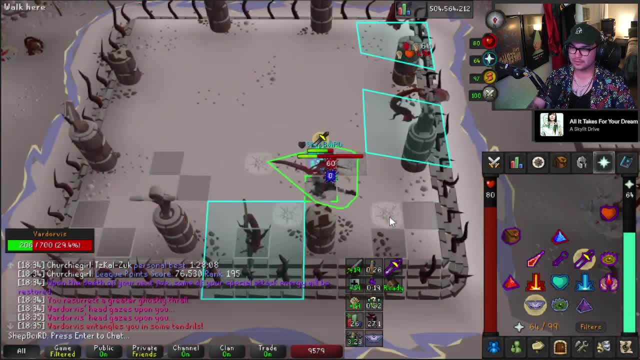 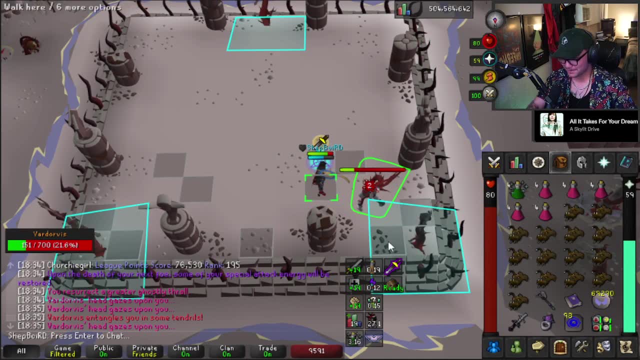 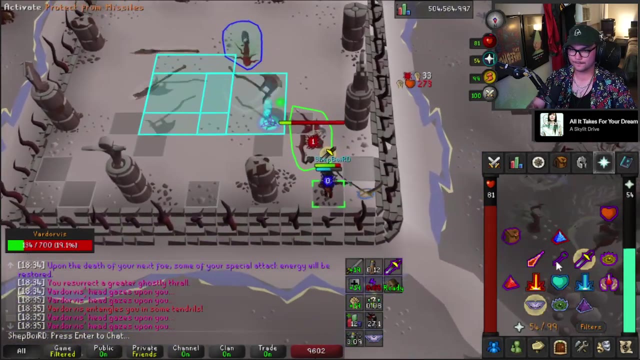 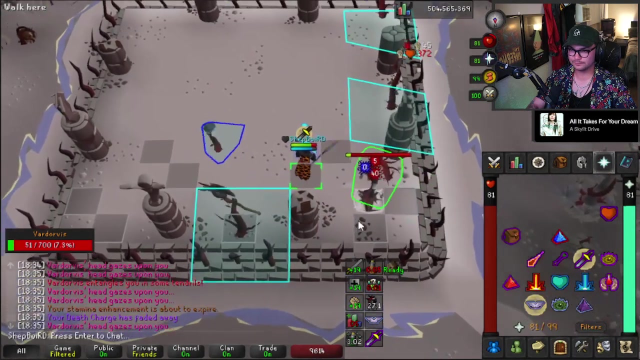 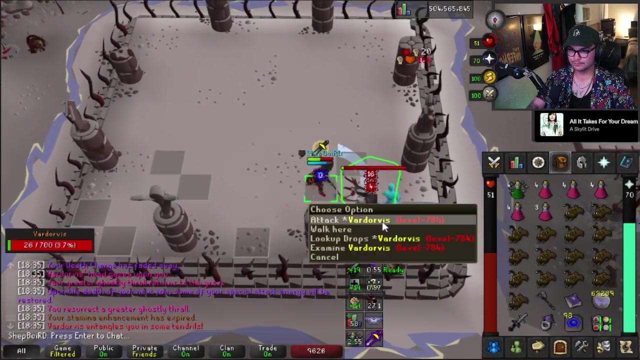 i bet, dude, like going back to doing uh off task zucks, like it feels so much worse, it feels so bad chip, good morning. how are we? how are we doing some vardoci, doing the vardoci, damn it. i just wasn't sure. i was like i, i thought i was gonna kill it, uh there. so i was like 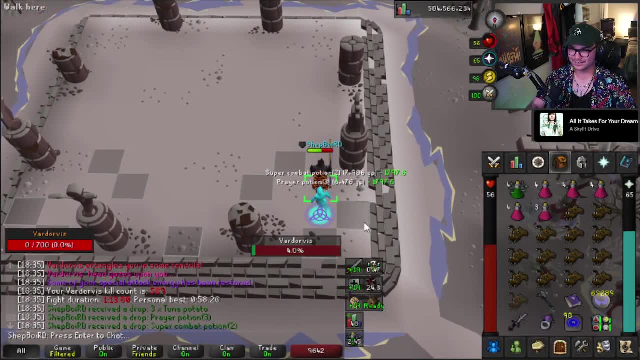 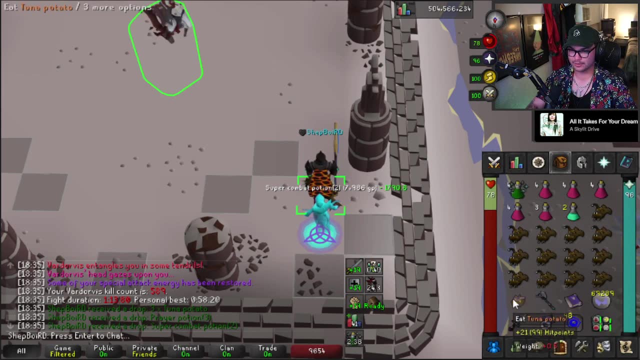 kind of nervous for the death charge. that's why i didn't didn't do the thing. i want to eat a tuna potato and then overheal with an angler. is this like five head? are you guys like proud of me? tell me you're proud of me. right, right, fucking now. 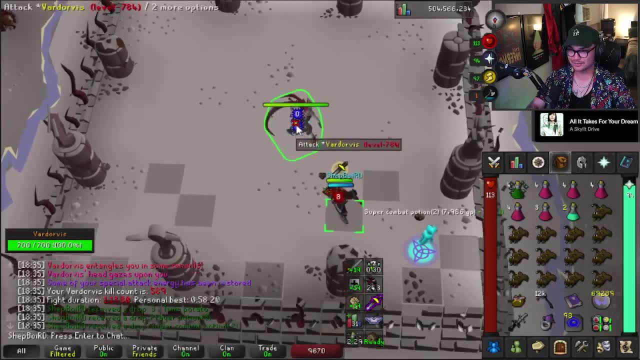 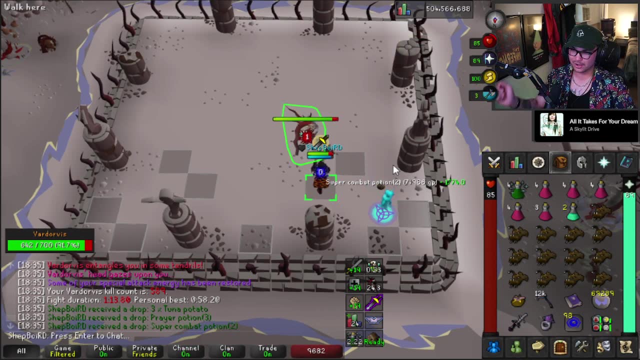 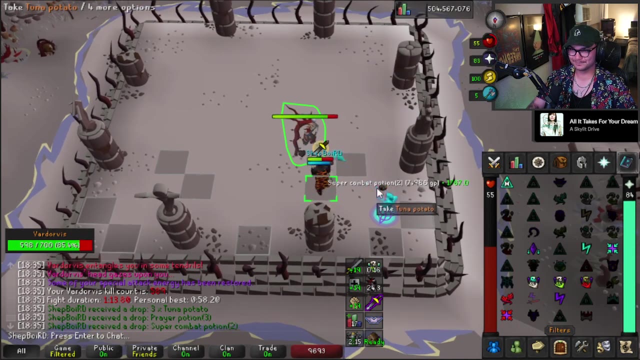 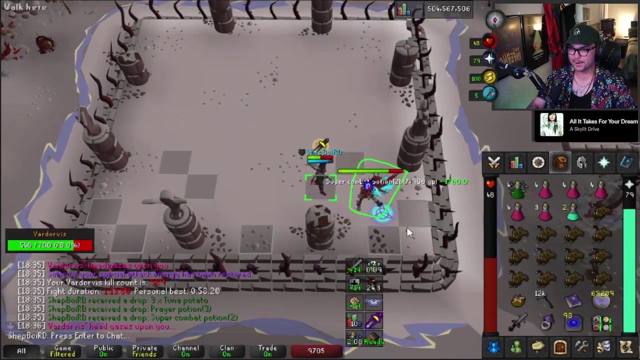 right, fucking now, that was some game: 200 million runes, jesus christ, to loot one. well, i guess you have a billion dollars in runescape gp slow class. yeah, we were gamer gamering there for a moment. i do have a bear's task too, i. i don't know what i want to do like on task with slayer outside of. 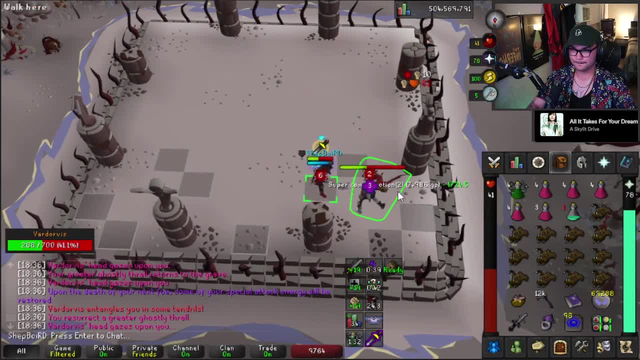 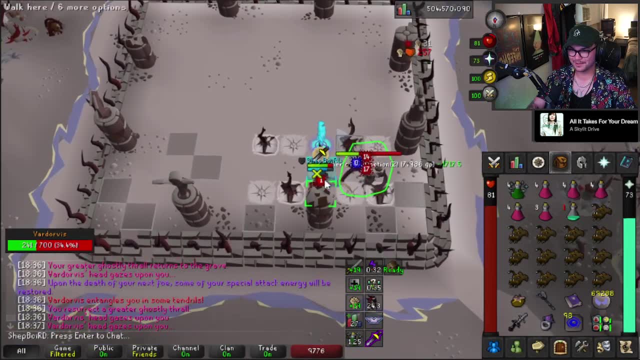 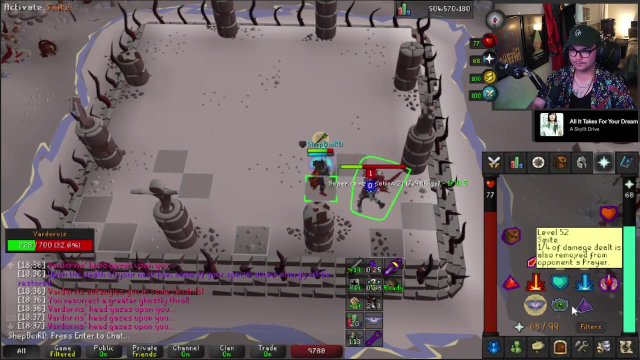 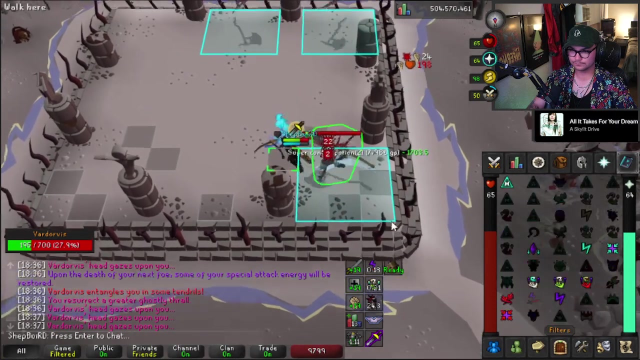 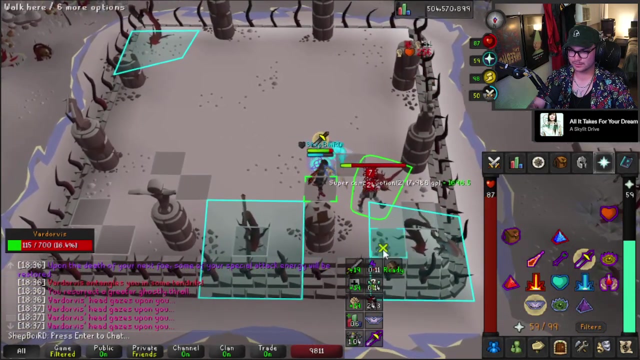 i need a lot of skilling time. go hunt some cloggies. what do you think we're doing here, babe? what do you think we're doing here? that's definitely, uh, not a ancient god sword spec. i wouldn't mind a bitch pet. i'm not gonna lie. 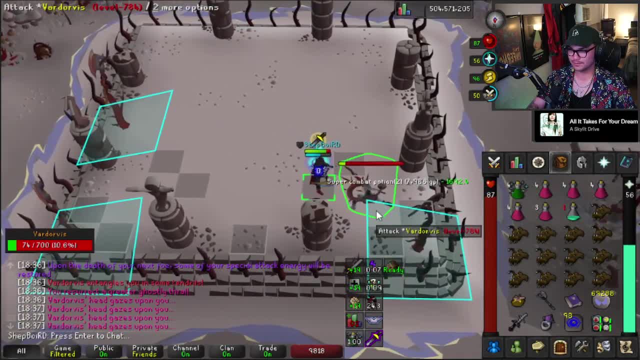 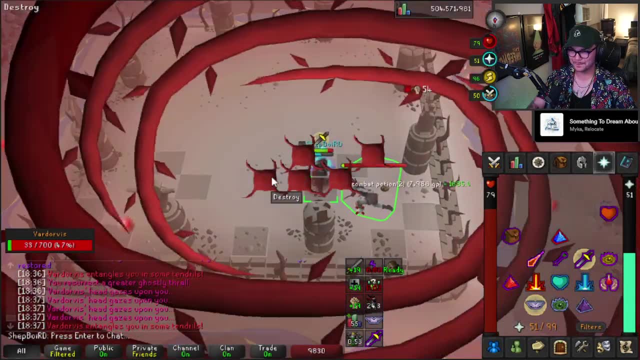 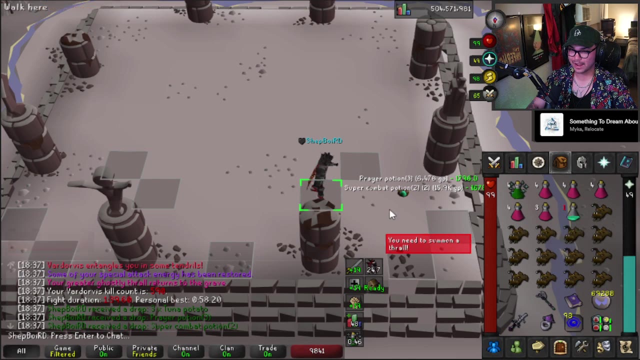 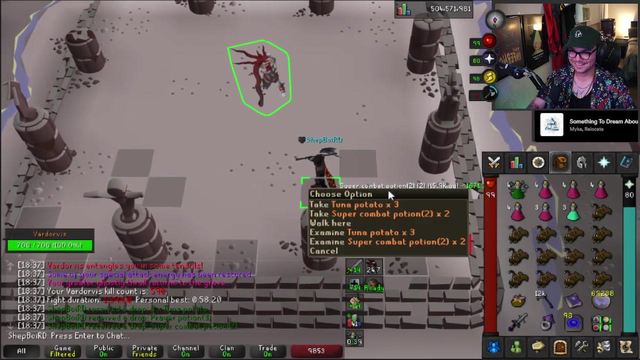 and a little ulti get the money back up. you know, i have another cloggy outside of a pet. it's my own, personal. i wonder what that would be, churchy, i wonder. oh wait, outside of a pet. actually, i do wonder what that would be like, because i figured. i figured you were talking about a suck. that's what i. 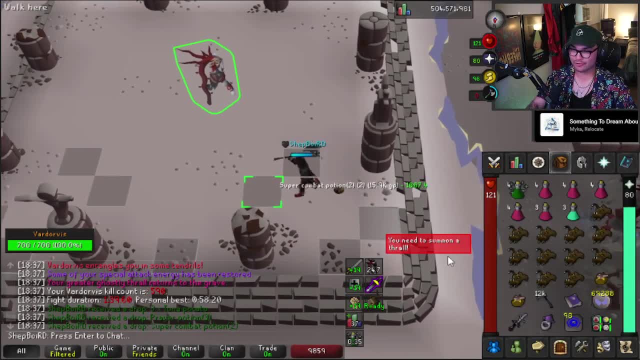 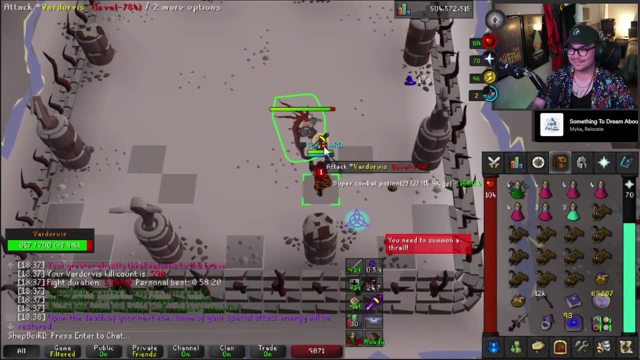 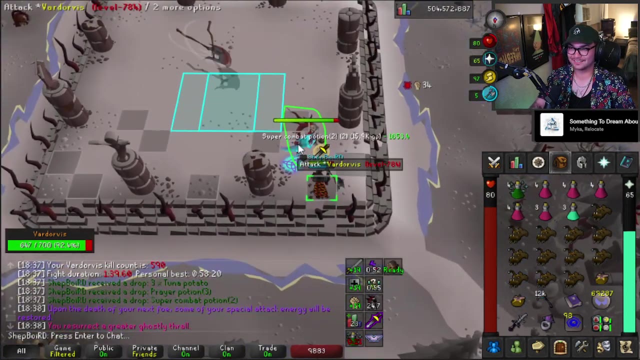 thought you were talking about. oh wait, yeah, that's right. that's right. yeah, dude, an eternal glory would be a sick clog, but yeah, that sounds miserable. 82 000 glories is insane. that is insane, dude. i have a clog i want from uh hydra. 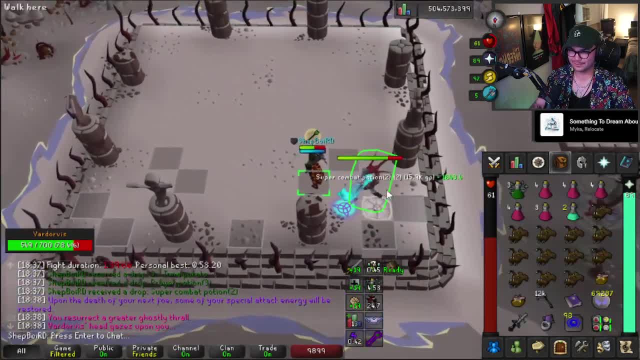 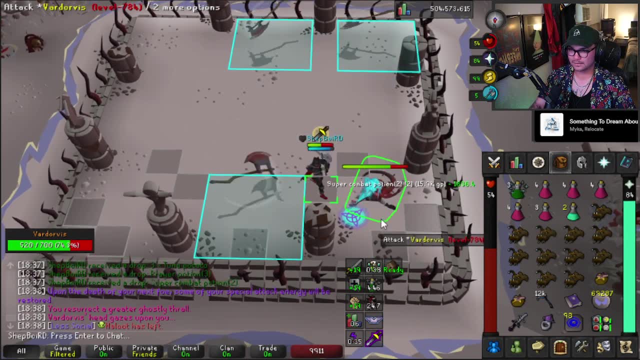 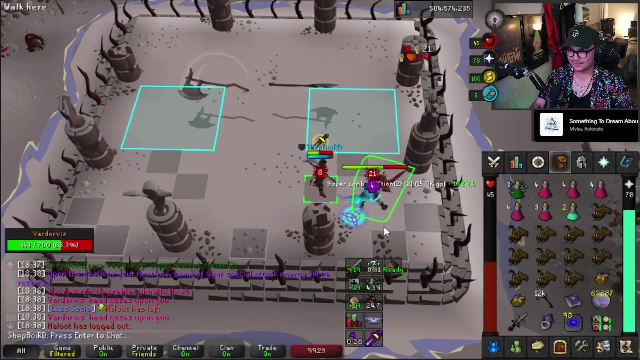 i'm almost 6 000 kc and that makes me sad, but really it's like the driest i've gone on anything like, just even pet wise like. i haven't gotten any pets like on here either. i don't know, that's insane. i just go four times. 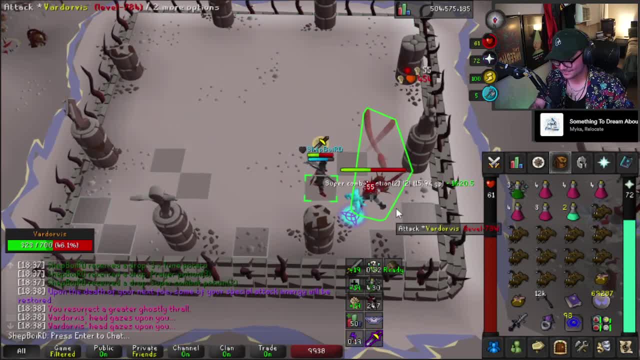 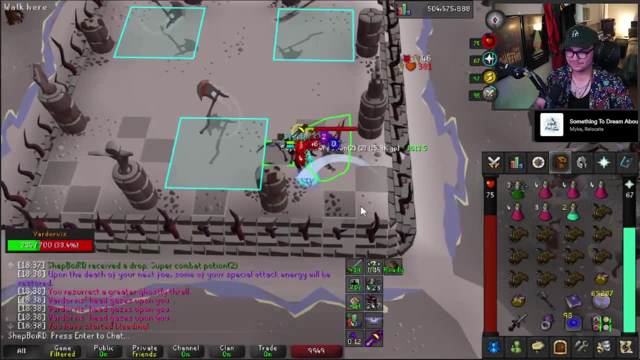 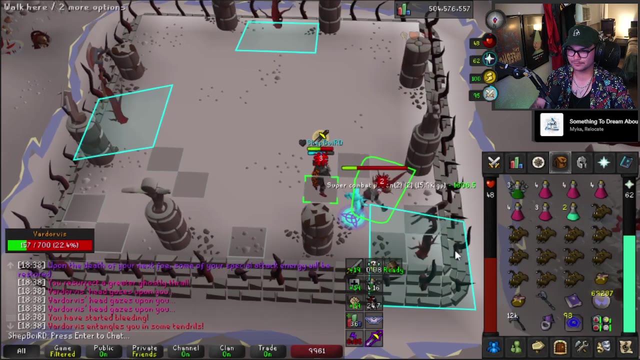 hey, you better not, you better not leak your world to herb. oh, i'm saying: oh dude, that was sick, that's super sick. man, if you ever see a dude in an uga booga mask- and uh, you know, an uga booga mask is gonna- 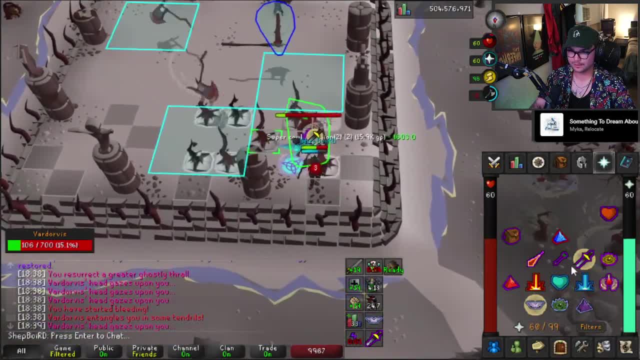 be the thing. what you're about to see is going to be aした life where the so-called wi-fi dogs- and they're not gonna get because of f3 Wuhan sutris to. you have to get some breath, boogamask and a fucking thingy. 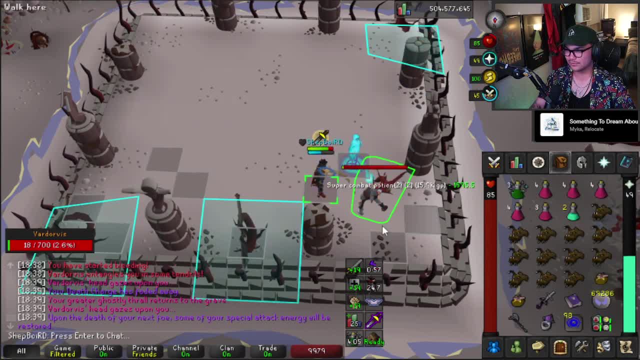 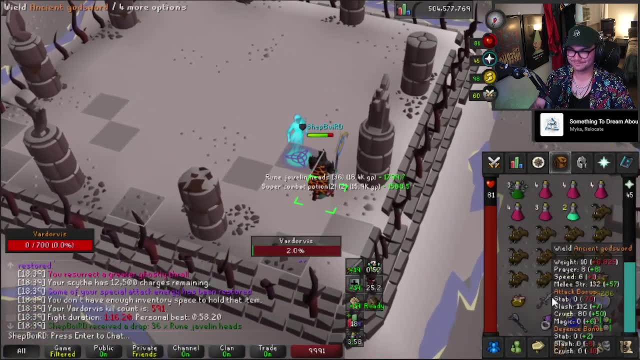 Four times for chaos. Ellie, Yeah, I mean, I'm getting close to right. Yeah, barrel chest, That's what I was trying to say. A bat chest Anchor Dude? I feel like I haven't gotten a lot of the money drops here either. 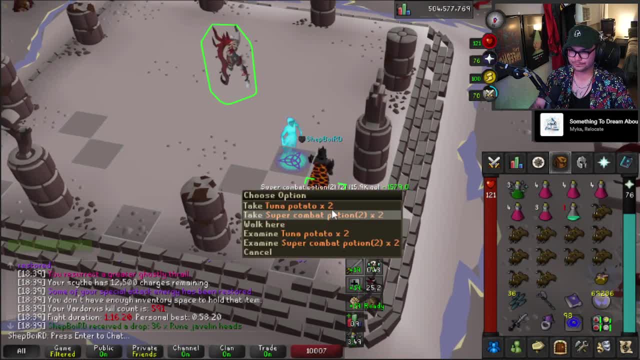 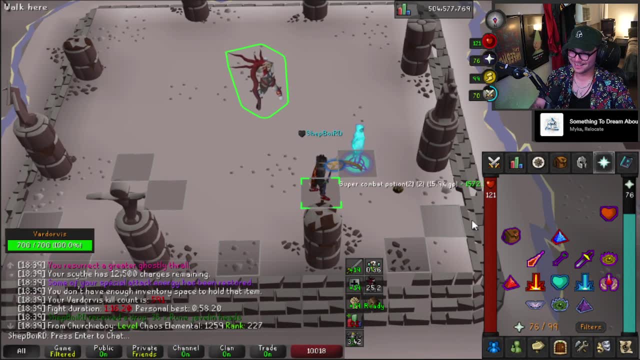 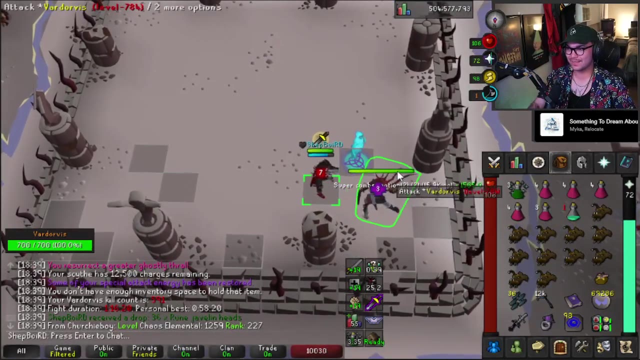 Like the onyx bolts and stuff. That is insane, That sucks, I'm so sorry. I mean I feel like that's what happens is like you get spooned on some things and where you go dry, like you go really fucking dry. 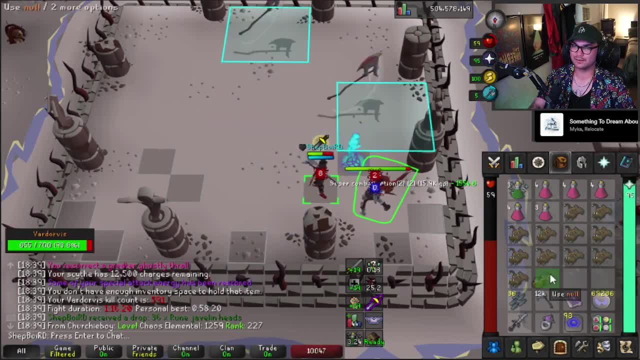 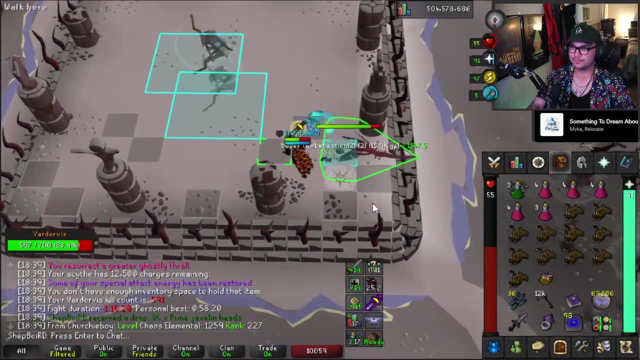 I don't know. Levi went pretty fucking dry Like I was almost three times right on my lure And then when it happened I didn't believe it. That little fart cloud holds a lot of meaning to me, Dude, that's base as. 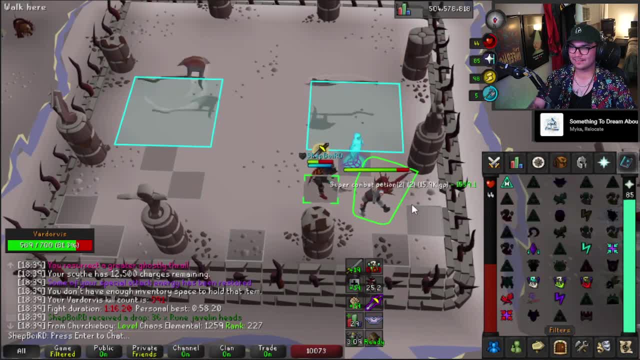 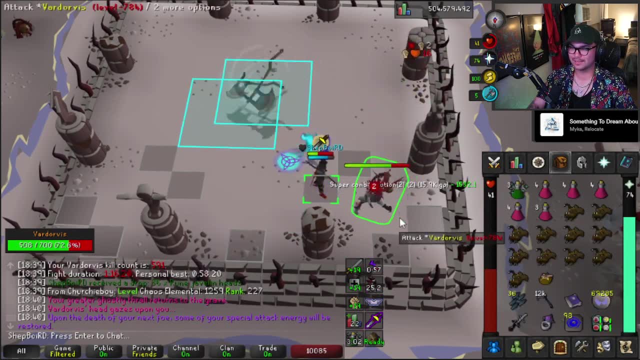 fuck, honestly, Base as fuck. Like that's something I kind of go for like every now and then, Like because during the charity stream I was like dude, if I just went and got a pet, that'd be a sick hit. like. 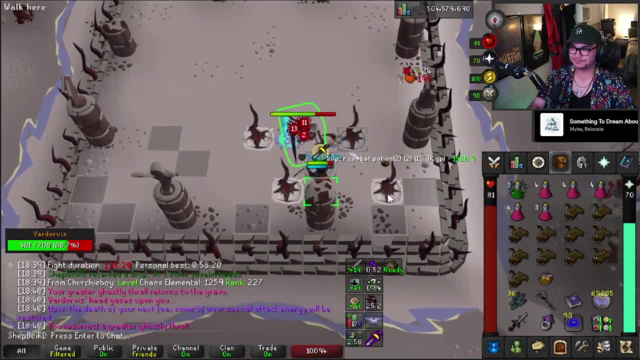 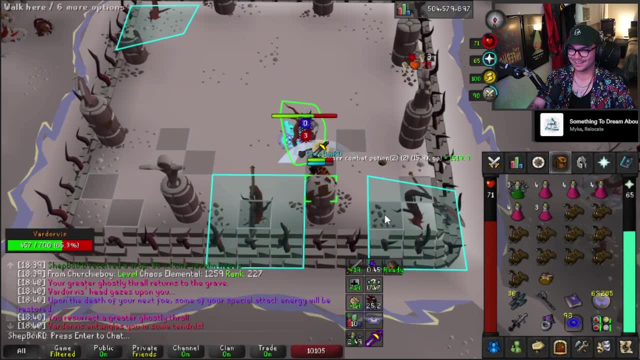 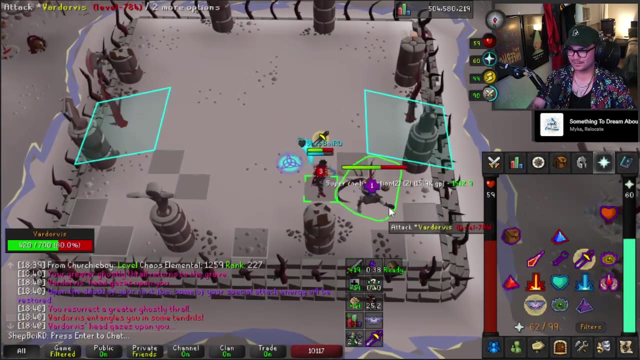 for the charity stream And uh, yeah, I didn't get any uniques, any loot beams like nothing, Nothing, Nothing. But it is what it is. I guess I share your pain at Levi. It also went insanely dry for the lure. 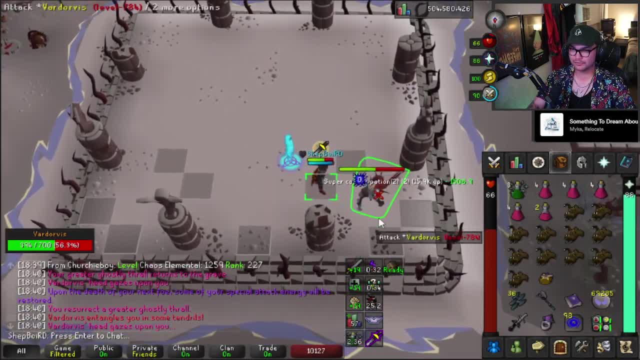 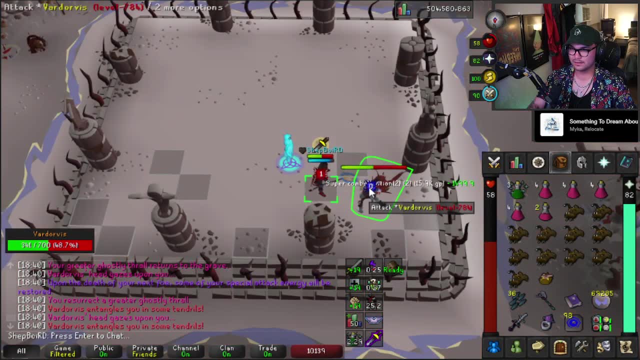 Yeah, But like I don't know, Maybe it's Stockholm Syndrome. but like I actually Levi, I would put at number two, Like I think Vard is my favorite. Uh, then Levi, then Whisper. 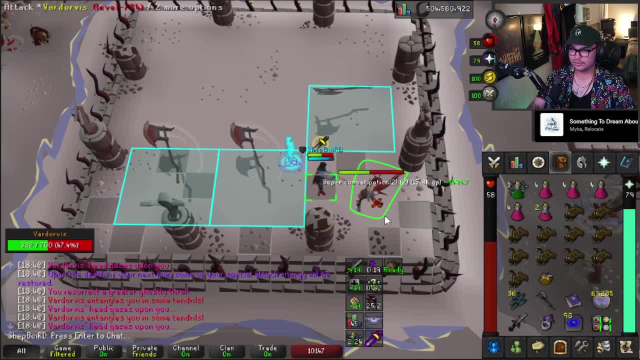 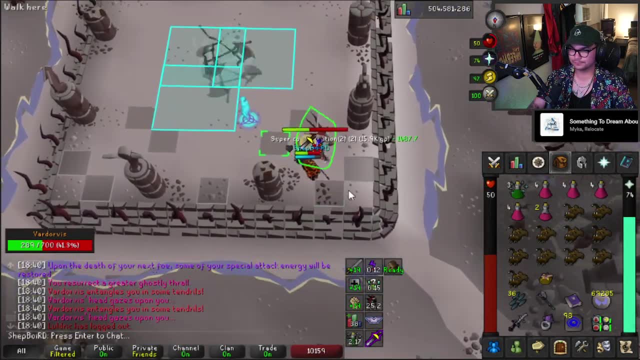 then Dude, Like I used to really like Dude because it was super chill. but now I'm just like I'm falling asleep, I don't know, Because I did a lot of Dude. Well, I mean, I did a lot of Dude on release. 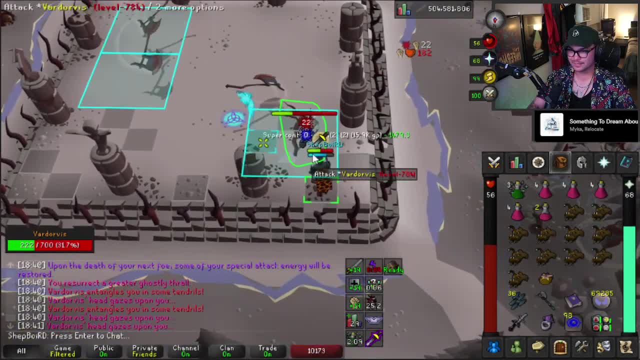 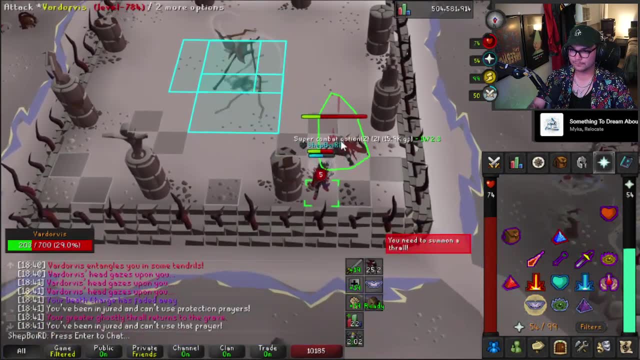 and I haven't really been back. I guess is how I should say that I was ranked 12, dude, I was ranked 12 Dude. I was like waking up because, uh, Oh, I just turned off my prayer instead of actually 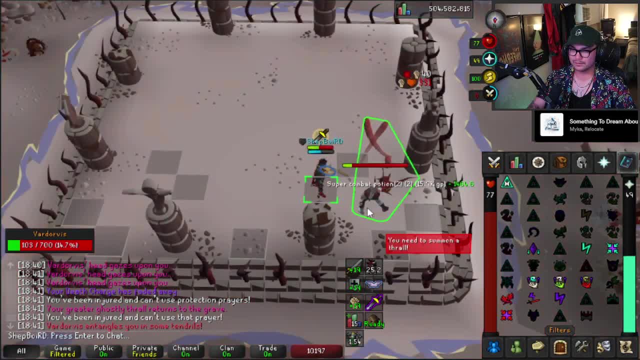 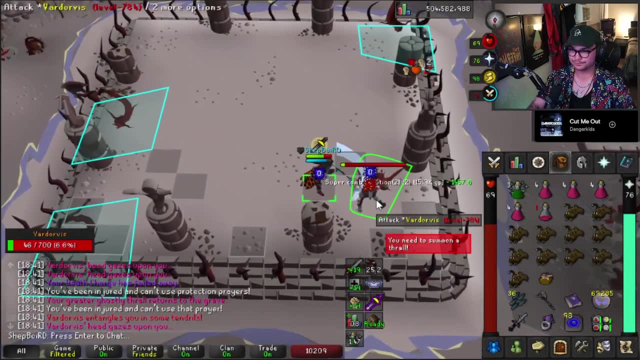 That was sick. Um so like when Dude or Desert Treasure 2 released literally the next day. I uh got my appendix pulled out And uh reminder: if you need healer spec, I'm outside, Oh shit. 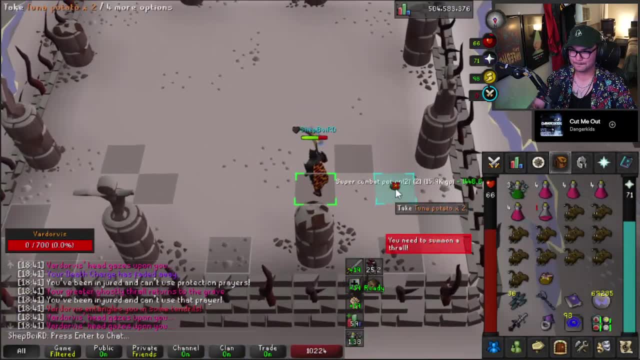 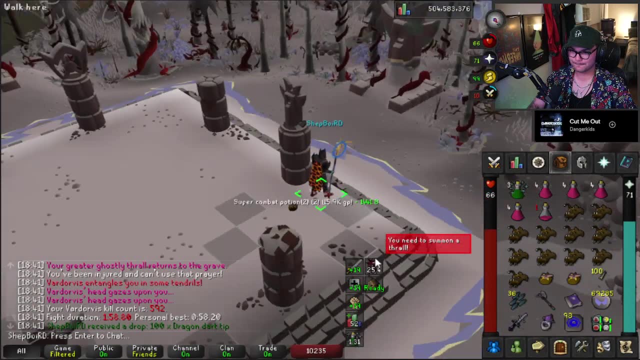 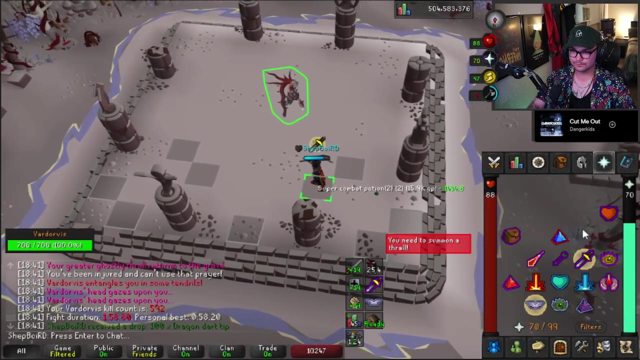 Oh shit, Damn. that makes me sad that that wasn't perfect. Well, I'm fine. I think I was about to like step out, but I got food. I'll just eat When I uh have free inventory spaces, then I'll. 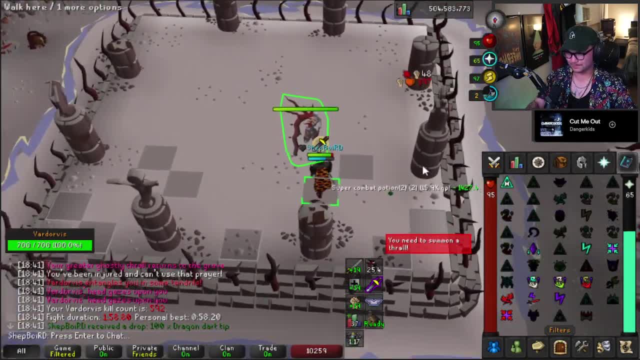 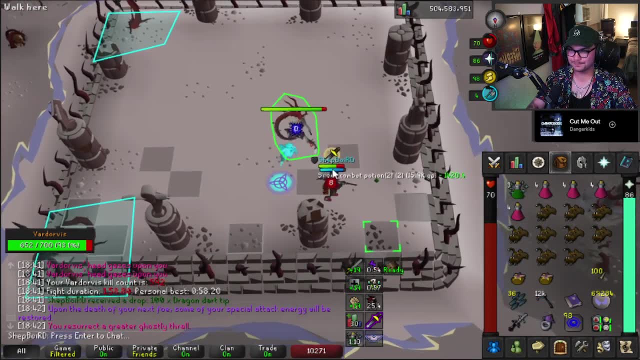 I'll do it, I will do it, I will do it. But yeah, I uh, fuckin' uh. I was like waking up and I would wake up at like 3 o'clock in the morning and go to bed at like. 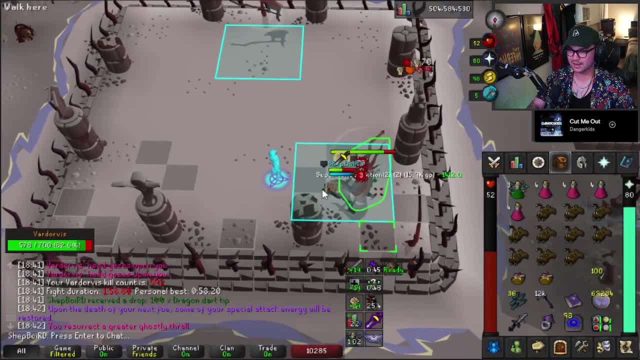 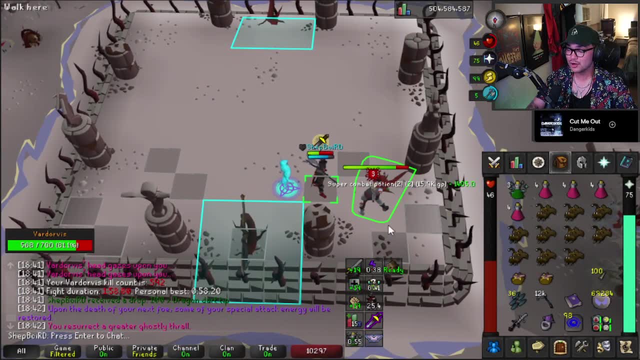 8, and then, like some days like I would like stay up all night and just continue to grind dude Um and yeah, I was ranked 12, like uh, fuck, I lost that screen. 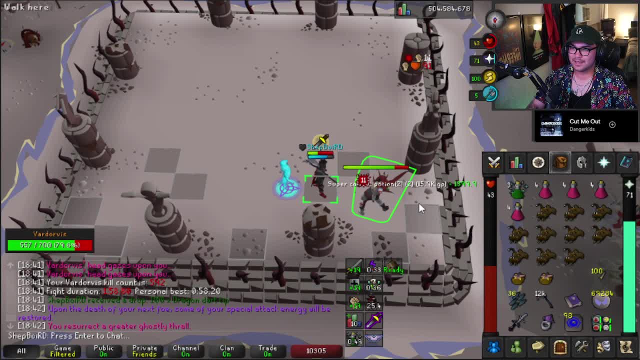 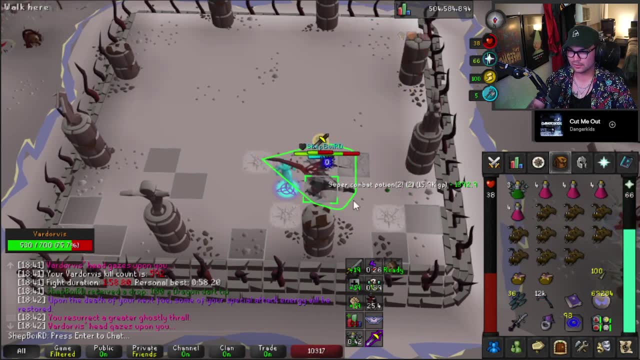 No, it's on my Twitter. It's on my Twitter. Yeah, I was like cause, uh. so when I reinstalled Windows, I lost a lot of my. uh, I lost a lot of my, like, old clips. 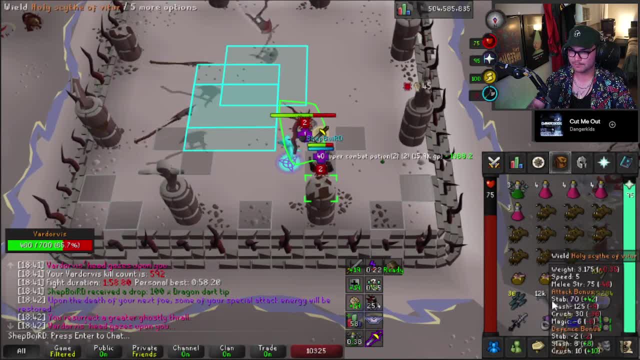 and screenshots and everything and it like I'm actually like really bummed out about it. Um, I didn't lose anything that was like super, super important. like in my personal life It's just like all my RuneScape. 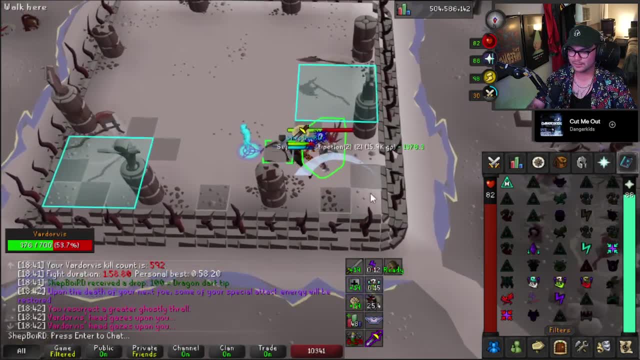 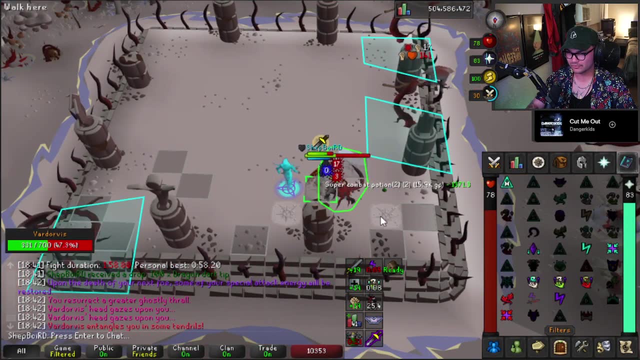 memories, Um, but even still, like you know, it really sucks. It really sucks Cause, like, the only two drives that got wiped were, uh, my OS drive and then the drive for, uh, uh, uh, what's it called? 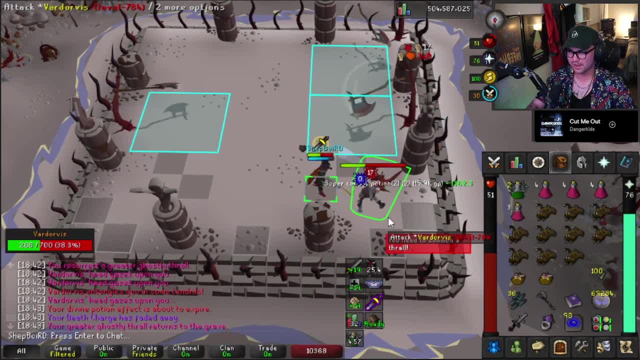 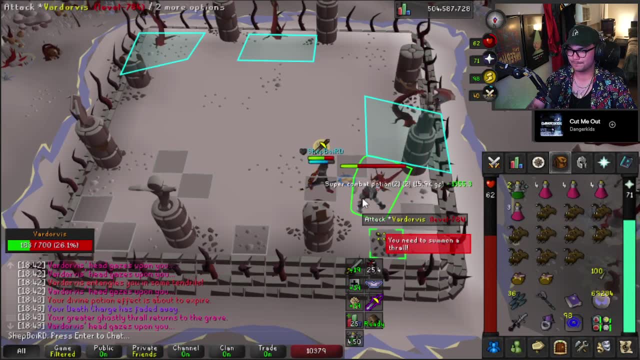 Uh, that I use for like stream stuff, like clips and all that stuff. And uh, I had a couple projects for the old YouTubes, um, that I was like on and off working on and uh, 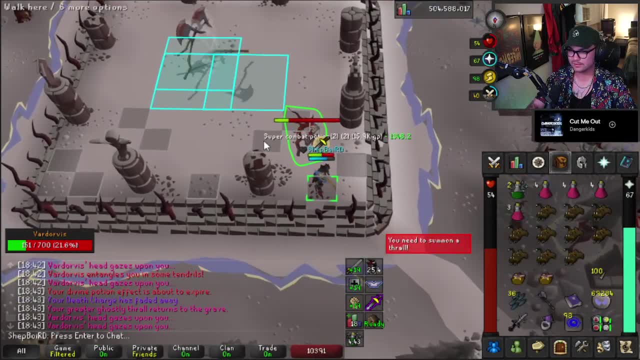 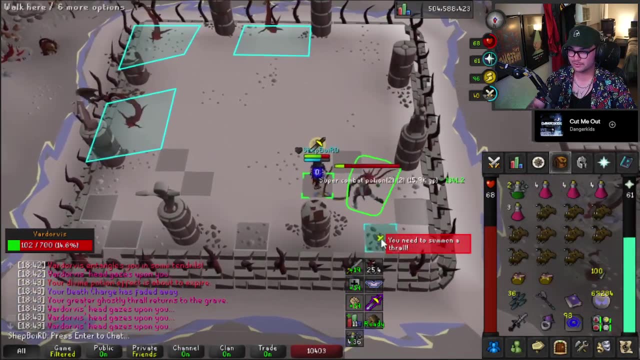 I lost those and I lost all the footage, so that sucks. Been streaming a little more lately, uh, been finding it a lot of fun. Yeah, dude. um, I've actually been streaming less lately, but I do always enjoy streaming. 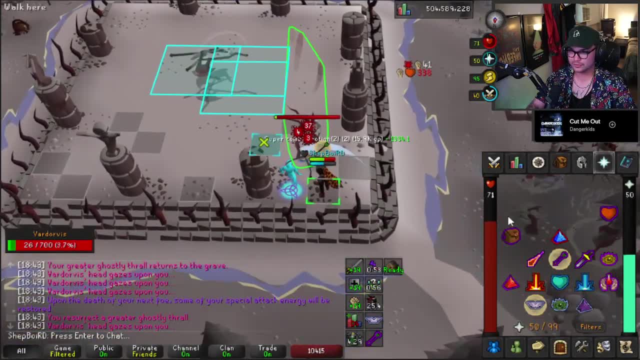 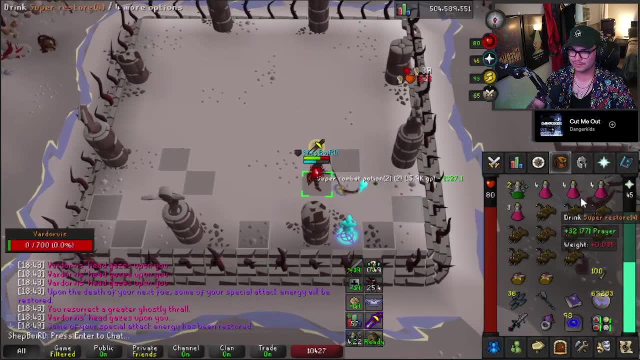 Like I don't know. I've always enjoyed it. I'll have to tune in at one point, Cause I I don't think I've ever been there for a churchy stream. Actually, now that I'm thinking about it, 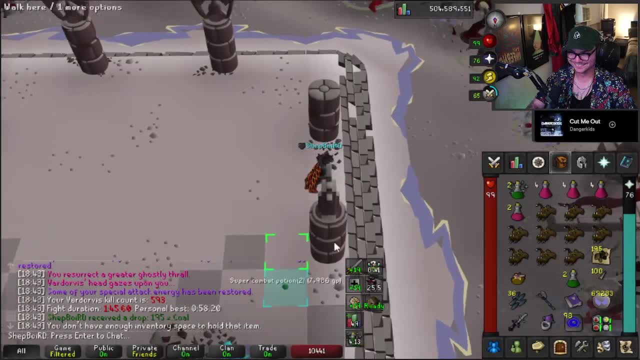 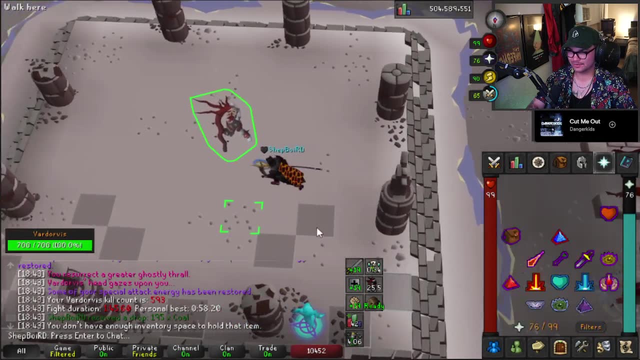 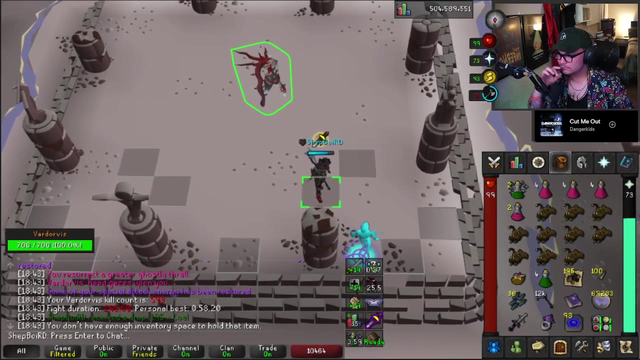 I'm just egoing the shit out of you. you know I'm kidding. I'm kidding. I streamed six of my last twelve infirmars. Did you stream today? Hold on, Yeah, I'm following you. I don't know. 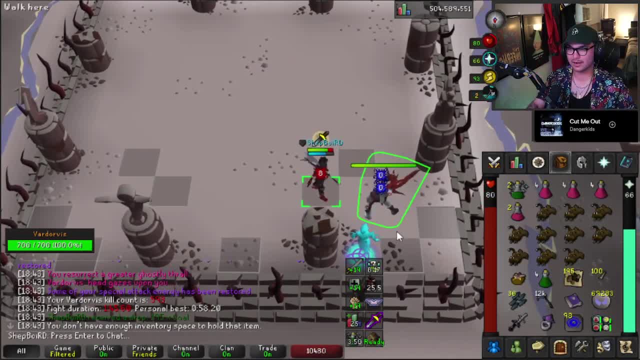 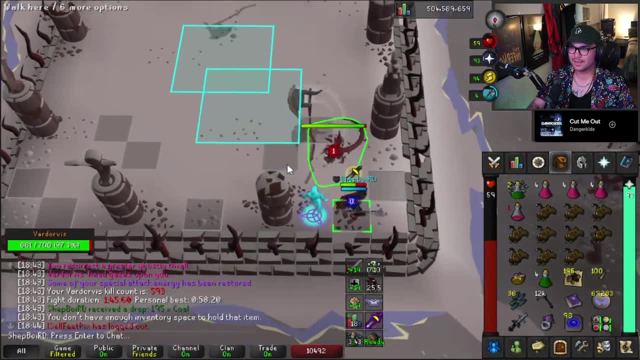 All three completions. That's huge. I'm still not at a point where I'm like 100%-ing Inferno, Like it's still a toss-up, sometimes like cause I still like, and the thing that's bad is like I'm good. 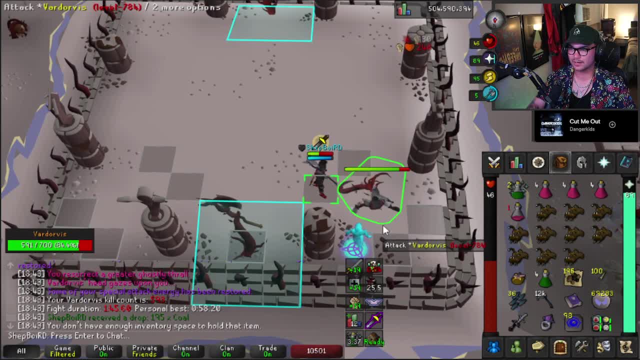 enough at Inferno that like when I fuck up, I know exactly what I did and I'm just like it just feels bad cause I'm like I know the soul and like as soon as it happens. 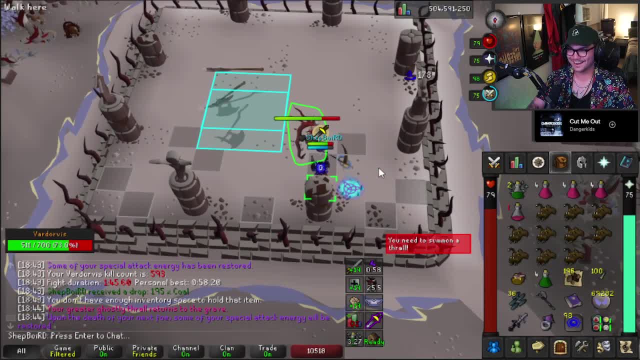 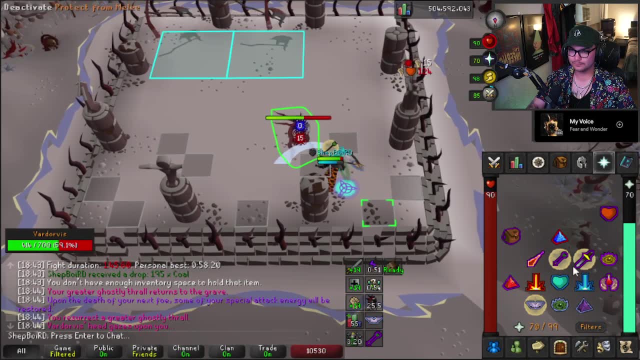 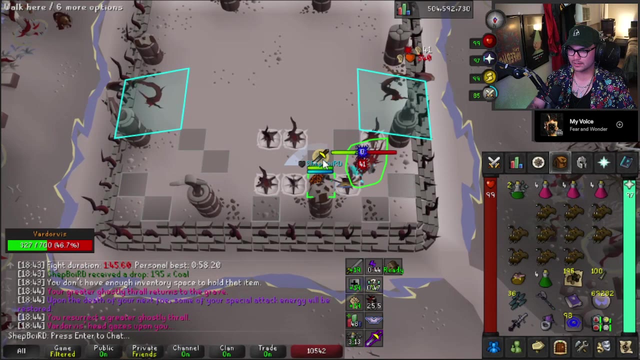 I'm just like feel really bad about it. I don't know, I don't know. At least it makes me feel bad, Cause like I remember when I was learning and you know I would just die. and then I'm like, how did I die? 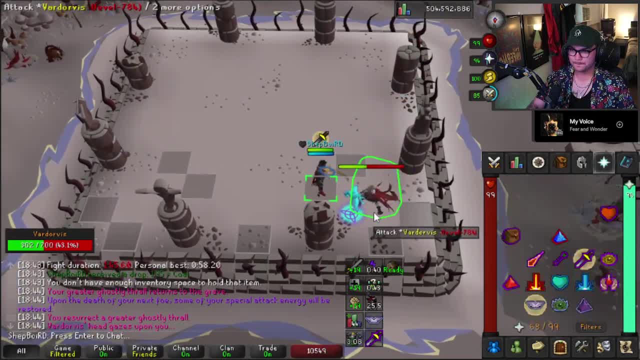 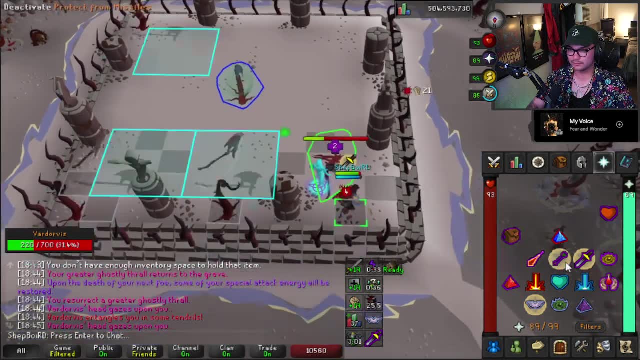 You know, and it's like confusing- I need to go on a, uh, nightmare arc and that's something that I like kind of want to do. I just like haven't buckled down and done it. 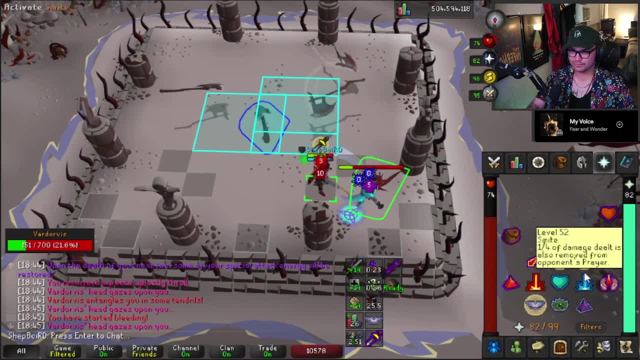 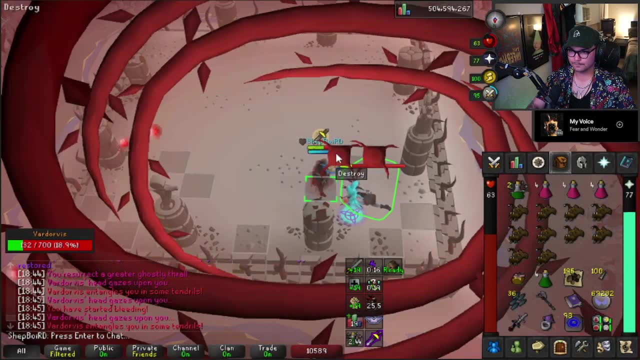 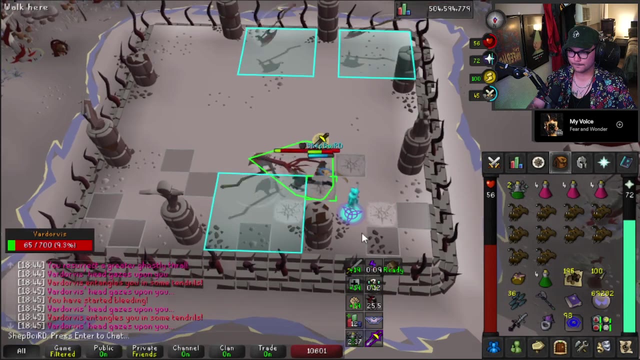 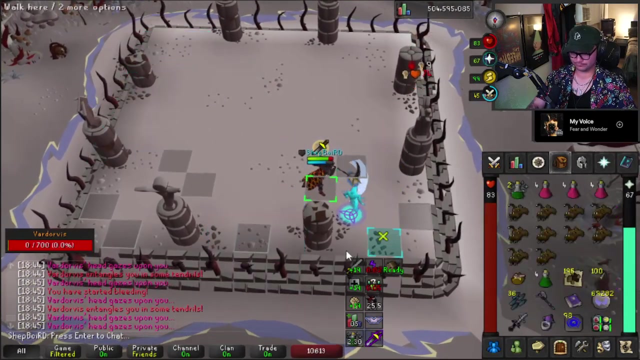 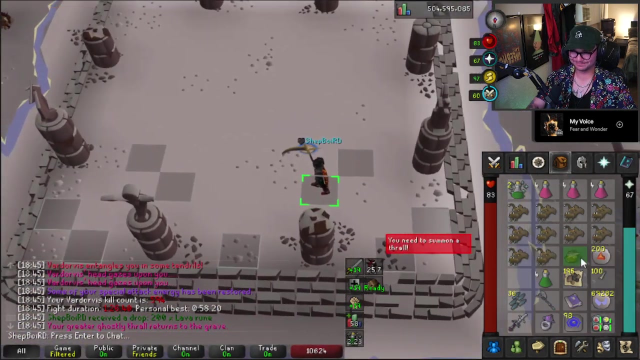 I moved so early, dude, I moved so early. I moved so early. Surely I get spooned an Ultor. Surely I get spooned an Ultor, right? Does this cope, Like because I went dry for all the other vestiges? like 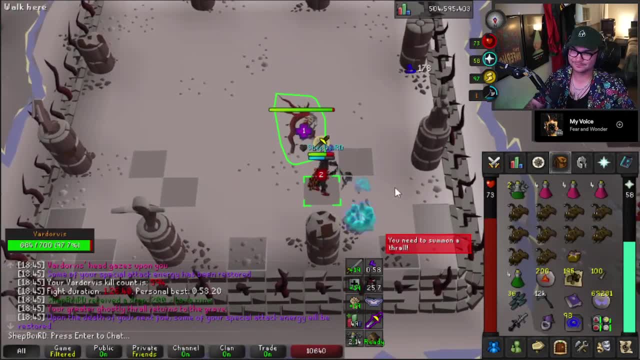 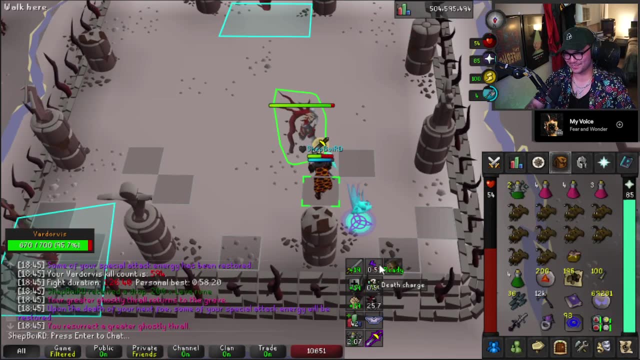 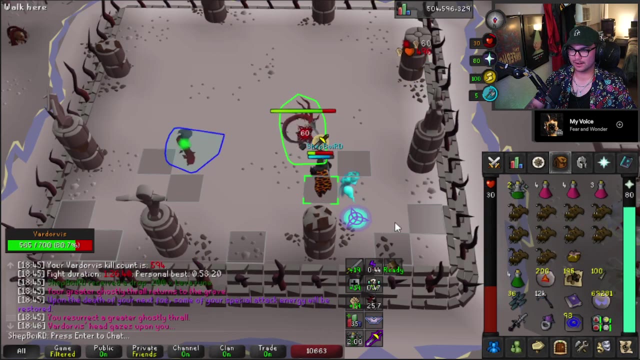 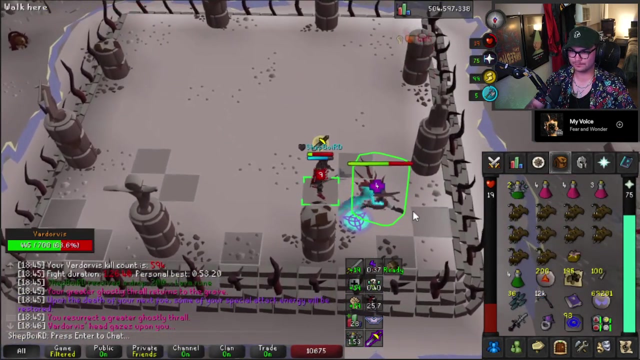 do I, uh, do I get spooned an Ultor? Cause I deserve it right, Like surely, Surely, I deserve a fucking spooned Ultor, Like at least it'd be ice anyway, I don't know, Dude, I'm getting smashed. That's the Bodhi number Into the. 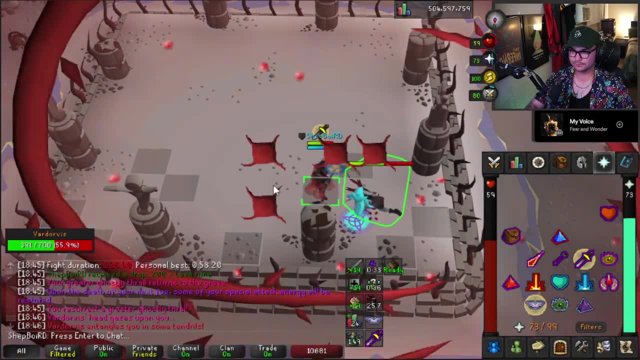 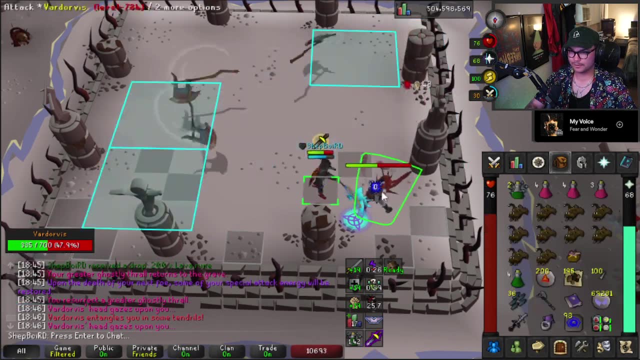 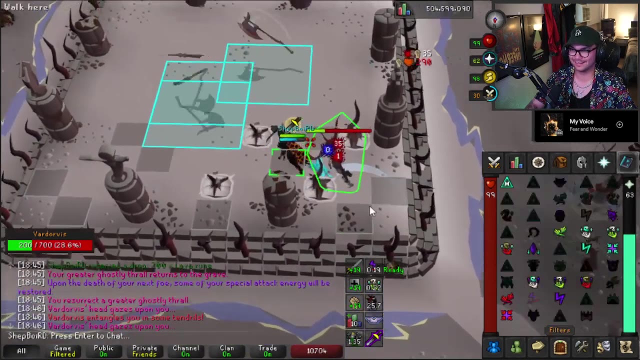 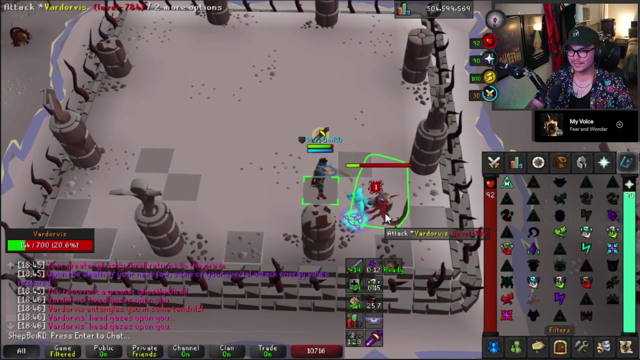 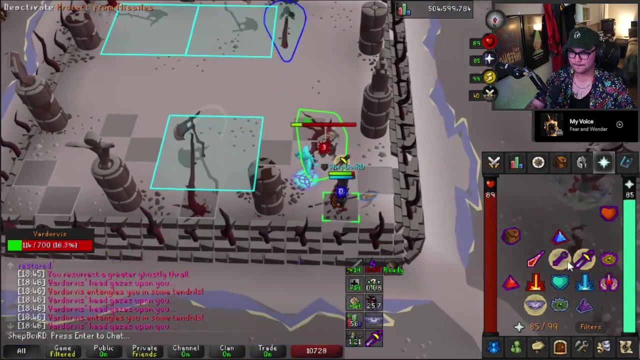 49? I'm just gonna spec early and I'm really glad we got all the shit DPS out of the way and then now we're back at decent DPS, I don't know. And then now that I said that, you know it's like 2, 1, yeah, okay, I spoke too soon. I spoke too soon is what happened. 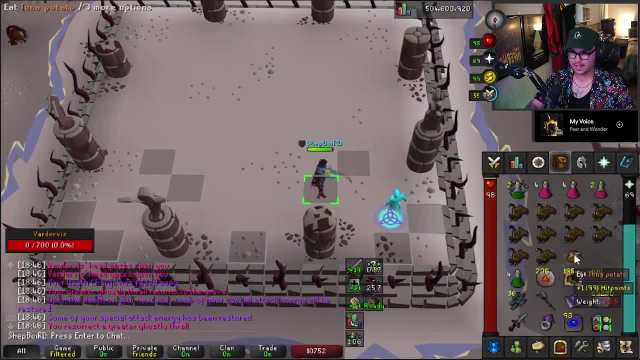 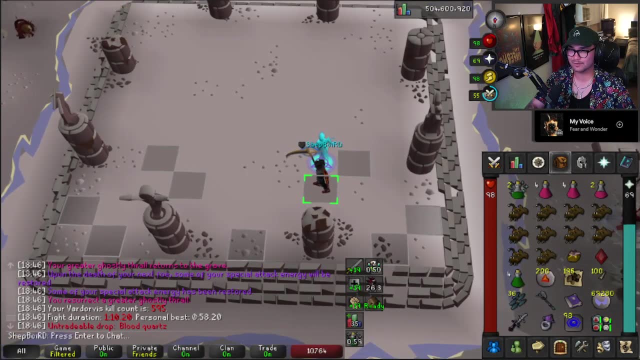 I thought I was gonna miss that, but I guess I didn't. I guess I didn't. Blood Quartz: How many have I gotten? I've been like hella. I've got 7. 7 Blood Quartzes. dude, I'm tired. 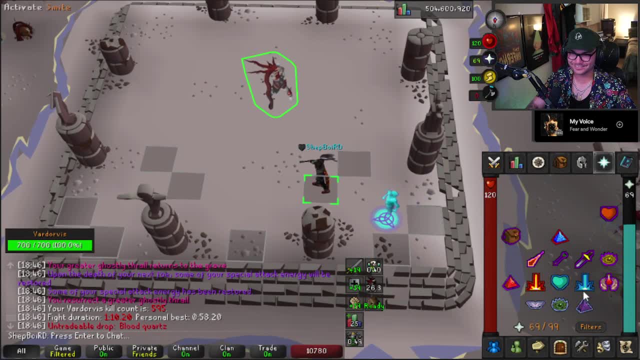 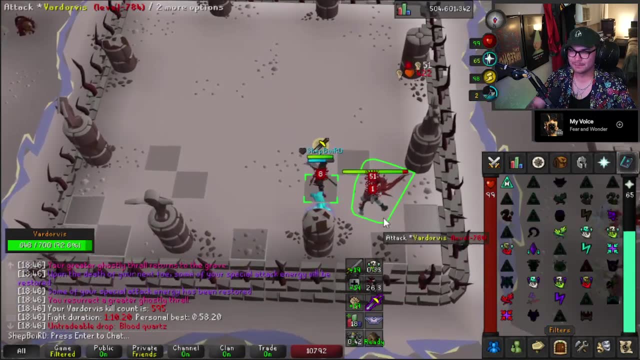 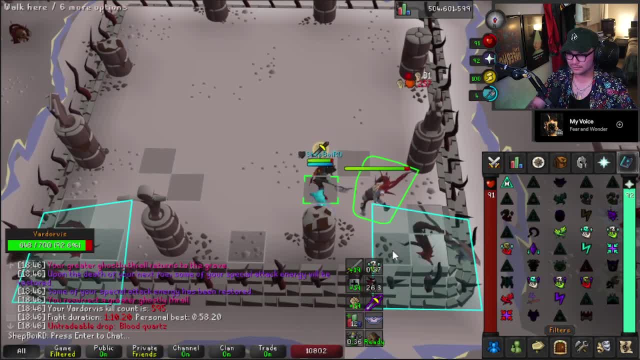 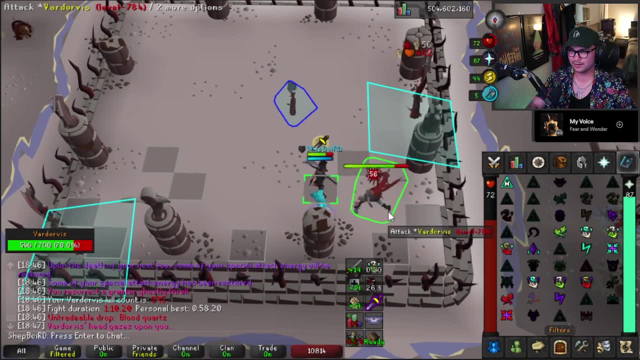 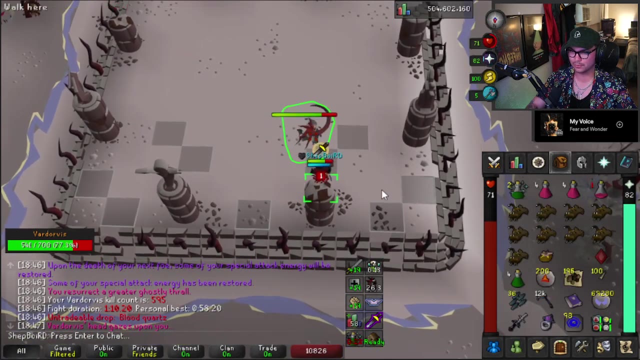 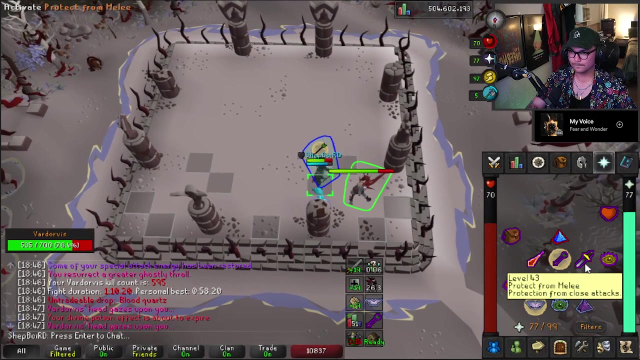 Levi, Levi, Levi, Levi, Levi, Levi Levi. I think I only had one. I don't know My Divine's gonna pop, so I'll just like just do a normie super combat Axe is back to being not good, Oh, Oh. 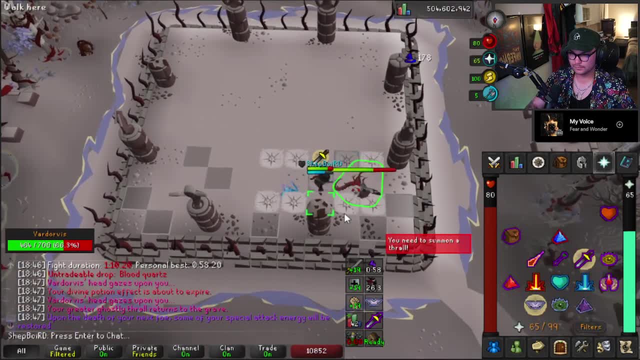 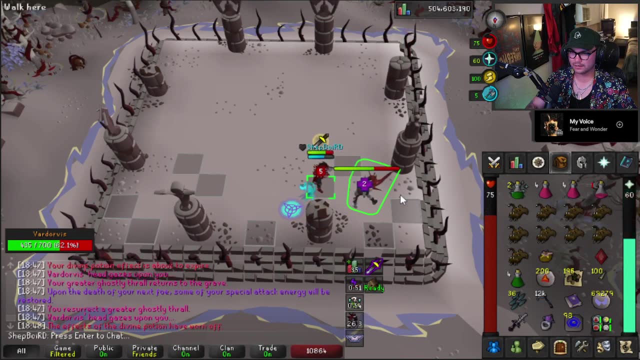 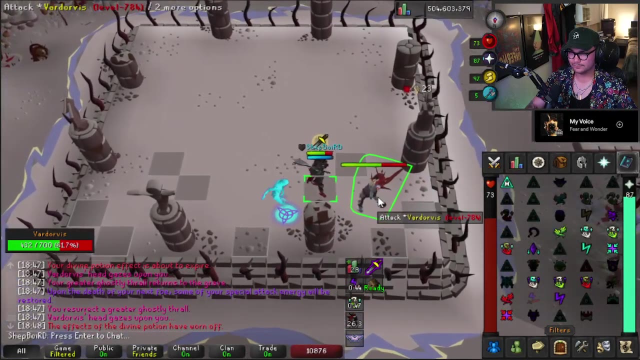 but yeah, I'm not sure on uh my quarts, because uh, yeah, I know, Levi, I'm dry. I think I'm dry at uh Duke, I don't know, and I wish they would like go back to the. 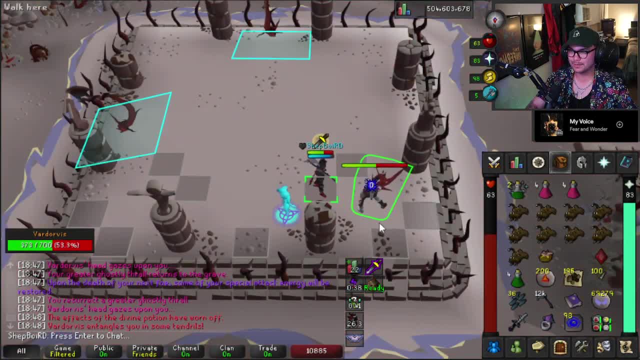 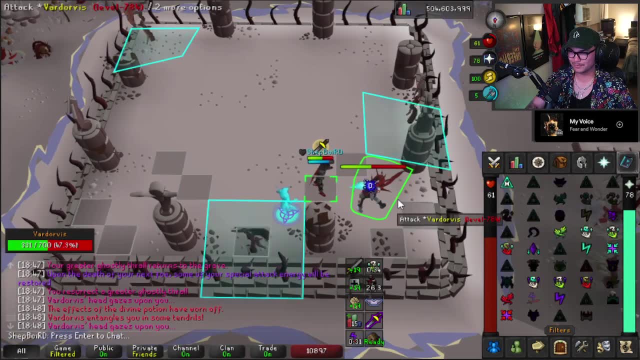 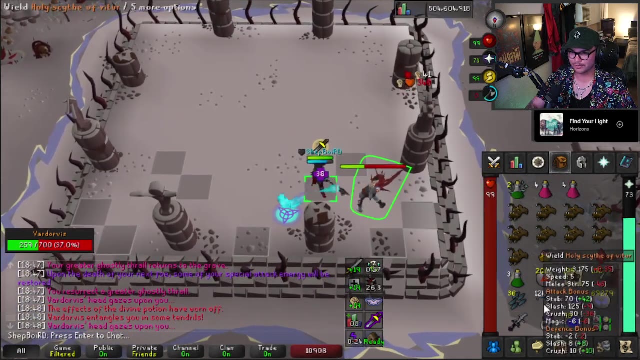 other bosses and anytime like, or maybe on ground items, like anything that's tagged like add, add a uh sound thing, would that be weird? like make it to where you can add a little sound clip of like you getting a drop just to like trigger that dopamine response like 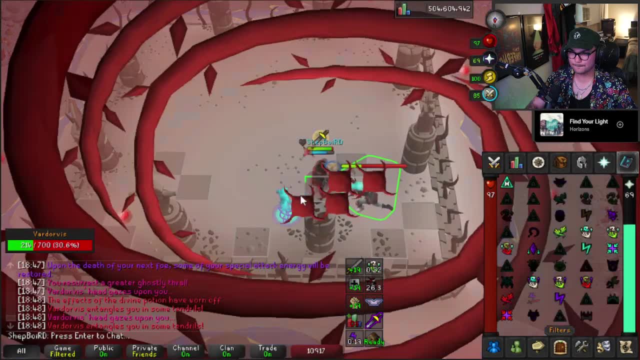 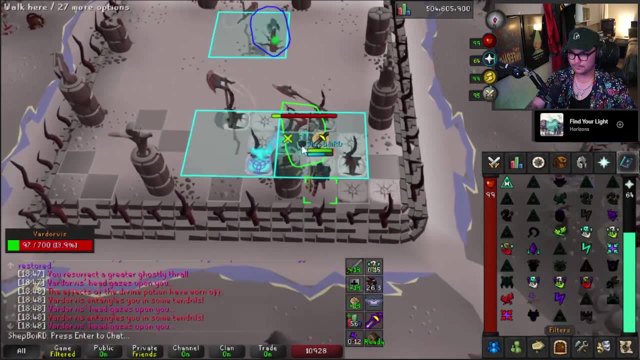 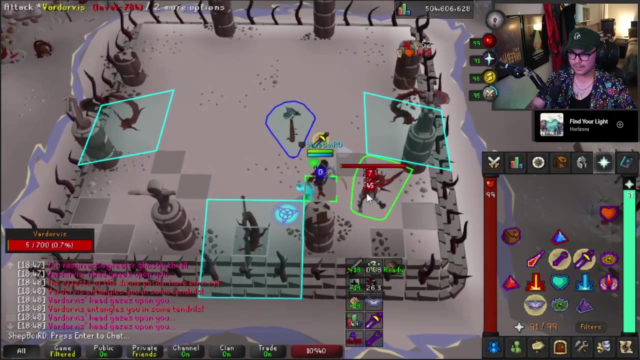 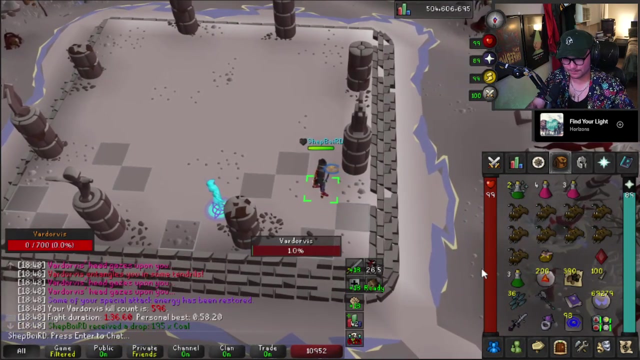 I think that'd be sick. We're gaming- Gamer-ing is a thing- Blamo, Blamo, Never the back-to-back jingle, Uh, okay. so yeah, let's see collections. there are plugins where you can add custom. 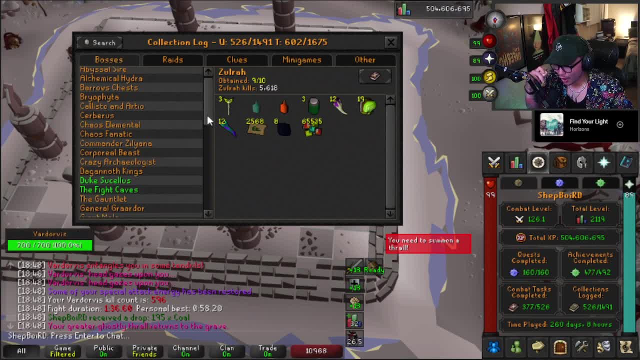 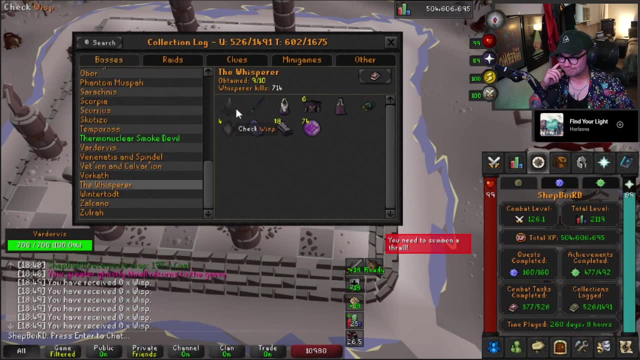 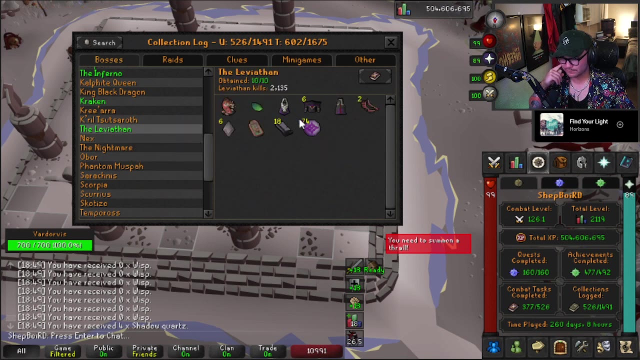 sound effects, so in items of certain value, really, Oh fuck, Because, yeah, that'd be cool. Okay, so I'm a little underrate on Whisperer. Let's see Leviathan Six. I'm like way, way underrate. 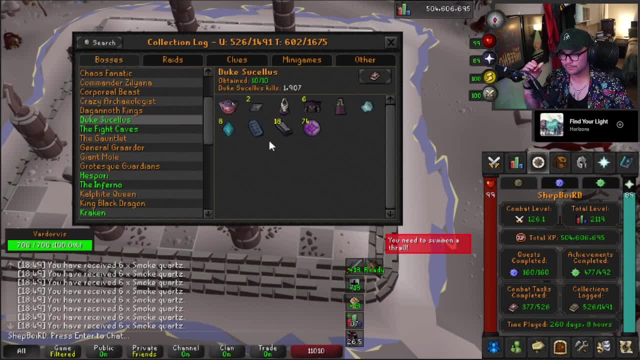 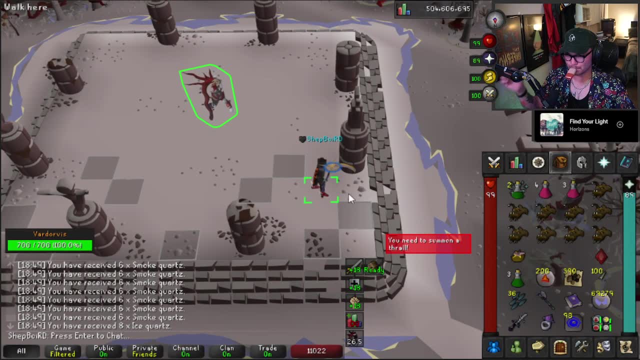 Uh, or sorry, I was overrate on Whisperer Duke. Oh Duke, I have eight. Fuck, never mind dude, I was capping out my ass. I do be capping sometimes. It is unfortunate, but it's true. 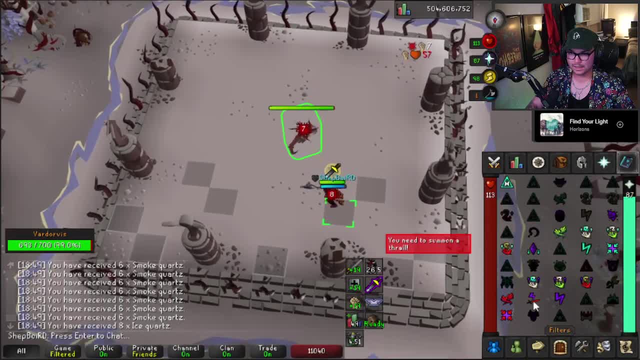 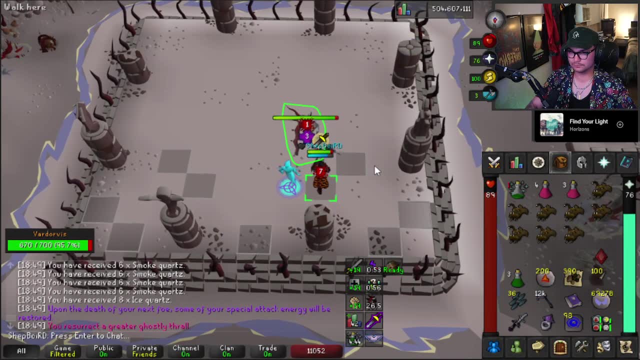 It do be true, But that is okay. I think I might change up the music. I don't know what I want to listen to right now, Because I kind of want to listen to hardstyle, but then I'm like, not really. 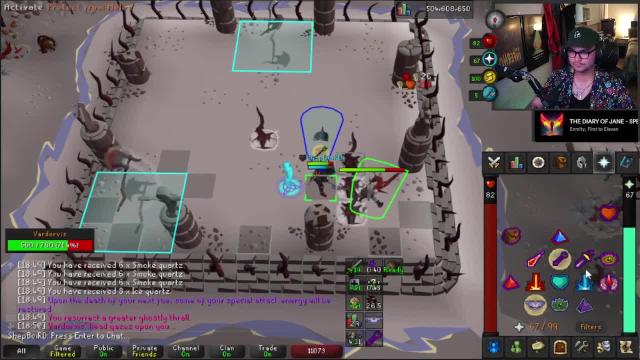 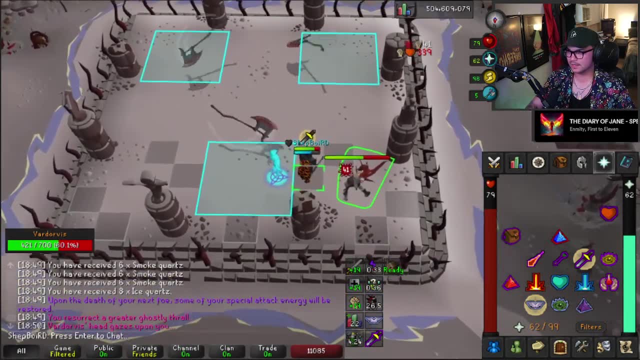 Then I'm like I wasn't really feeling the stream for this. It's like a mix of like hardstyle and trance. There's a lot of like covers on this uh playlist. There's a lot of covers on this too. 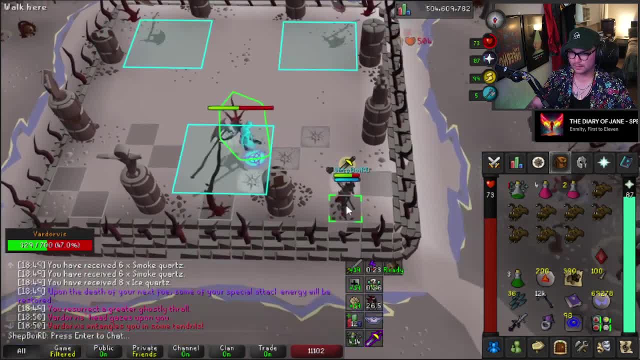 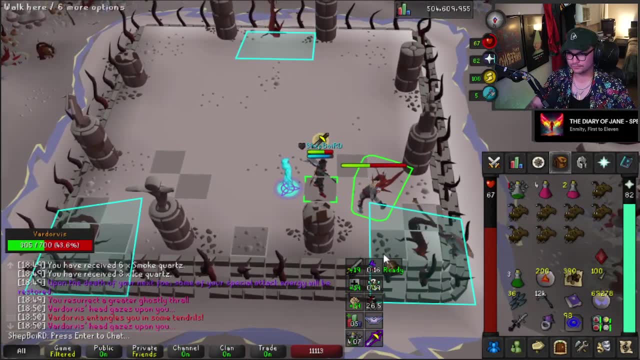 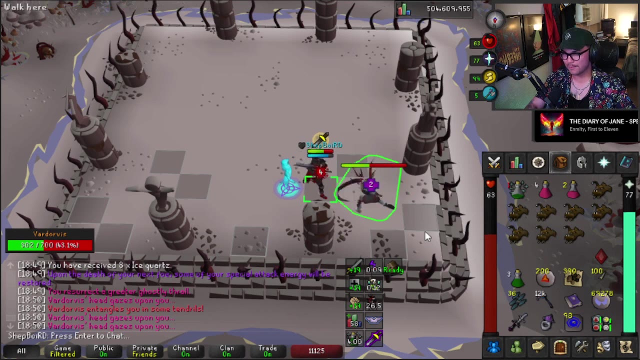 Gotta turn this up just a hair. Poor me. That's not too loud for you guys, Not too much louder. My vape almost killed me there. Huh, Huh, Senserton. How are we King, How are we? 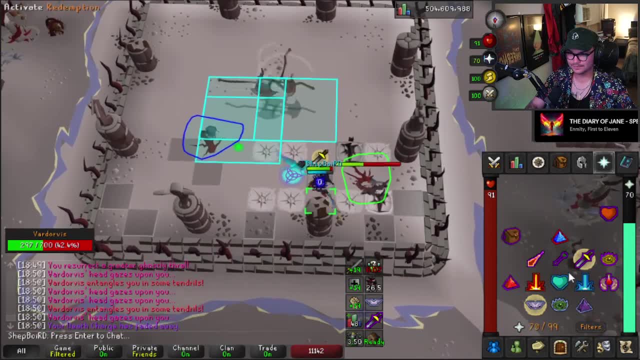 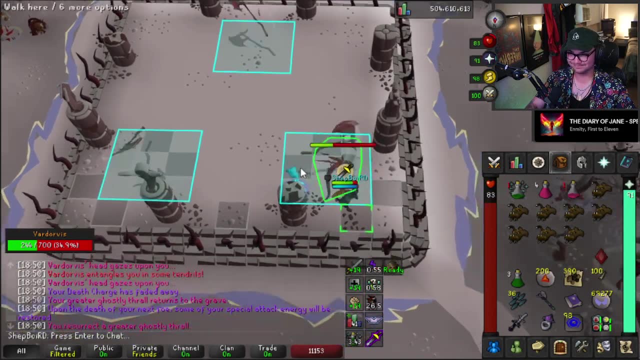 We're doing some more dancing. We're doing some more dancing, Although bug is fun. Actually, I don't know. I do want to. I do want to play RuneScape for a little bit. How we doing King. 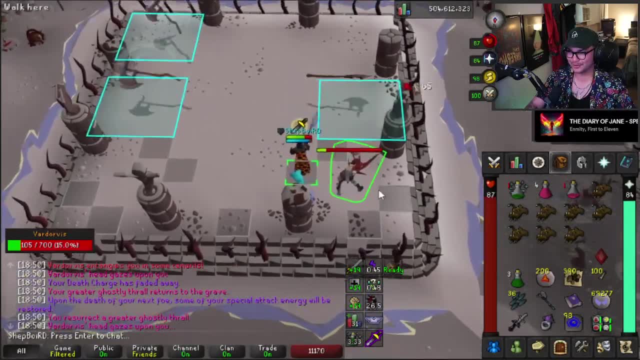 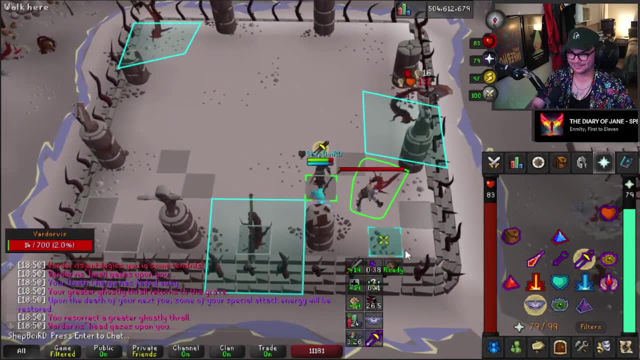 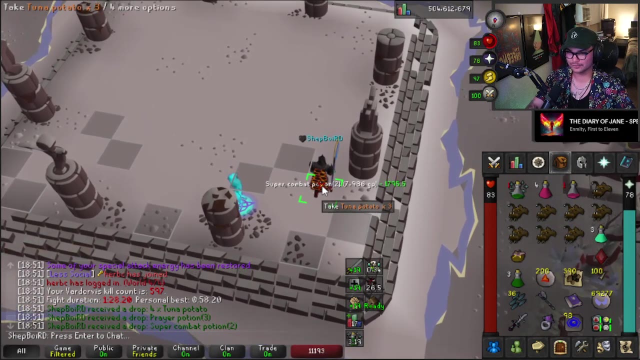 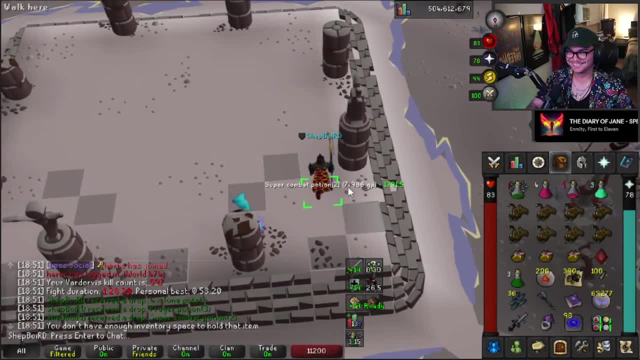 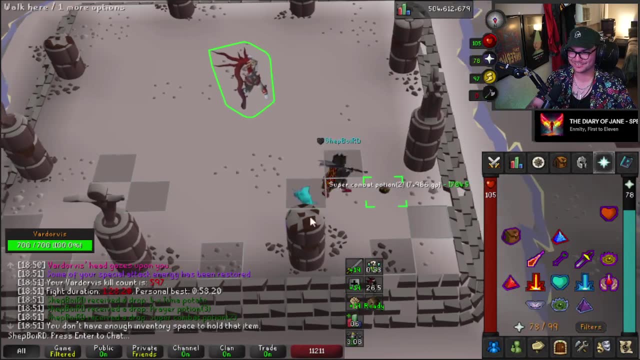 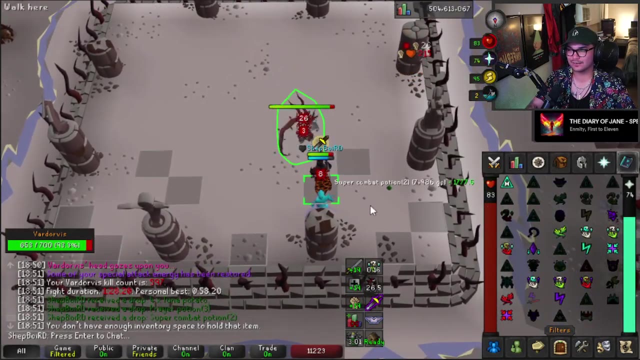 I mean, what Game's fun? Want to play more? Yeah, you're goddamn fucking right, dude. You're goddamn fucking right, brother Dude. I like I don't know It's so fun Because it's like, especially like on the like earlier difficulties, it's like turn your brain off, click bug. 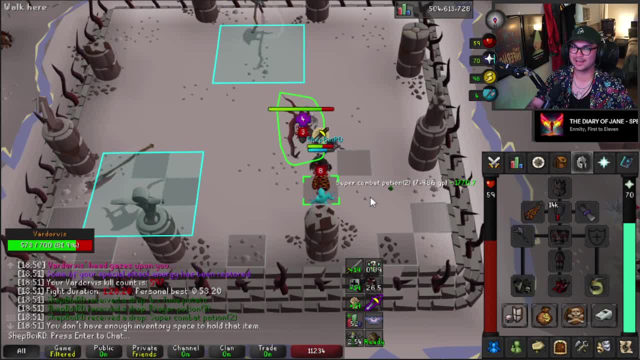 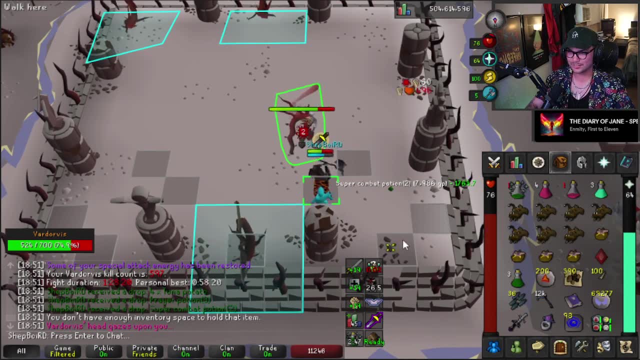 And then, like you can ramp up the difficulty a lot where you actually have to like- I don't know- Be like fuck, Be super, like cognizant of everybody's, like specials, and have to like our stratagems. 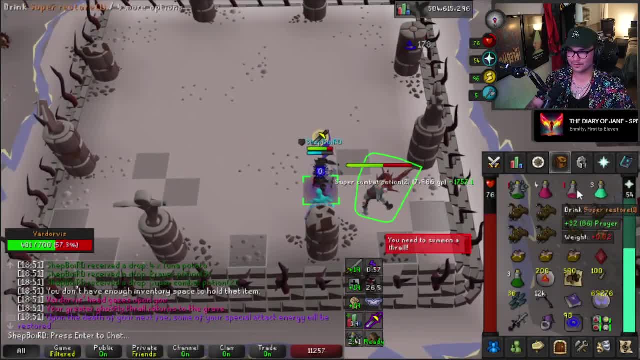 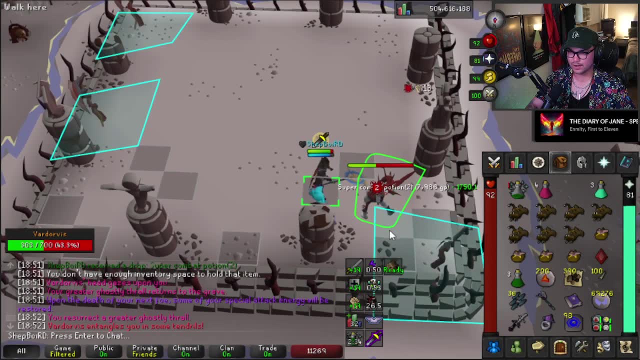 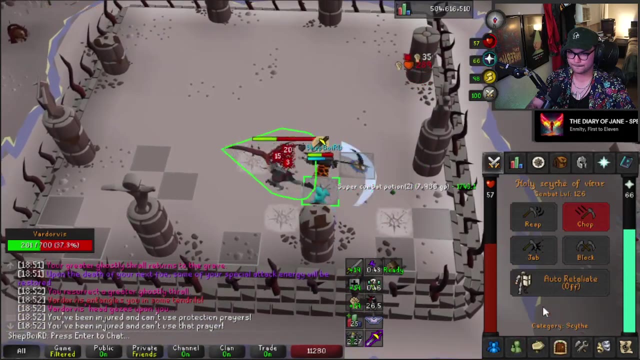 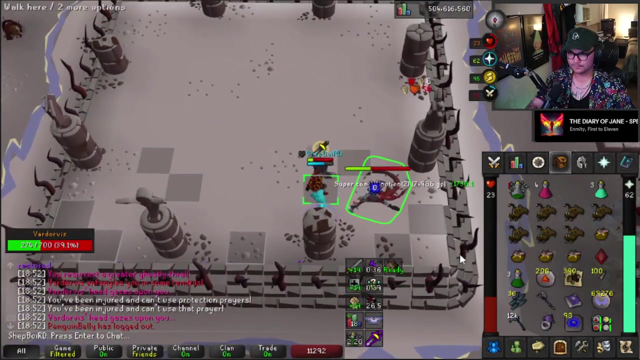 Um, I don't know, It's a really cool game. It's a really fucking cool game, Dude. I'm actually kind of fucking right now, Kind of fucking right now. I don't know. That was some movement there, That was some movement. 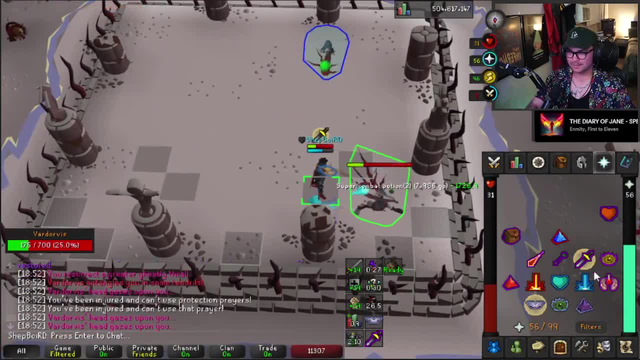 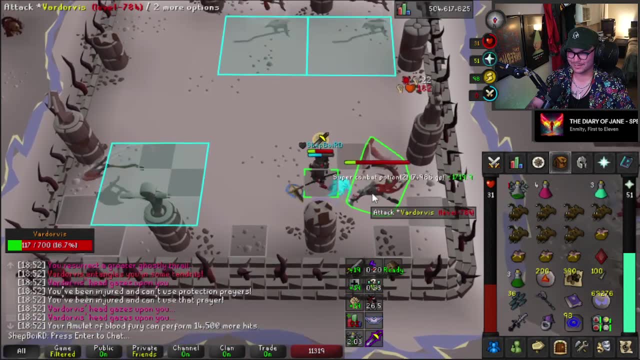 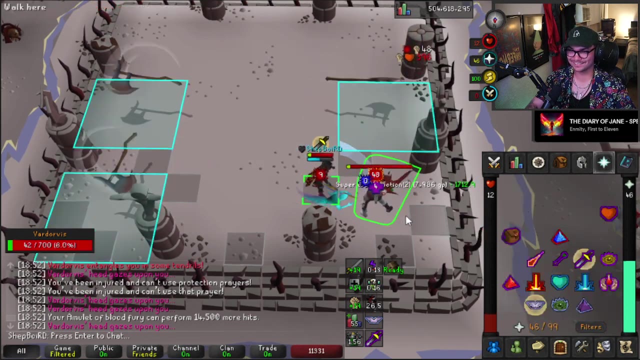 Hopefully blood fury. This might be a hit up churchy for a heal angle after this one. This might be a hit up churchy's ult angle on this one, Because I'm not eating, I'm not fucking eating. That's DPS loss and we hate DPS loss. 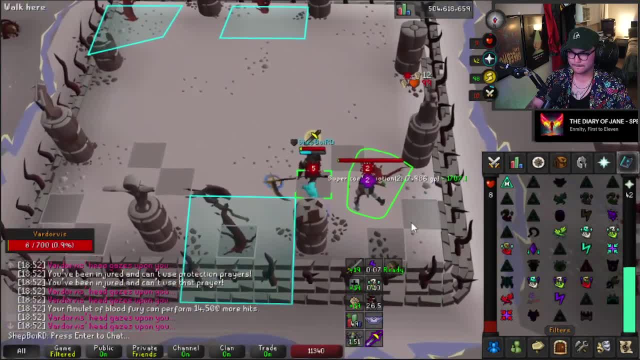 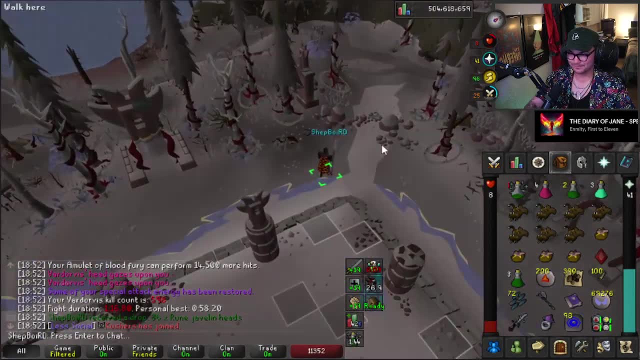 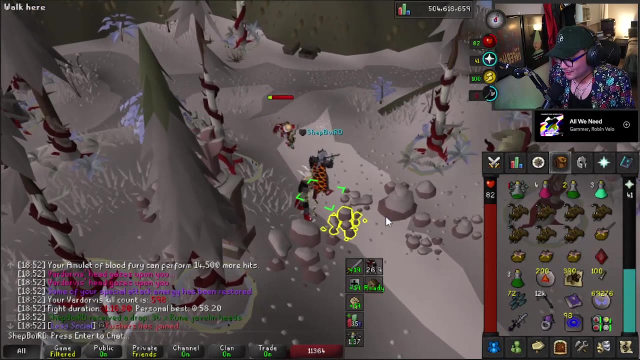 Yeah, Yeah. that next hit was going to kill me for sure, Without a doubt. Senor Churchington, If you could, sir God, you're my hero, You're my hero, Just fucking kiss me on the lips. 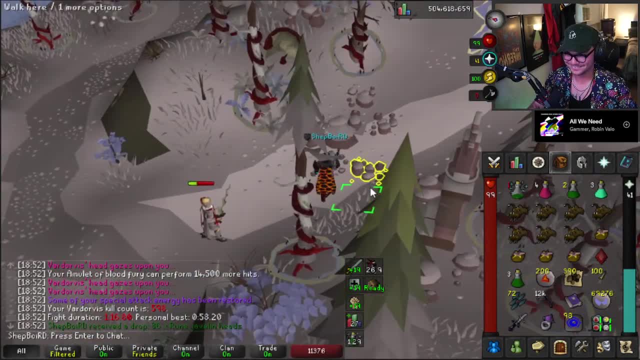 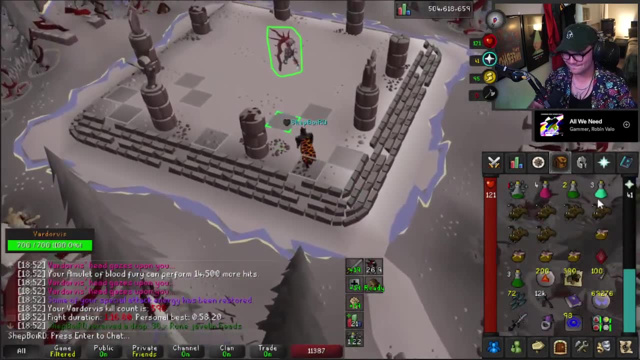 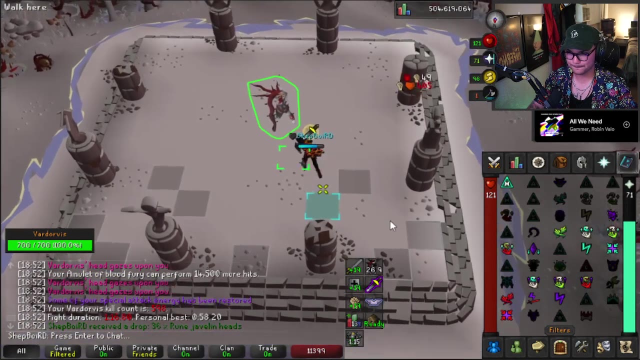 Just kiss me on the mouth, dude, Holy dude, I'm ready. I'm ready. I feel rejuvenated and ready to fuck. You know what I mean. Would you like to know more TY for the HP And the spec.